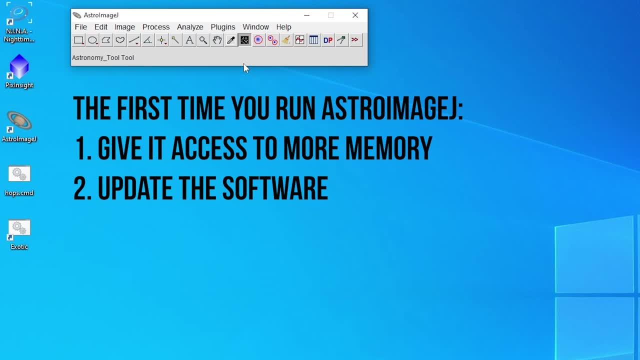 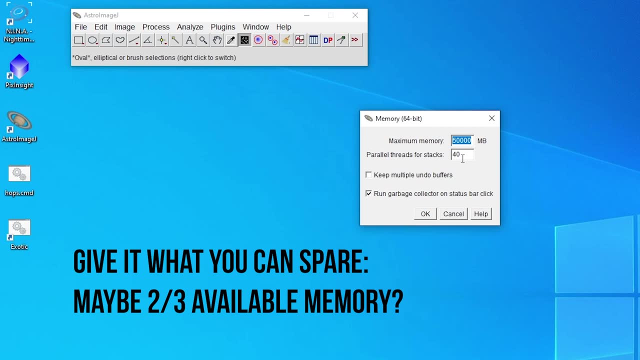 available to Java for this application, and the second thing will be to update it. So let me show you how that works. So obviously you need to configure this based on your own machine, but give it as much memory as you can. Maybe assign about two-thirds of your available memory to this. 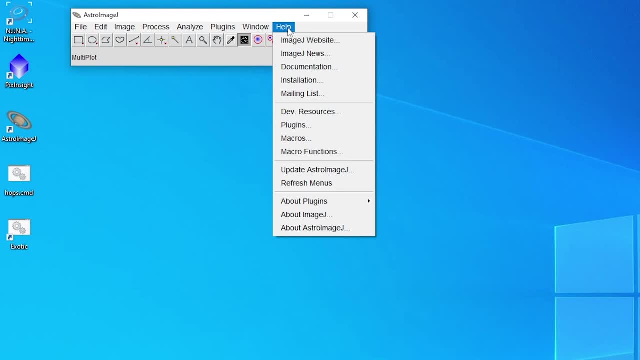 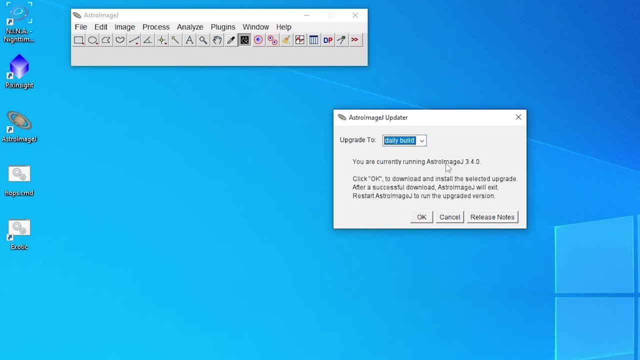 From an update perspective. you can just go in and check the updates. You're probably going to download 3.2, and you'll need to update it to 3.4.. That's a very easy process. Now, before we go any further, in Astro Image J, I think. 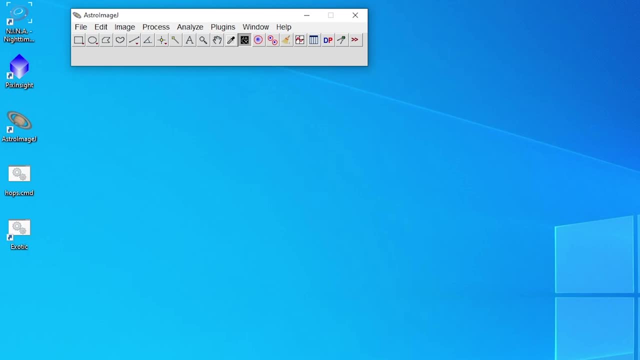 you need to understand the data you're looking at, Because the Neenah plugin took a lot of the initial workload away from us. you probably didn't have to go search to find a transit, which means you didn't have access to some of the data you're going to need at this point. So I'm going to show you one of 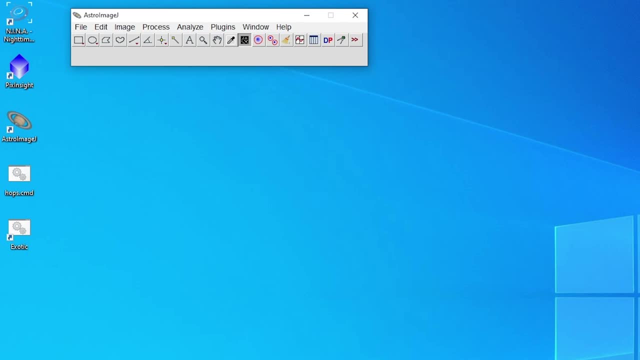 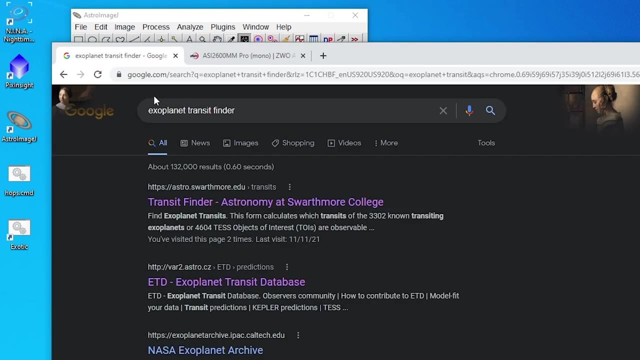 the online tools you can use to find transits or to go back and find your previous transit view imaged so you can get the data points you need to complete the processing. One of my personal favorites to use is the Transit Finder from Swarthmore College. 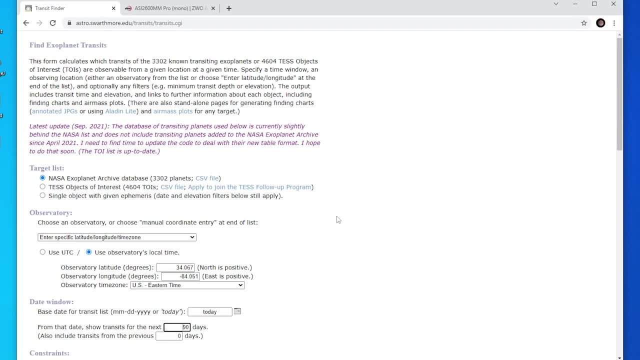 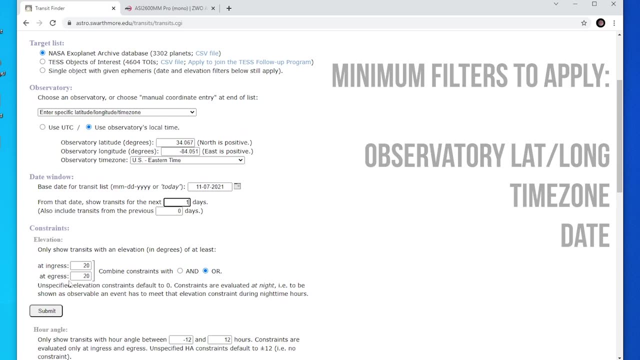 Now it's pretty simple to go through the filter. Make sure you at least fill out the minimum requirements- the observatory time zone, the date, the date window- Then you can go ahead and submit it. You may also want to include things like minimum magnitude of the star and even the depth. 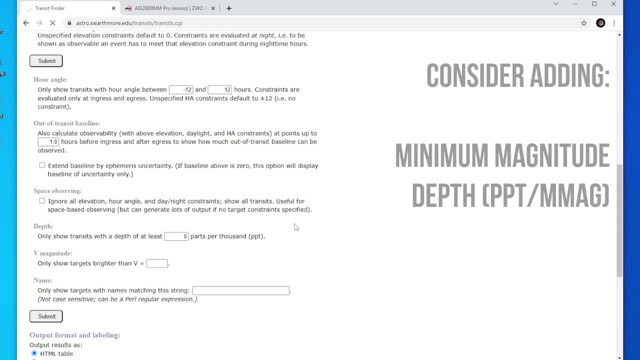 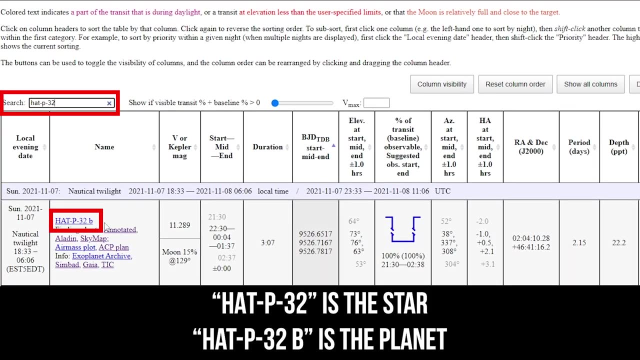 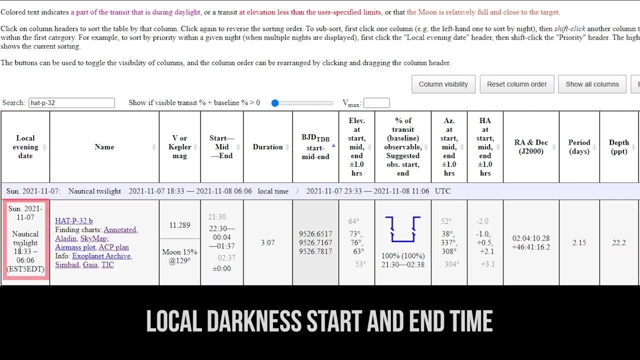 And the depth will either be in parts per thousand or milli mag, It's the same thing. Now I'm specifically searching in such a way here that I can find data about the transit that I captured- and that was for HAT P32B- around star HAT P32.. The first column is talking about my twilight hours, my dark hours. 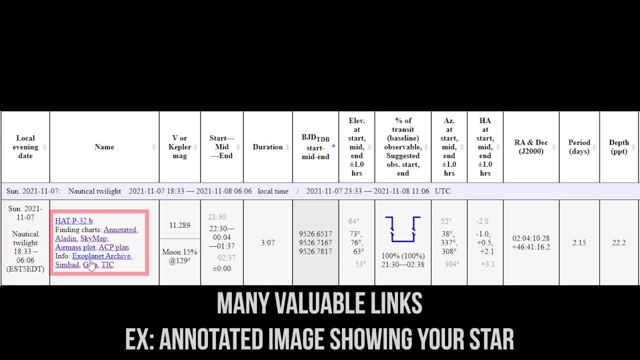 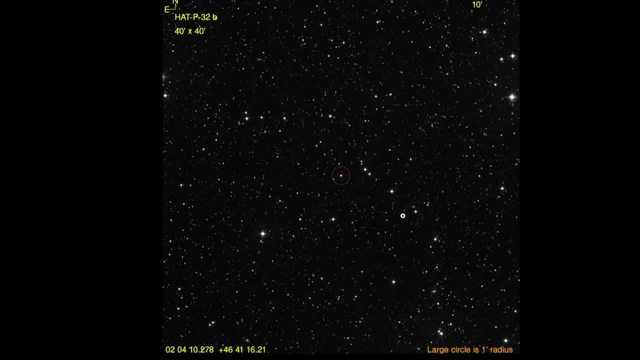 Am I going to be able to image this based on my own personal availability? The second column has numerous links available and we'll probably see these throughout the processing video. One example of that is an annotated image that'll show me where my star lies in a star field, which can be very helpful. 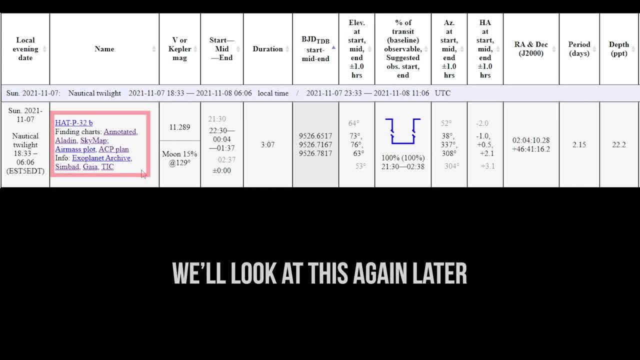 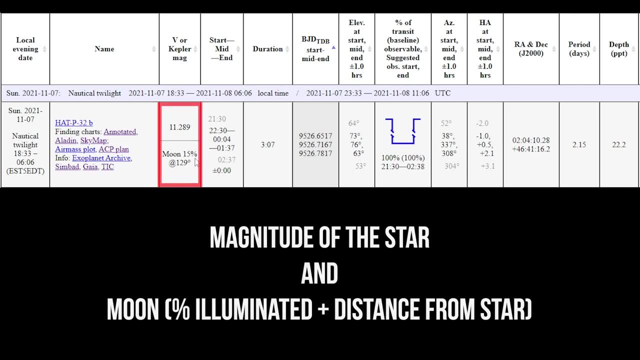 later on. We'll definitely be back here later. The next column covers both the magnitude of the star in question as well as the moon's position and potential effect on our transit. This next column here is giving us the timeframe of the transit itself, so we can see when. 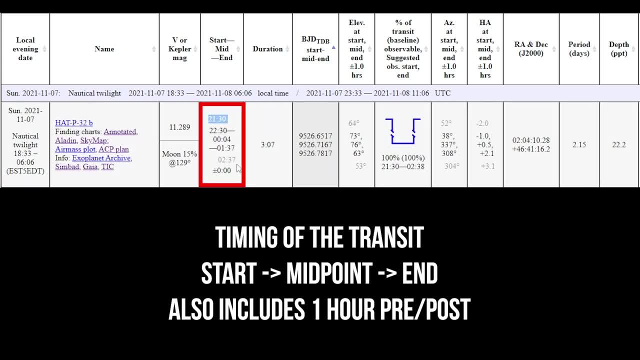 the transit starts when it ends, as well as the hour prior and the hour after. Remember, we need to capture a baseline during the transit to understand what the star normally looks like before the transit occurs. This next column is about the duration of the transit. 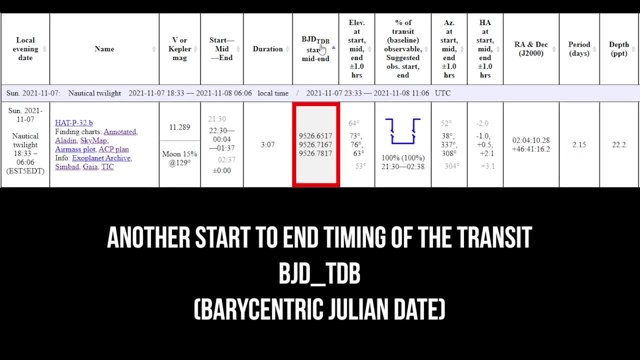 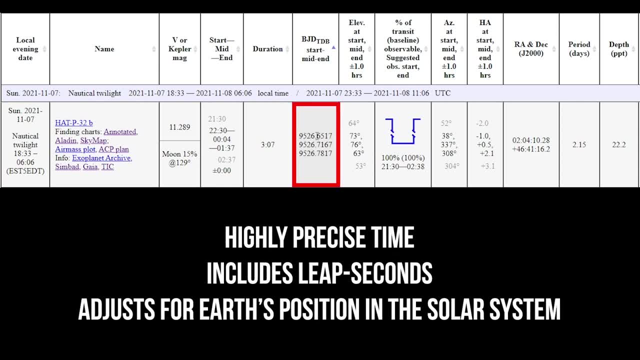 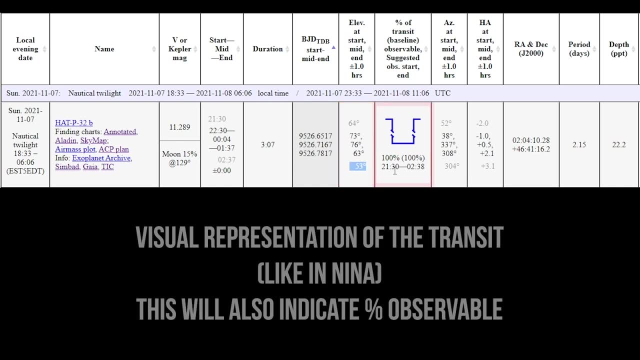 So it takes about three hours and seven minutes. The next column is time in BJDTDB. This particular time reference uses leap seconds within its calculation, as well as the position of the Earth within the solar system. Here we can see the altitude at each point on the transit timeline. Here we can see a visual representation of the transit like we saw. 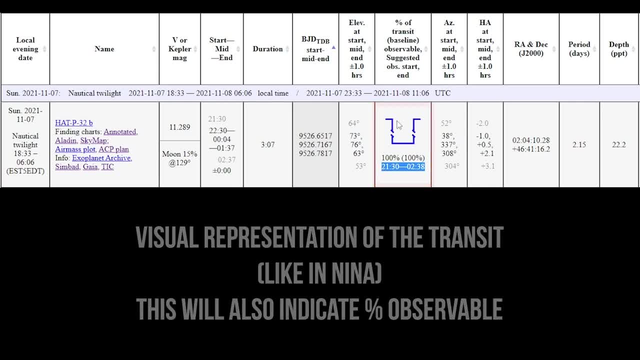 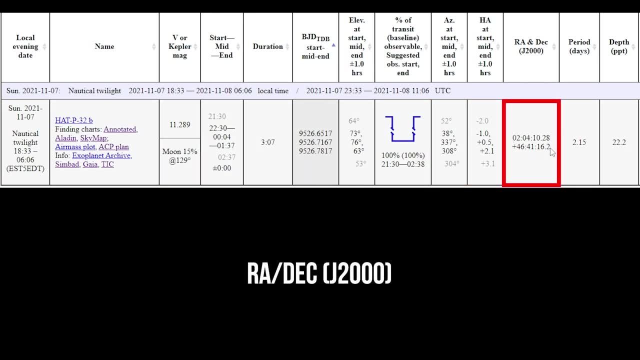 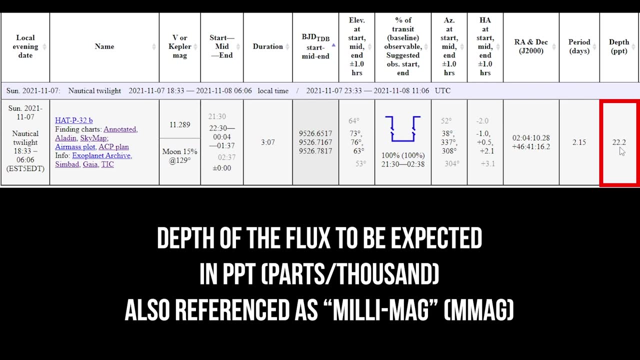 in the NENA plugin. The next couple columns talk about the position in the sky in relation to azimuth and hour angle, And then after that we see the very familiar coordinate system of RA and DEC. Finally, we can see the period in days. And then the last piece of importance here is the depth in PPT. 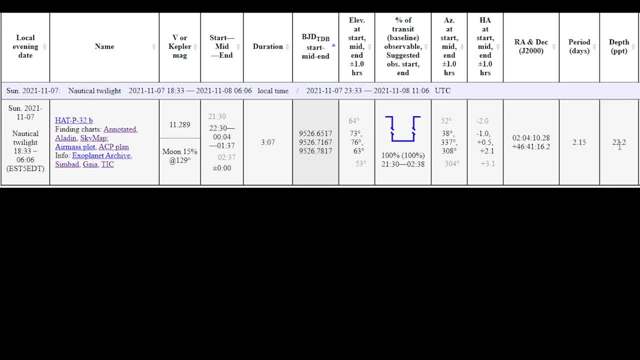 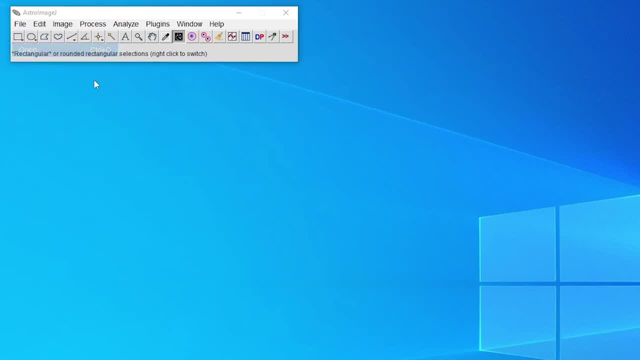 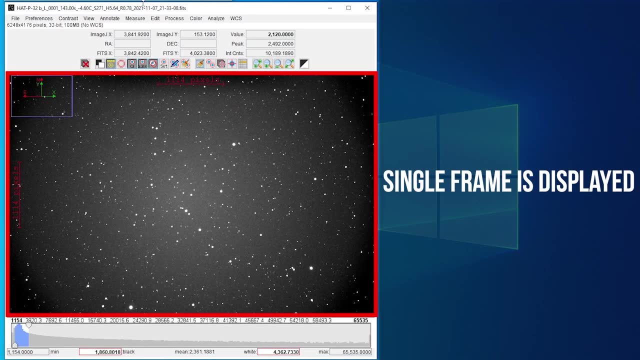 which is parts per thousand. And right now we're going to go back into ImageJ and open a single file using File Open. Now notice: here we have a single frame displayed and we can see that on the screen in the large area. We also have access to a histogram. that's. 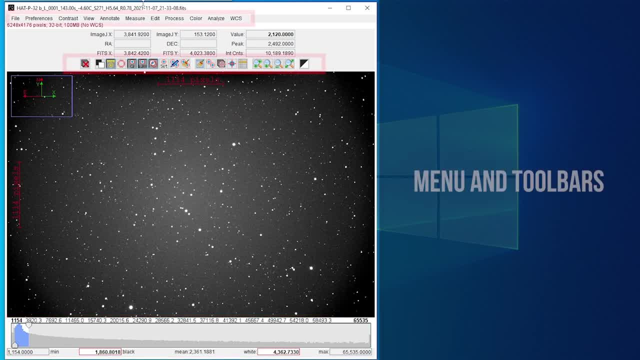 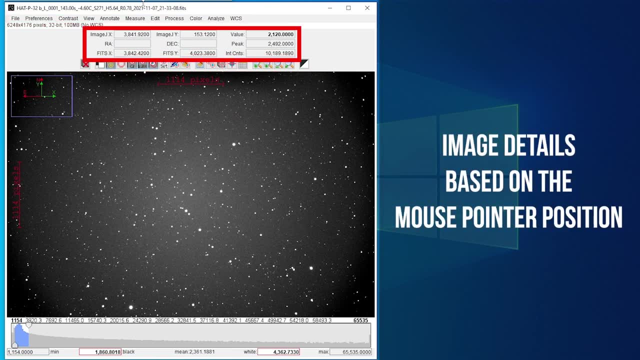 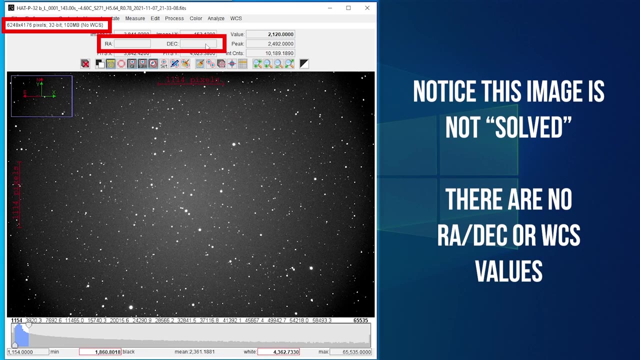 already pre-stretched for us. We have menus and toolbars that are available, much of which we will be using throughout this video, And we even have some image details based on where our mouse pointer is on the image in the screen. Notice we don't have RA and DEC coordinates and it also says up top: no WCS. 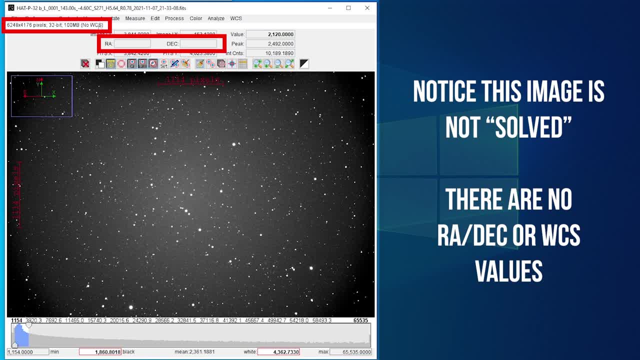 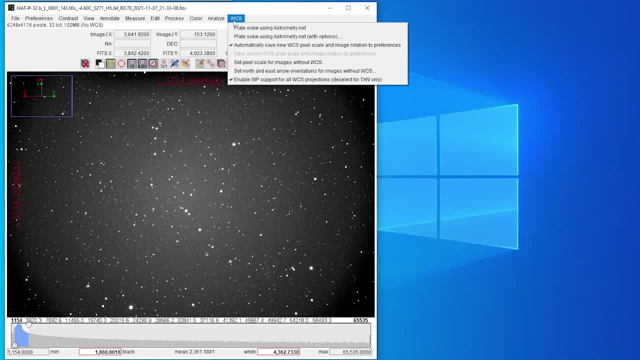 This is not solved, And in order to do this properly, we need to solve these images. You can actually do some plate solving within Astro ImageDay itself. It does have a hook to the API with astrometrynet, but I can't even imagine trying to run this many images through astrometrynet's API, So instead, what we're going to do is we're going to use a local. 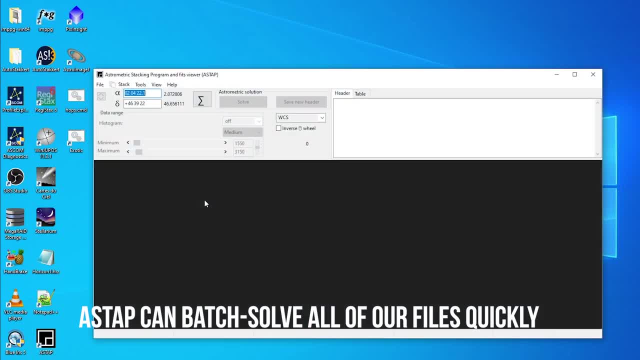 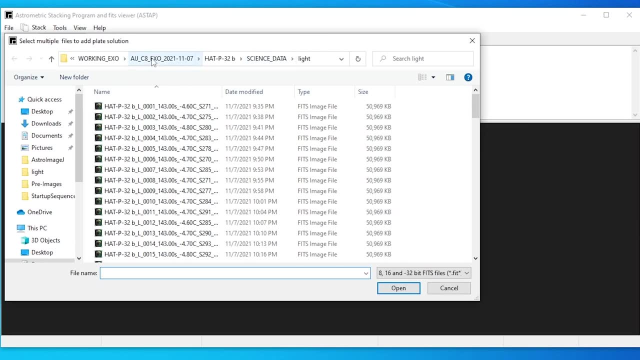 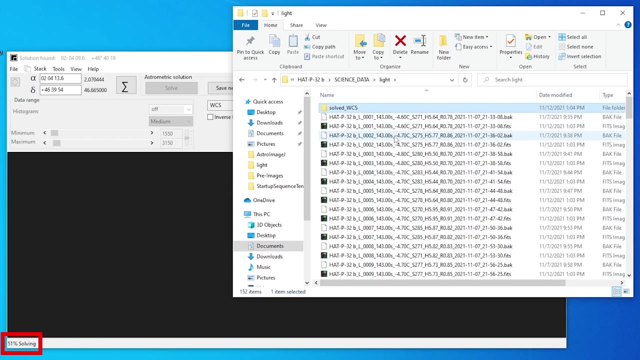 installation of ASDAP. So we're going to use ASDAP to batch solve. Notice, it's already set to WCS. That's the default. We're going to go up to Tools and we're going to batch solve these files. We're going to go into our light frames, We're going to select all of our light frames and then we're going to go ahead and it'll start up. So, as ASDAP goes through the process, what it's actually going to do here. 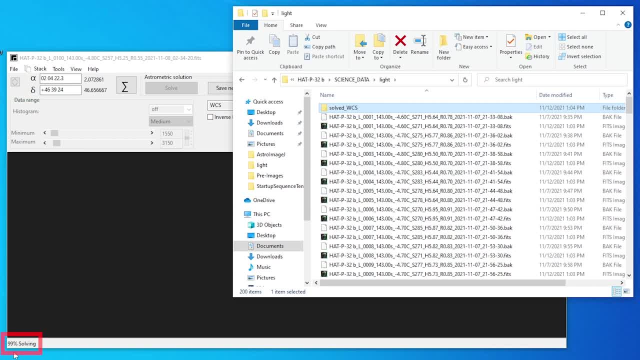 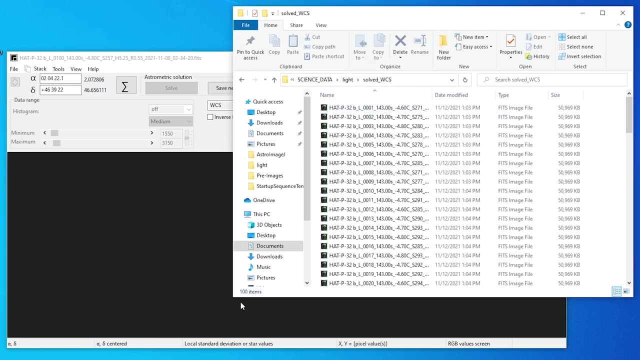 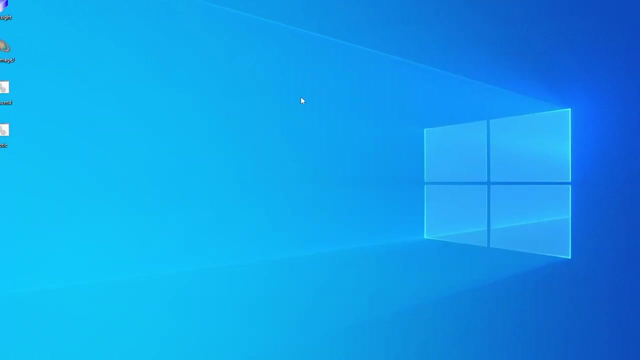 is. it's going to clone every file as it solves it, So it'll save the original file as a bak file and it'll create a new fits file with the solved data in the header. When it's done, we're going to grab all our new fits files and I'm going to drop them into a solved WCS folder, just so they're all together in one place And I can leave all my backup files where they pre-existed. Once that's done, we can close ASDAP and go back in to Astro ImageJ. Now, this time we're going to open up what they call a file sequence, So we're going to go to File Import: Image Sequence. 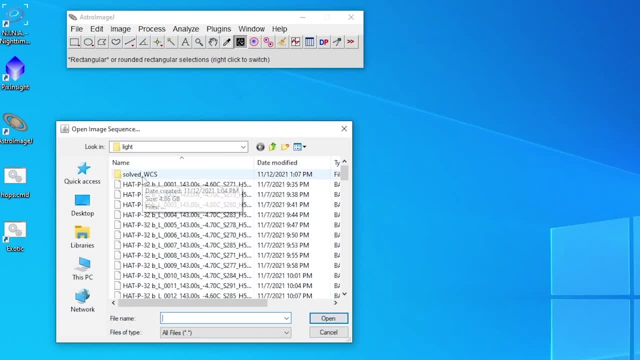 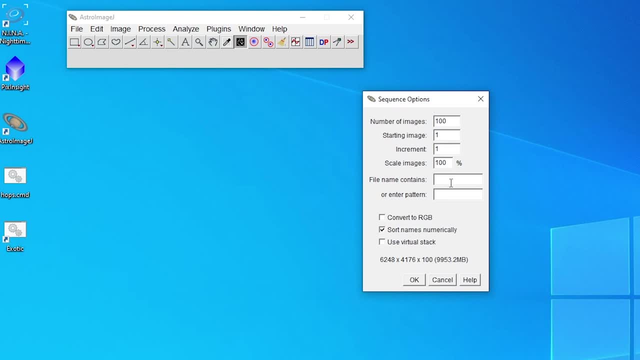 Make sure you go into your solved files and you only need to click on one of these. It's going to identify all the other related images in the folder. You can see it found 100 of them. I recommend only having the working light files in a single folder. It'll be easier to work with here. Otherwise, you may have to use some of these filters to specifically identify your light files. One other recommendation I found online is that you should be using virtual stacks. Now, if you have a lot of memory in your system, you may not need to use virtual stacks, But I did have a 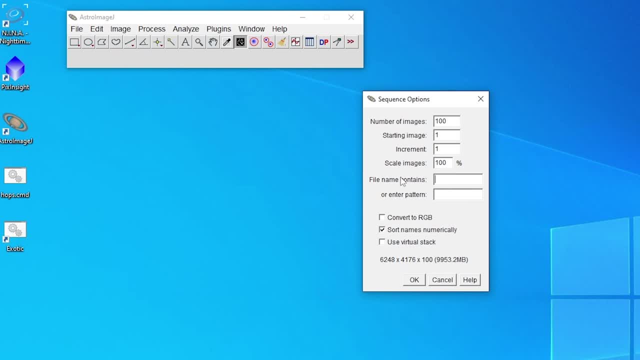 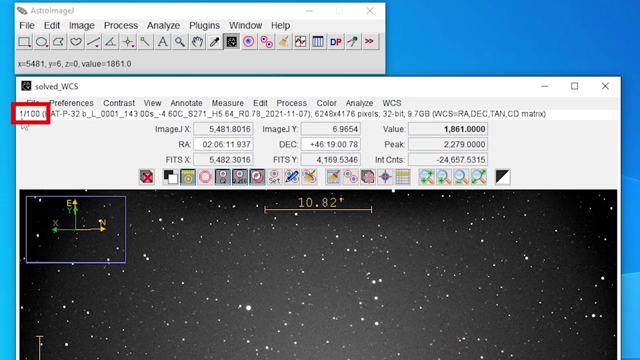 some challenges when not using virtual stacks. There were some performance problems occasionally, So my recommendation is check the box for use virtual stack. Now it's going to go ahead and open up that entire sequence of the 100 images that I found there. Notice we are at one of 100. Now. these are called slices within the tool, So I'm on slice one. you can see my file name is here. I have some pixel information about the size of the image And you can see my WCS and RA and DEC coordinates are in this image. 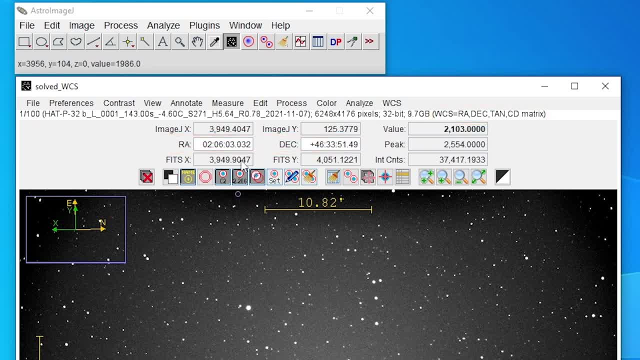 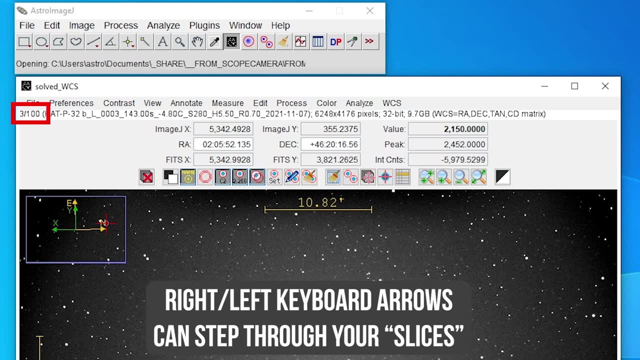 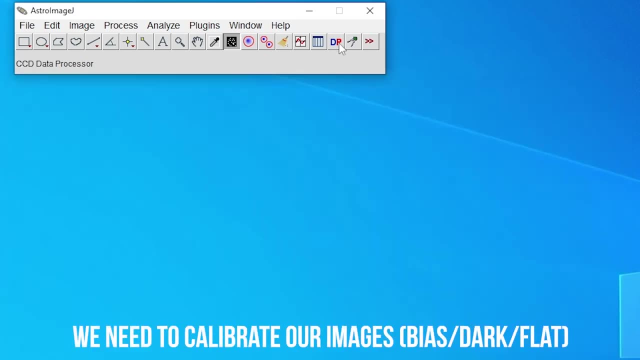 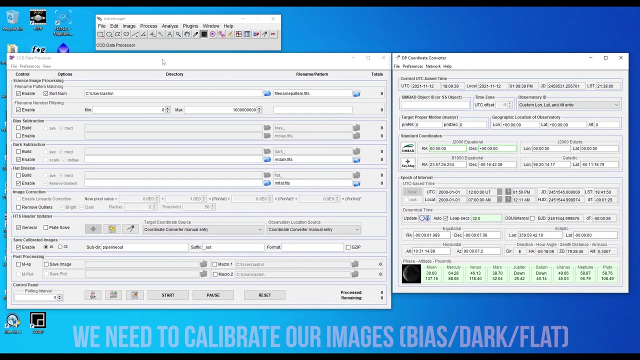 If I use my right and left keyboard arrows, I can go through the slices. so I can start to go through 1234 and so forth. There is also a scroll bar below the image that you can use as well. So within Astro image j, we can calibrate our files, And to do that we're going to go up top here and click DP. Now, like most things in AIJ, this can get a little bit overwhelming. The first top line here is about your science files. Those are your light frames. So I'm going to go find my light frames here And I'm going to go to the 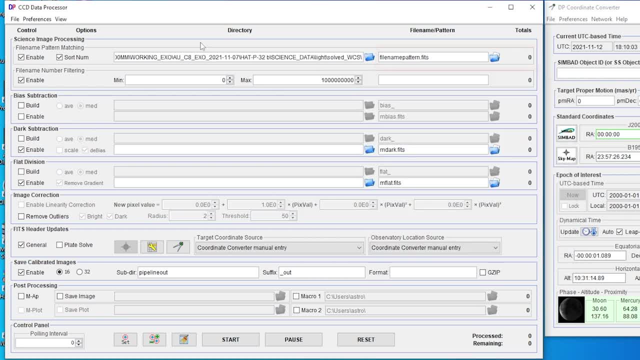 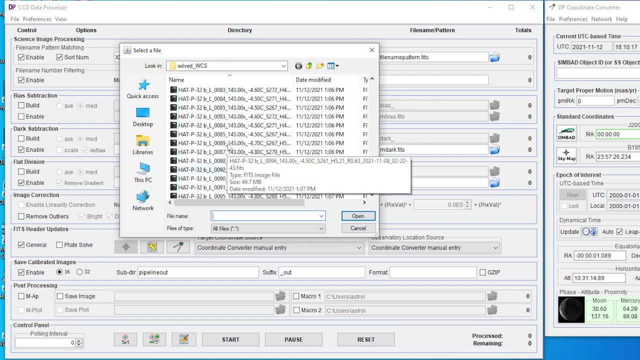 and identify the folder. this particular pattern doesn't match my files, so notice it says zero files off to the right. if i know there's a specific pattern within my file names, i can type it here now. it's critical to understand that this is case sensitive, using lowercase. 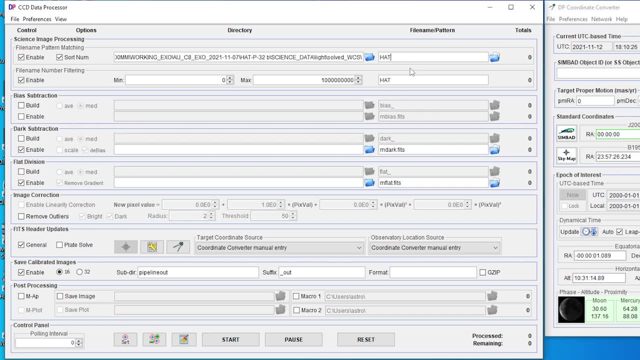 hat didn't work. even capital hat doesn't work because it's not a full match. i actually need to put an asterisk wild card there so i can use capital hat, asterisk, or i like to put asterisks on both sides, it'll always match if it's anywhere within the file name. notice now that i have a. 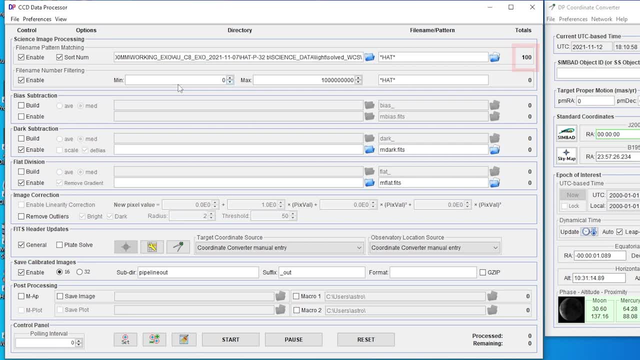 match, it found 100 science files or light frames. now we can go on to bias subtraction. there's two options here: build and enable. i could just click enable here and then tell it what the file name and location was. notice here: it defaulted to mbiasfits, which doesn't exist, so instead we 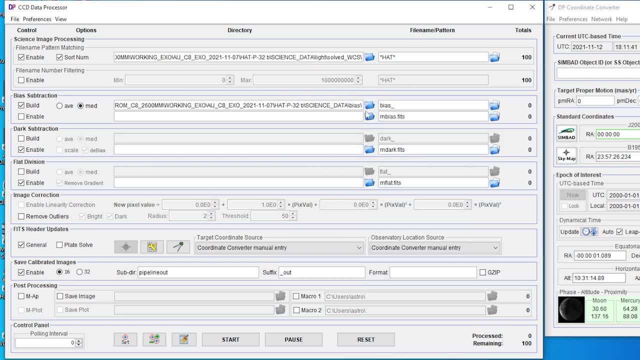 need to build our master bias, so i'll click build. i'm going to select the directory of my bias files and i'm going to give it a file pattern that works. in my case, star by a star notice, it found five files. i also want to enable this because i don't just want to build my master bias, but i want. 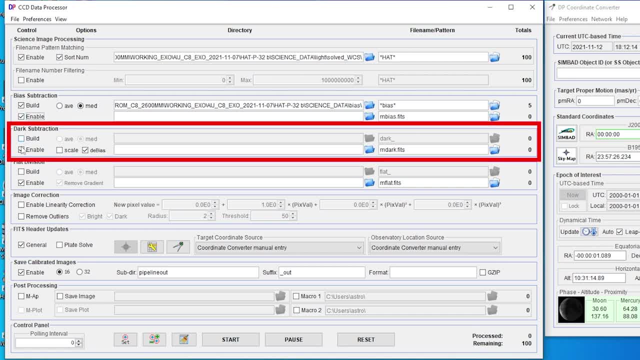 to process it against my light frames. now it's the same thing here for my darks. i could just enable it and select my master dark, but since i don't have one yet, i'm going to have it created as well. i'll click build, i'll give it the directory and i'll also give it the file. 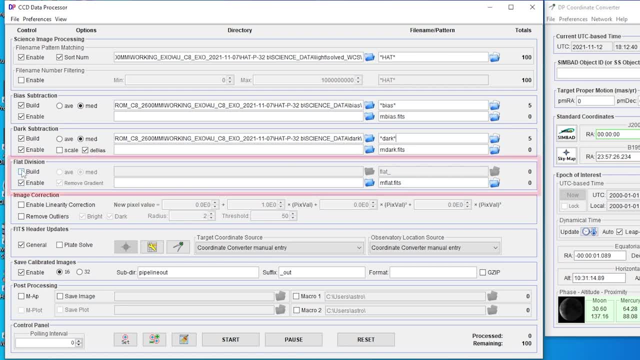 pattern it should use, in this case star, dark star. finally, we'll move on to flats. same situation here. once again, i'm going to build and enable, i'm going to locate my flat files. now notice that star, flat star doesn't work because if i look at my files, it actually has a capital f in. 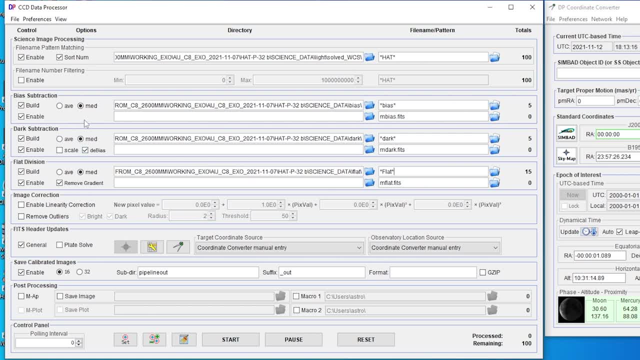 the word flat and this is case sensitive. now, by default, where do these master files get created? they get created in this science folder, which is your light frames folder. if i don't want it there, i can alter those paths. i can look at solve wcs, go up one level and then go up a second level and 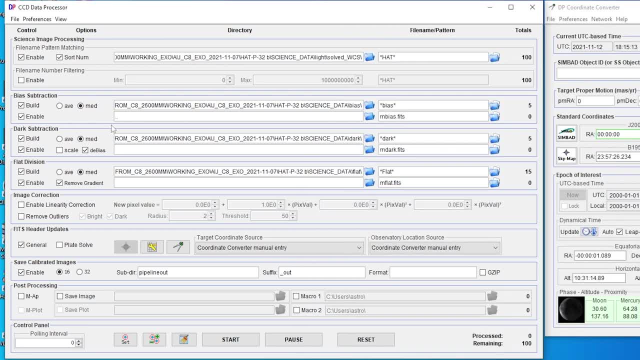 say: this is my science data folder. this is where i want my masters to be. if that were the case, i could just like a normal file system, tell it to traverse directories and, in this case, going up two directories is dot, dot slash, dot dot slash. it doesn't matter to astro image j, where it creates the files, because it's creating the. 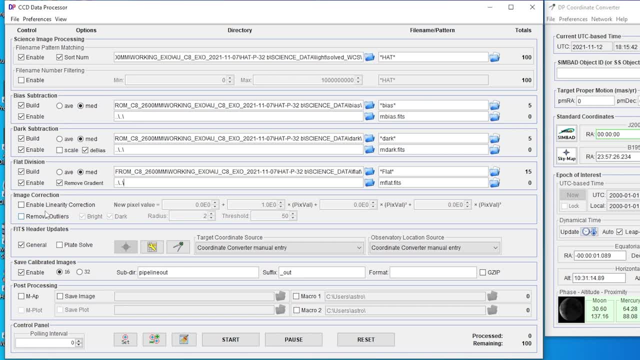 files and using them simultaneously, so it's completely aware of where it stored the files and knows how to retrieve it. okay, next we're going to skip over image correction. i'm not going to do any image correction here, so the next thing we need to go to is the fits header update. 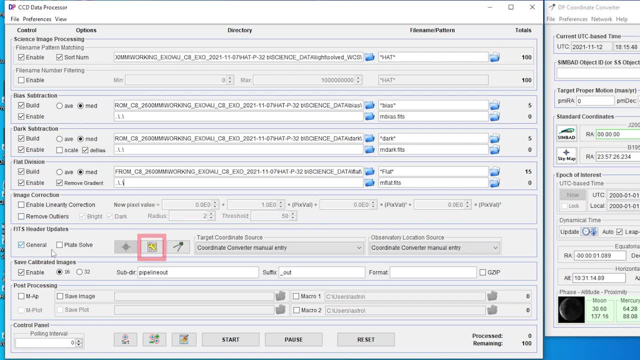 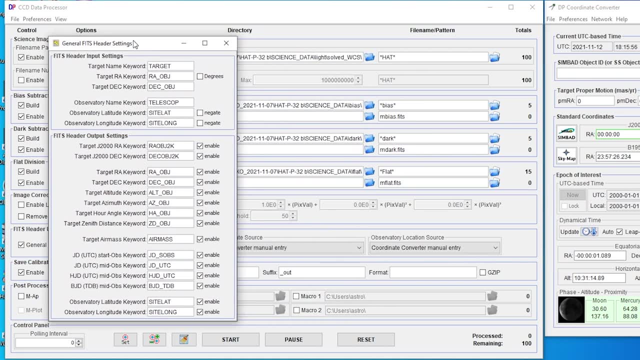 so what you need to do is click here to open up the general fits header information. the section at the top is the fits header input information it needs. so we need to know the fits headers in your files that relate to these data points, because everything here at the bottom is going to be generated, calculated and entered into your fits. 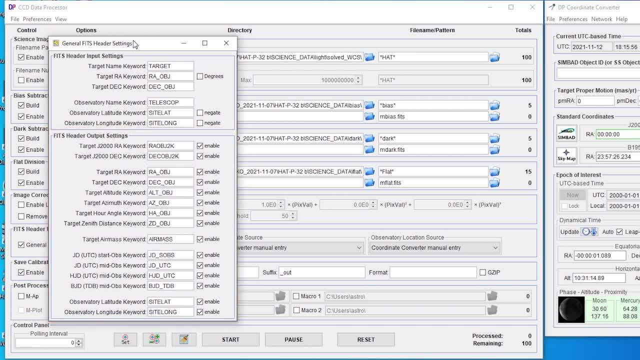 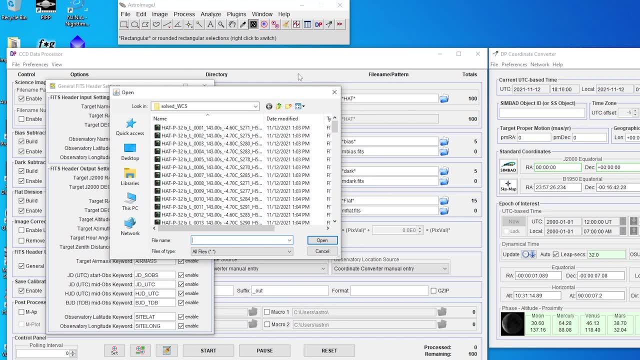 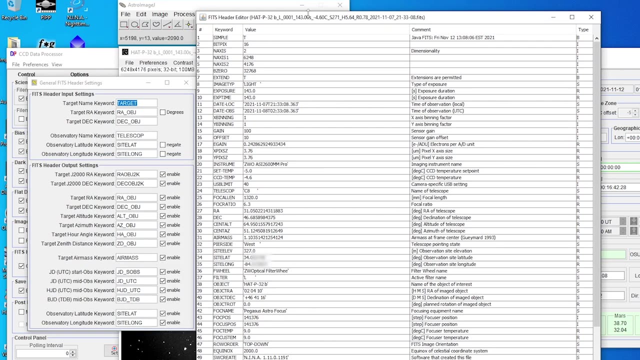 files as a result of the processing done by aij. but it needs the stuff at the top to be in place for that to happen. so the easiest way that i found to do this is in aij to open a single image at this point and then go up here to edit, and then edit fits header and that'll show me the fits header. 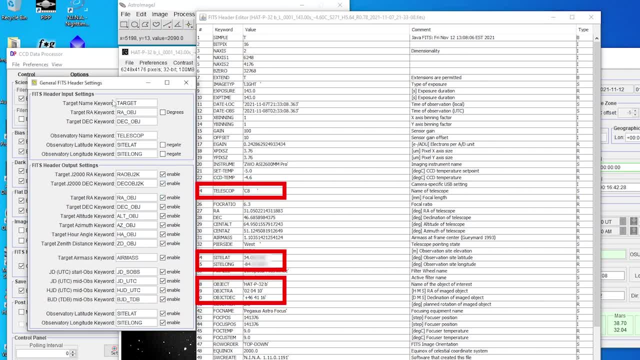 on that file. now i can use the data there to see how i need to alter the form on the left. so notice, my target name keyword is actually object in my fits header, so i need to modify that. my target, ra and deck are different as well, so i need to find that in my fits header. 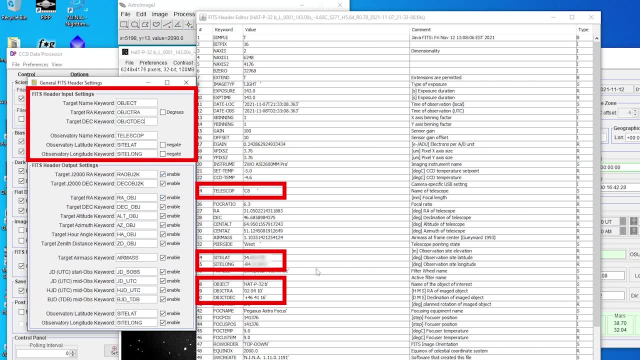 and alter the parameters. so aij knows where to look in the fits header to retrieve that information. you need to make sure that all six pieces of information at the top here are valid and can be found in your fits header. one other point i'll make. at the bottom here we 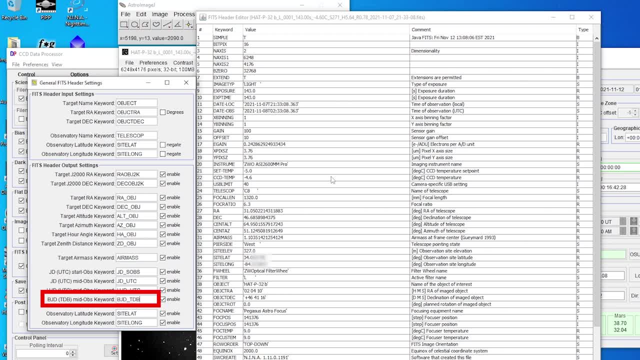 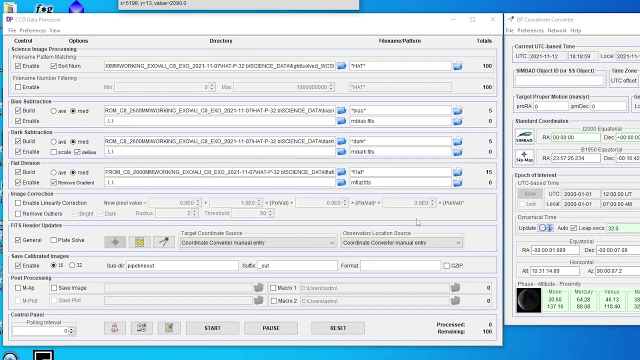 want there to be a field for tdb time, so make sure you have that field as bjd tdb. if it says something else, change it to bjd tdb. okay, so we can close those two fits header windows, as well as the single image we opened, and come back to calibration, the next thing we need to 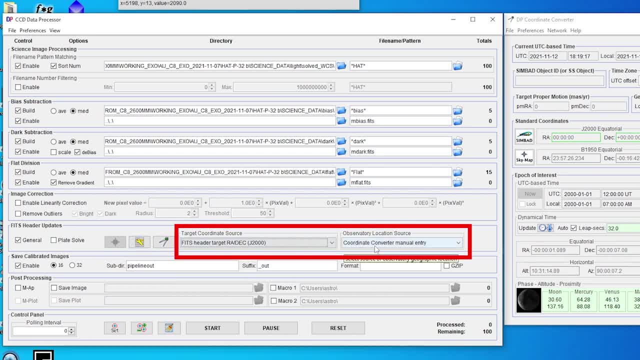 is we need to tell the form where to pull the target coordinates for the source and for our observatory location. one other suggestion here: go off to the right in the conversion tool and go ahead and click update to update the leap second data. i do find this is a little fluky and sometimes 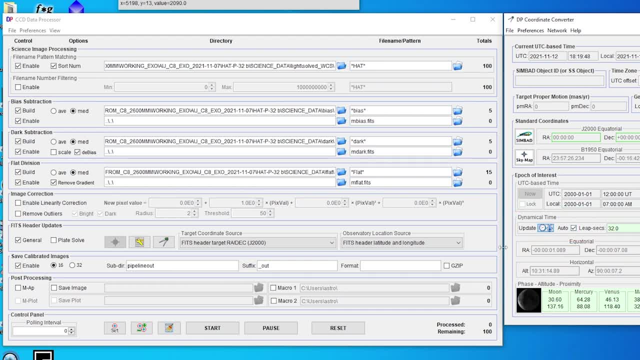 the lookup fails, but it is important with tdb time that we have an accurate number of leap seconds calculated as part of our time frame reference. we can come back over to the main window and i'm going to use 16-bit images because i'm using a 16. 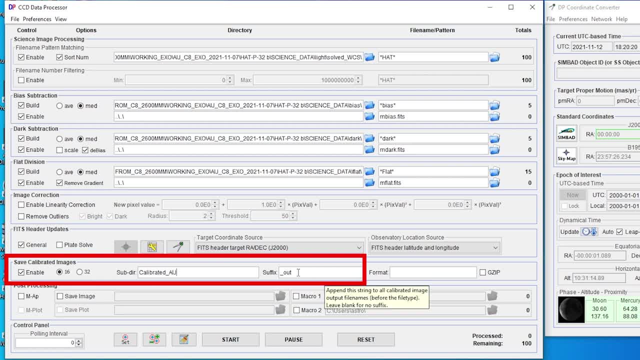 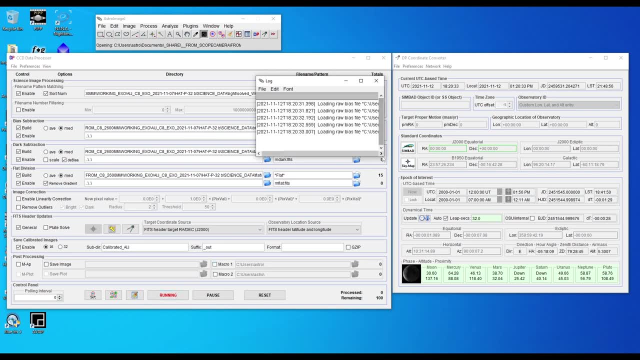 bit camera. i'm going to set the output directory for these files to be calibrated underscore aij and i'm going to leave the suffix of out and i'm going to go ahead and click start. now we're going to get a log file that pops open. that'll allow us to watch the calibration process, and we're 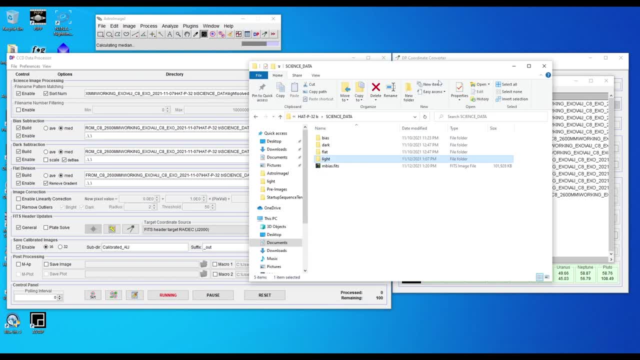 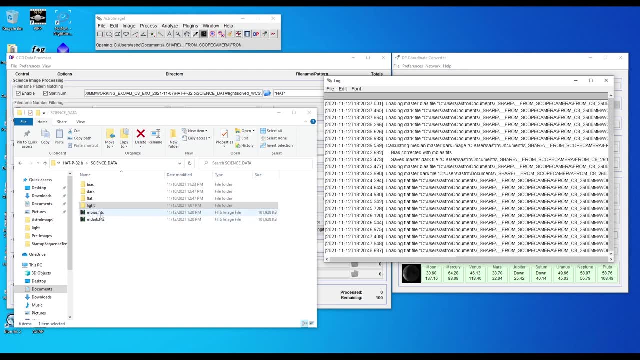 going to start the way we would expect. we're going to go through the bias files and create a master bias. we can see that's dropped in the folder. then we're going to go through the darks and bias in the master dark. then we'll go through our flats and process the flats appropriately of. 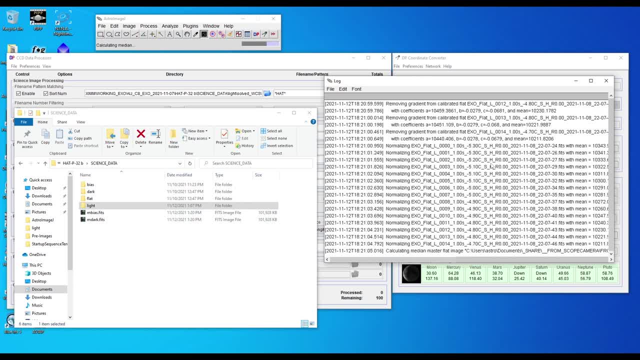 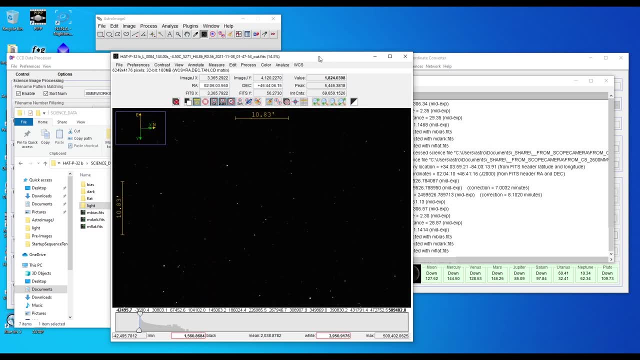 course, using the master bias and darks against the flats until we generate our master flat as well. at this point you'll see an image open on the screen as the system goes through all of your light frames and properly calibrates them against your master files that were just generated. 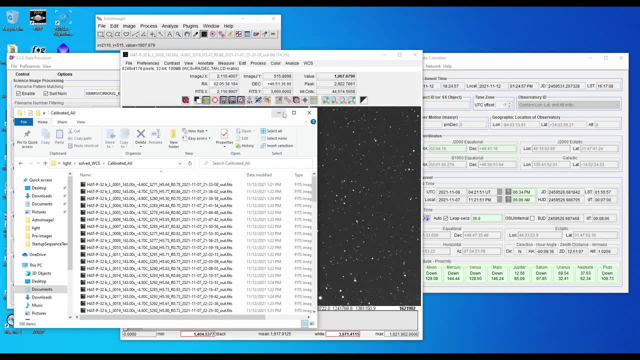 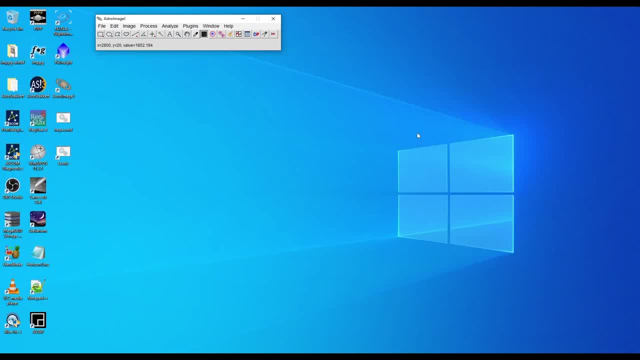 i'm obviously going to speed this up because we don't want to watch this process in its entirety. once it's done, you can just close out of that, leaving the smaller astro image j window open. then we can go and open a new sequence, and this time we're going to open up our calibrated files. 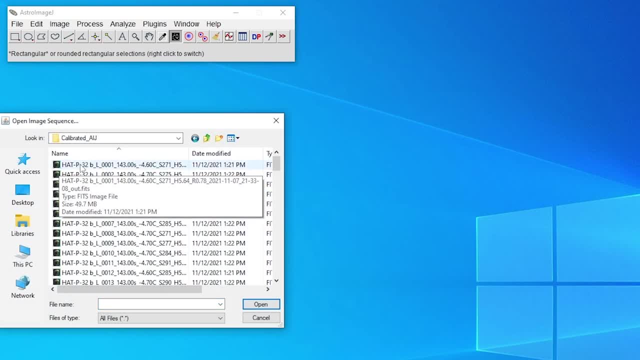 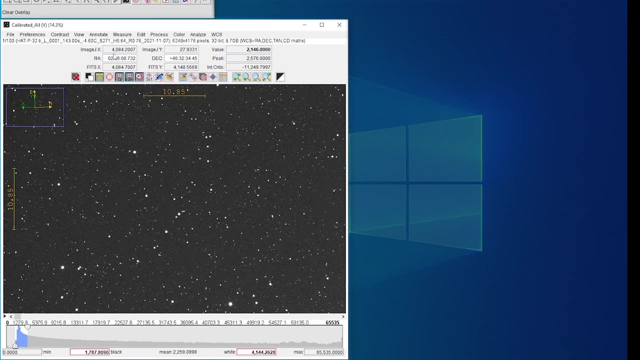 select one of the files in the new calibrated folder and again open it like we did before, making sure use virtual stack is likely checked. it now opens up our calibrated frames. so when we open the new sequence here, let's talk a little bit about the interface, this little circle. 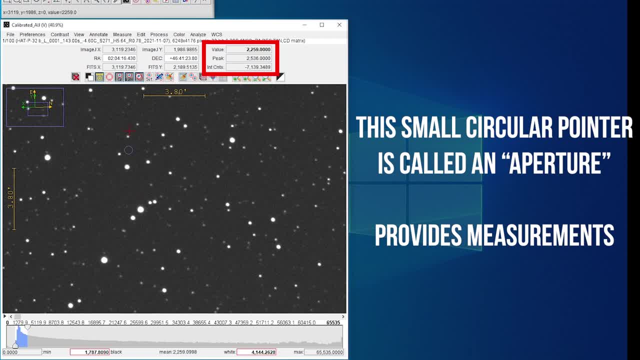 i'm moving around with my mouse is called an aperture and based on what's in that aperture we can see values up top are changing the value of the pixel. i'm centered on the peak value of in the circle as well as the int counts, which are the sum of all the pixels in the circle. 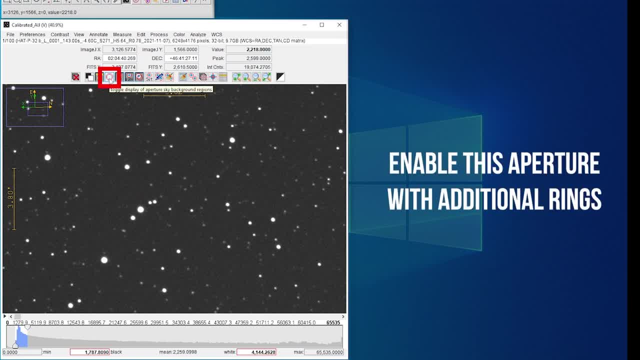 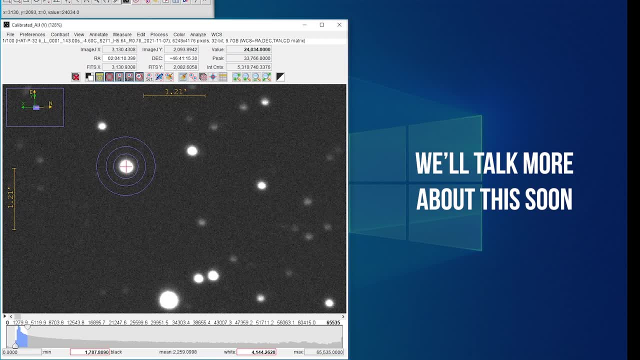 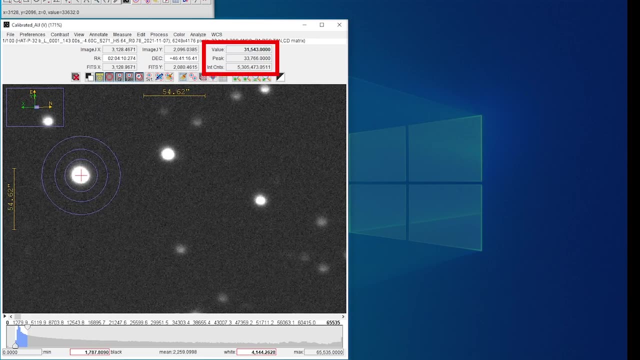 so what we want to do is actually enable a different pointer that has multiple aperture capabilities, and to do that we click up here on the toolbar now. we'll go into the reason for this soon, but there is a reason we need this specific tool. so you notice here again the value peak and 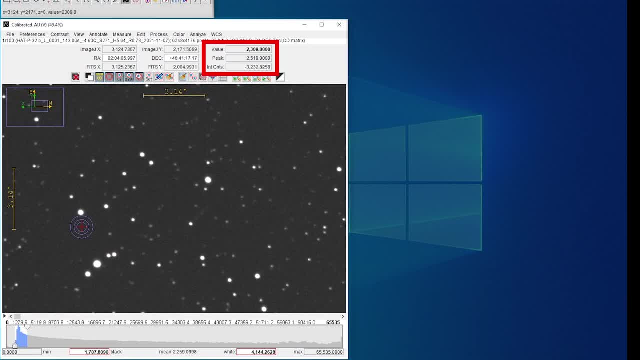 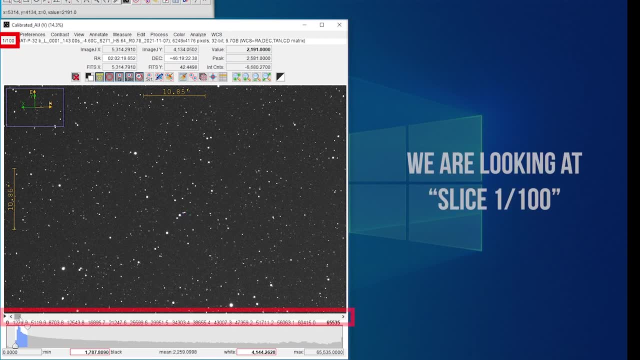 in counts. as i move around and center on a star notice i can scroll in and out pretty easily with and also notice that we are looking at slice 1 of 100. i can use my arrows on the keyboard or we can click around here on the scroll bar. as i click around on the scroll bar, notice that it. 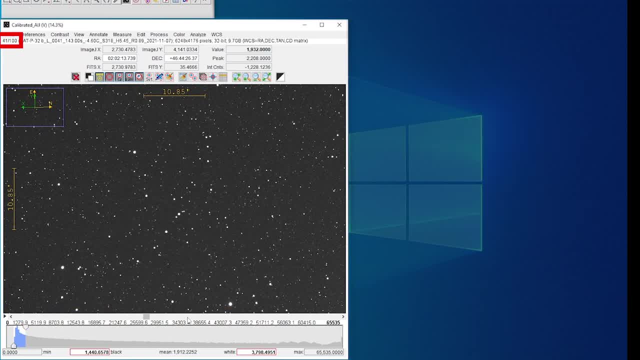 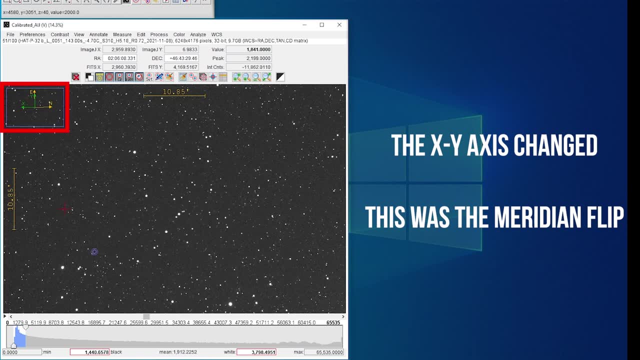 jumps 10 images at a time. when i go between images 41 and 51 notice the image seems to move a little bit. if i look in the upper left hand corner, it tells me the direction of x and y, as well as north and east notice. x and y changes somewhere between 41 and 51.. the application knows how to properly. 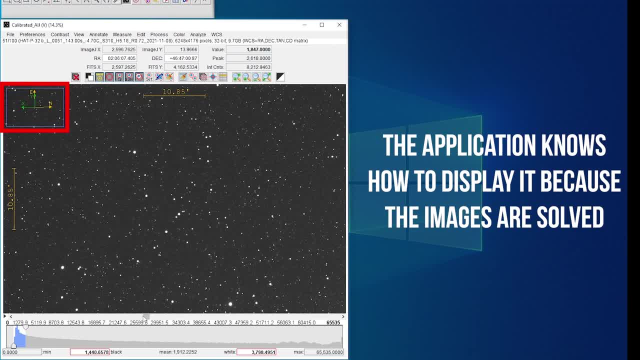 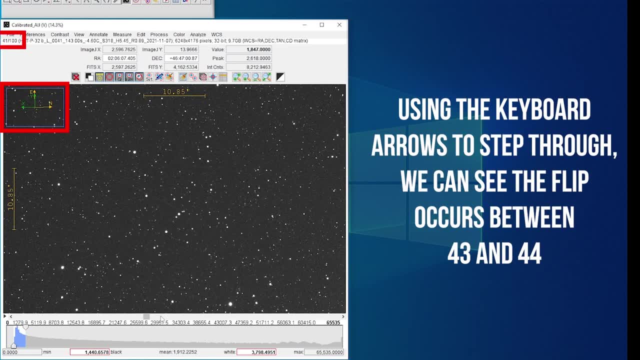 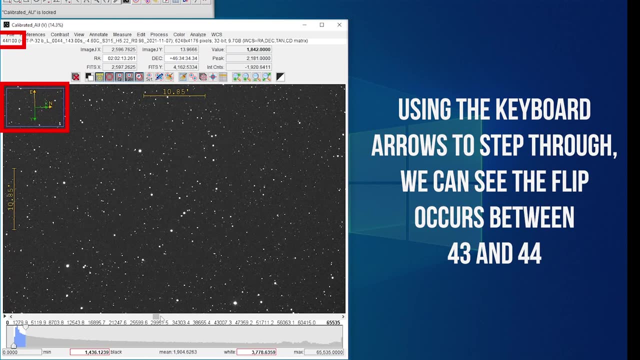 align these and align them because of the solving that we did earlier. now, if i step through these one at a time using my arrow keys, notice that between 43 and 44 is where we get the jump. this was our meridian flip that occurred. now, any movement like this. 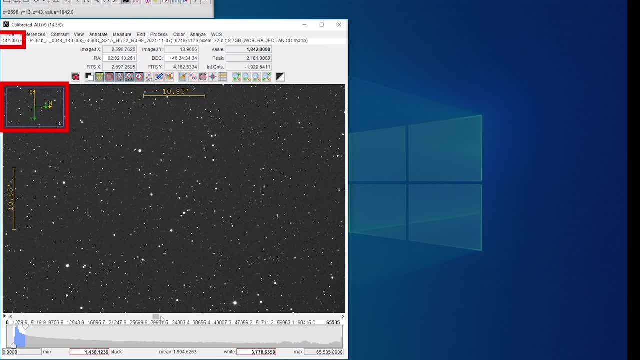 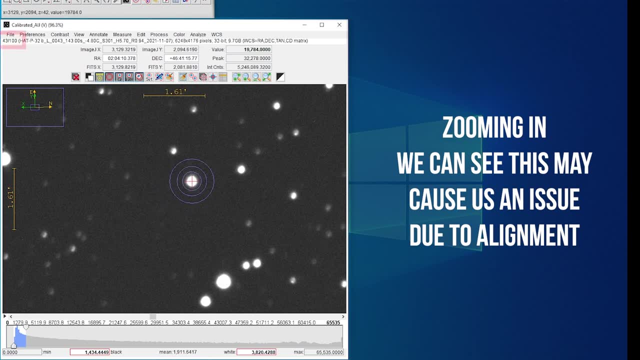 could end up being problematic. so what we're going to do is take a look to see how dramatic this movement is. so i'm just going to zoom in and center on a star, and here i'm on slice 43, and if i move to slice 44 we can see there's quite a big jump. now this can be an issue. 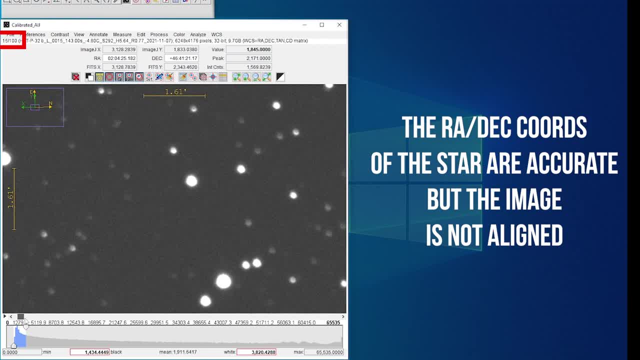 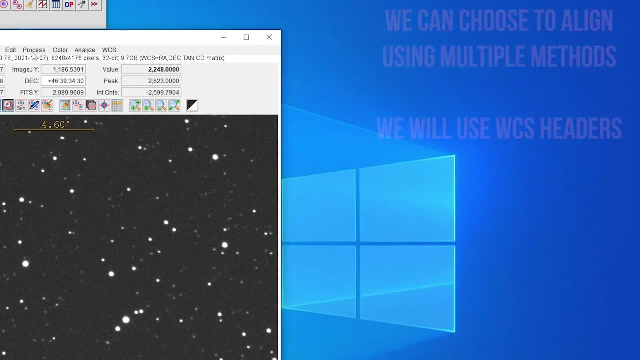 as it relates to alignment of our images when we want to go through the stack and take measurements. so the next thing i'm going to do is alignment and we're going to go up and we're going to go to process and we're going to align stack and we're going to use wcs headers. now, make sure. 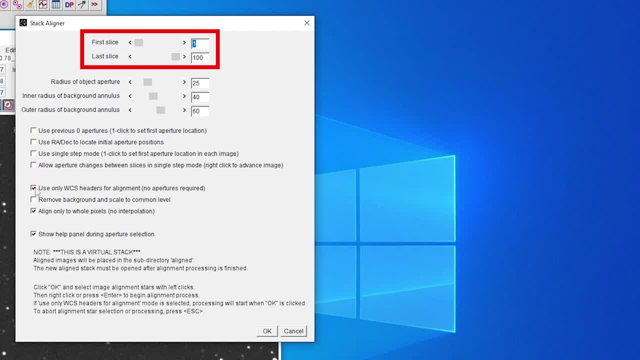 when you go in here that we're going all the way through the slices, make sure it goes from slice 1 to your highest numbered slice, in my case 100, and i'm going to use wcs headers only. i'll go ahead and click ok and we'll see the process moves forward. we can watch. 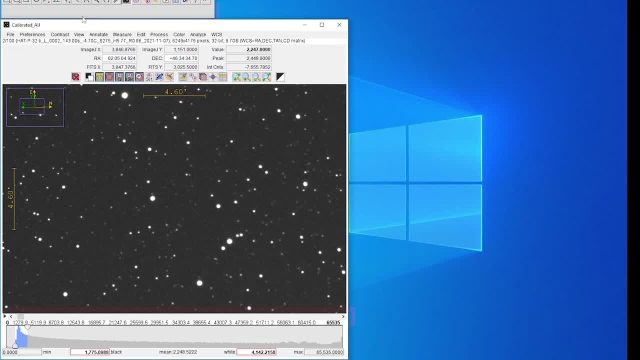 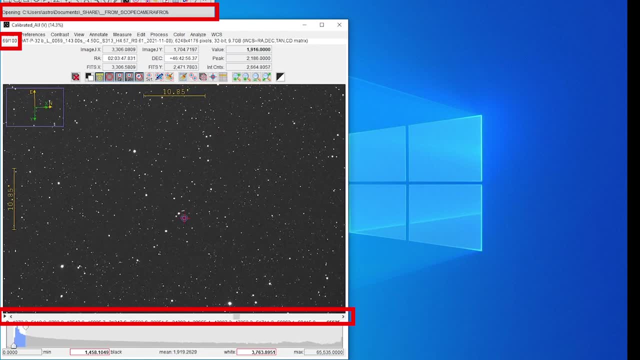 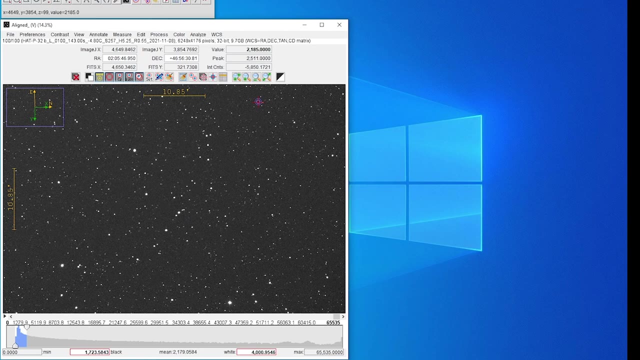 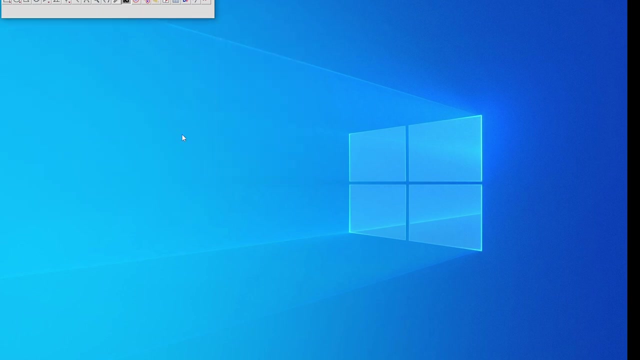 all of the images be opened one at a time, and we can see the slices progressing through from 1 to 100.. when it's done, it'll tell you it's done. we'll close this image sequence and we'll do file open image sequence and we'll open the newly aligned files. so now let's just do a quick validation. 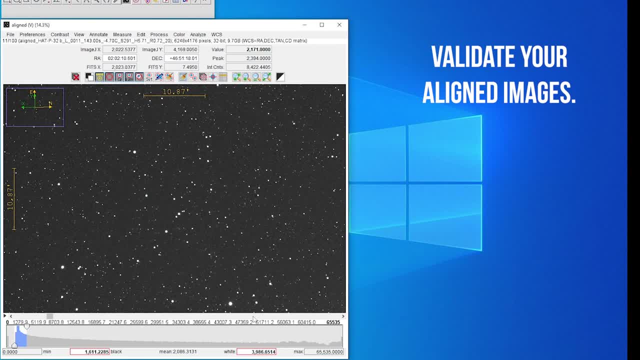 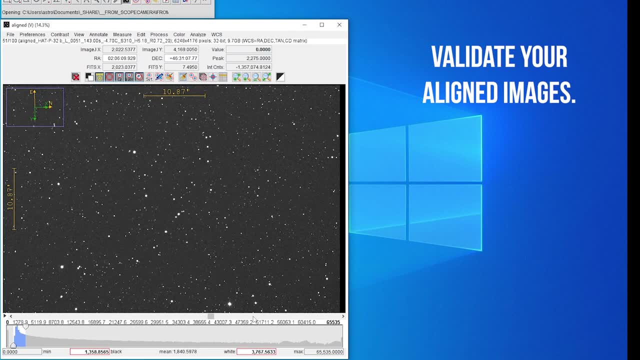 i have my aligned files open. i'll just start going through 10 at a time by clicking on the scroll bar and we can see we're skipping through 10 at a time. notice: as i click through, i'm not seeing the same movement i saw previously. 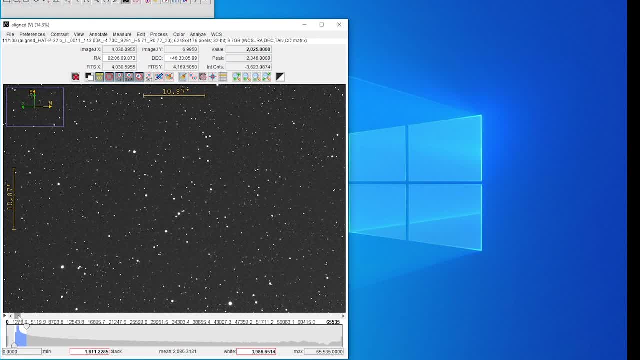 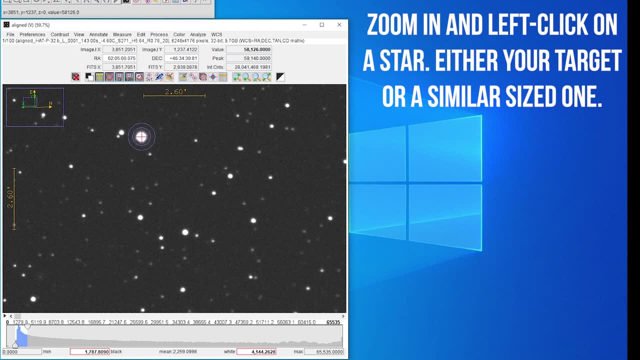 and this looks pretty good. okay, the next thing you need to do is find a star, and i like to find a star that's the size of my target star, or maybe a little bit bigger. here i'm going to find a larger star in my star field and i'm just going to left click it now, when you do this nothing, 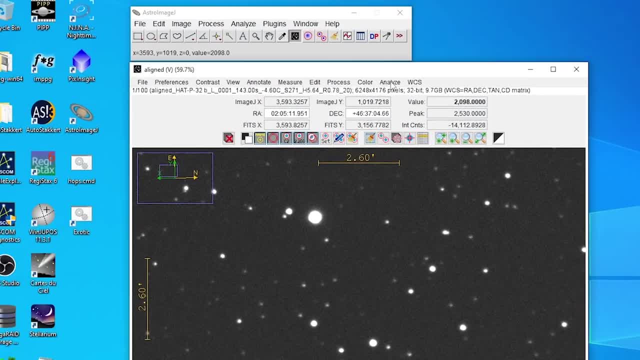 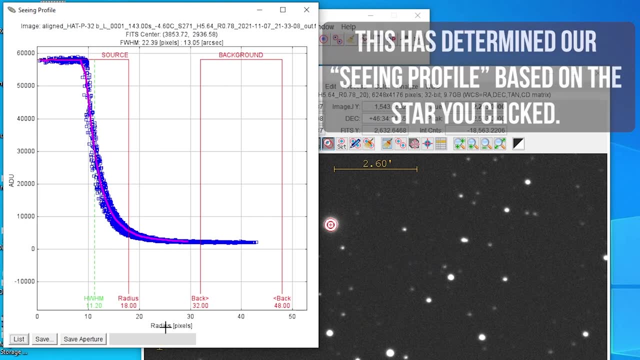 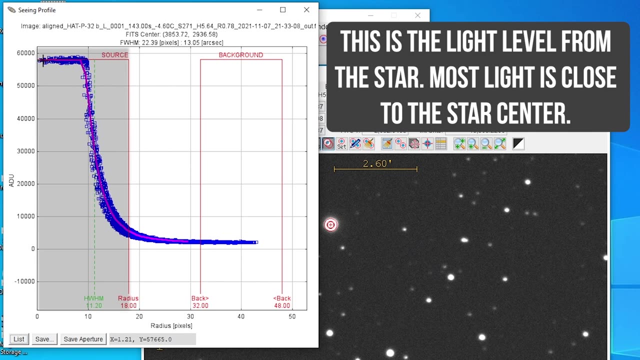 nothing noticeable will happen after clicking that star. go up to analyze and then plot seeing profile. this is the scene profile based on the star i clicked on the left hand side. this is plotting the light level. now most of the light from the star is close to the center of the star. 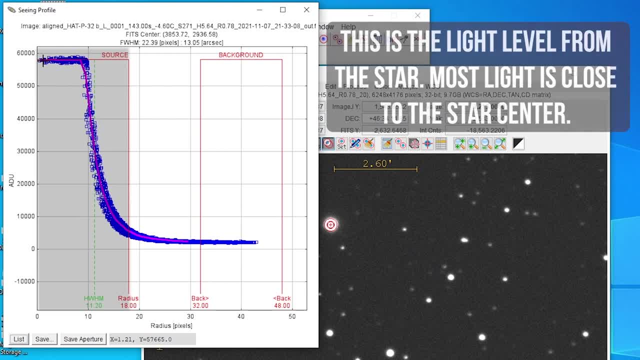 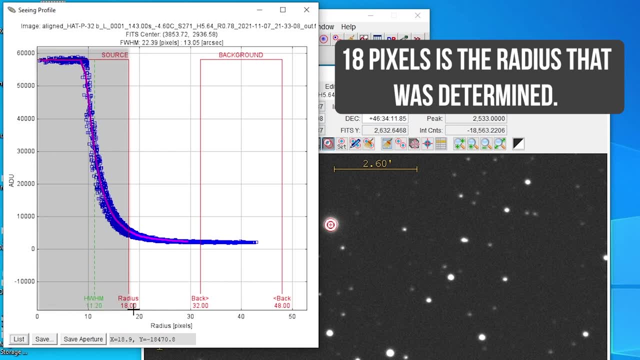 obviously it will even include some of the star glow around the edge of the star. the system has determined that from the center to a radius of 18 pixels is the aperture size that will be used. from radius 18 to 32 is sort of a dead zone we don't care about. and then we have 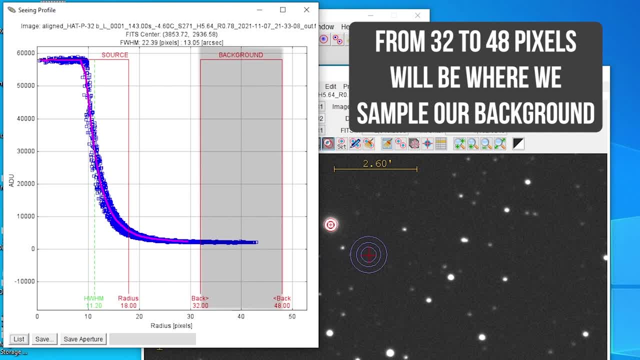 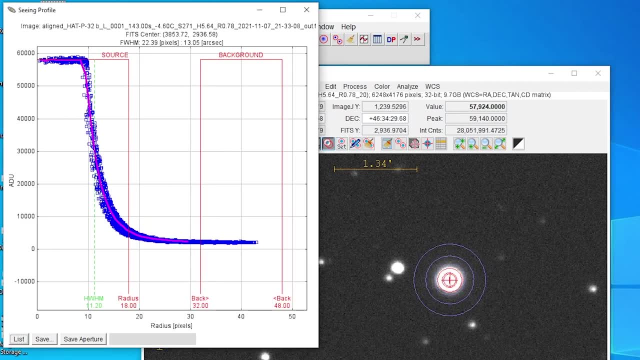 an area outside that from 32 to 48, which is where we're going to sample our sky background. so the way this is going to work, moving forward, is that we have target stars and comparison stars that we need to measure the light levels of throughout our entire sequence. the inner circle is where we 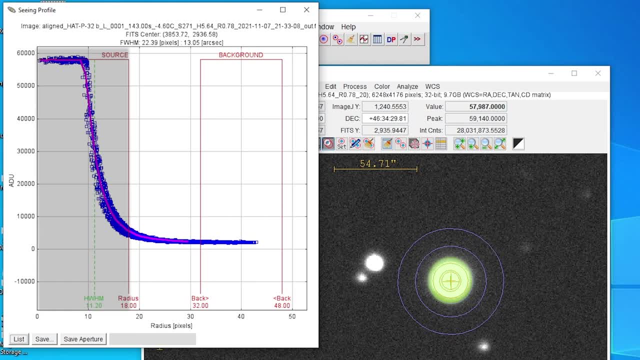 expect to see all of the light of the star. so the star itself, including the little bit of star glow outside of. that is called the aperture. then we skip a little bit of space and then we have a second ring. that's called the outer annulus. now, that area should not have any stars in it and should really just 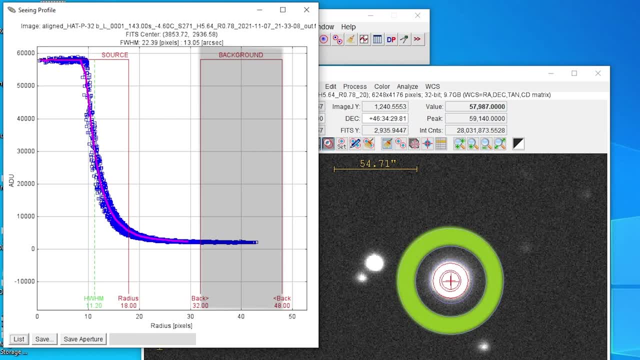 be background sky. we're going to take a mean value from that outer annulus and that'll be our background value. then, ultimately, what we'll do is we'll subtract that background value, which includes things like sky glow and light pollution, and subtract that from our inner aperture. 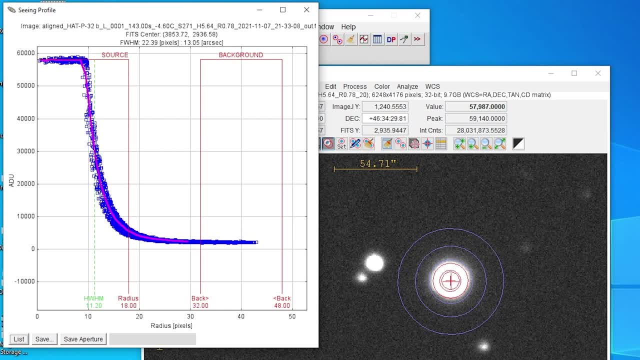 to give us a true value of the stars measurement in flux. if you're happy with the values you see here, you can click save aperture and that will be ported into one of our next steps. okay, so now we need to select our stars and start taking measurements, and we're going to click this icon. 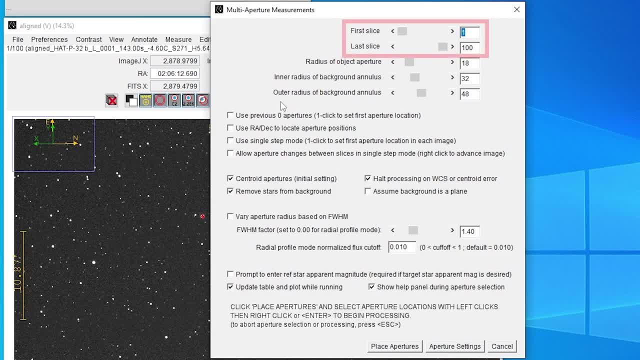 up top, which is the multi aperture measurements tool. when this opens up, make sure you're looking at all of your slices, from 1 to 100. notice that the aperture pixels have automatically pulled into this form. the next thing we want to do in this section is: in this section, we're going to 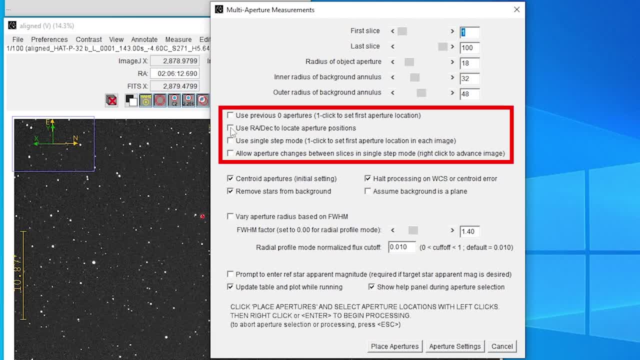 go to aperture settings and in this case we want to tell the system to use ra and deck to locate the aperture positions between slices. so we're going to start on slice 1 and select our stars, but we want to make sure we're measuring the right stars all the way through and we're going to use those. 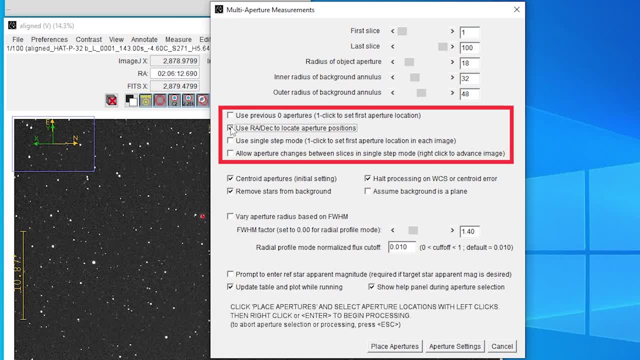 ra and deck coordinates all the way through our solved images to make sure it's consistently measuring the right stars. in this next section, uncheck, halt processing. that's not important for us here- and then everything you can leave here should be set up as default. we're going to go now. 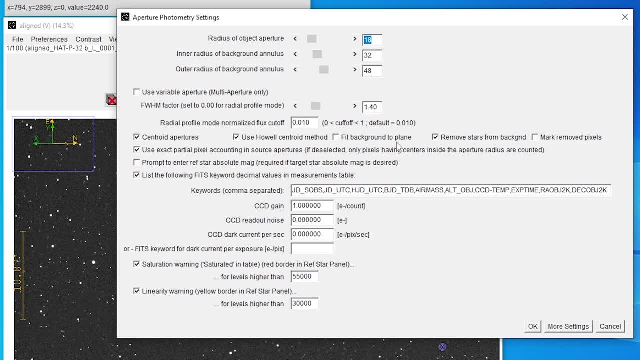 now all of this should be fine. your aperture pixel counts up top will be different than mine because you clicked on a different star in your own image and there's some other data you need to modify here, specifically related to your camera. so because i used my asi, 2600 mm from zwo, i'm going to 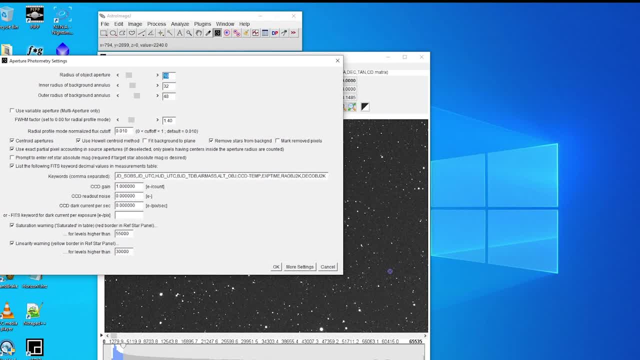 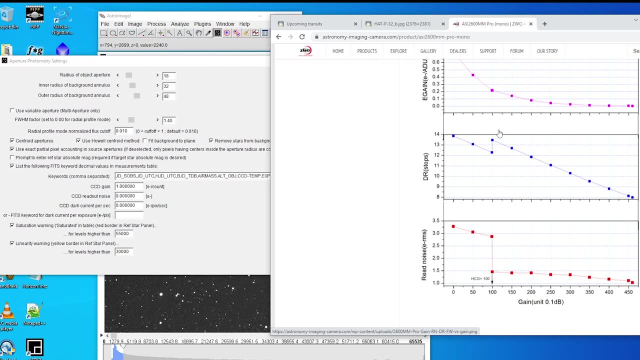 go to their website to pull some of this data. now i shot at 100 gain so i can go and retrieve these data points. the first data point i need to get back is my electron count based on my gain. so that's point two in my particular case. 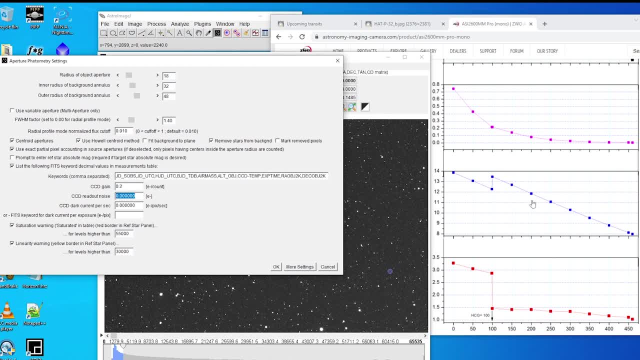 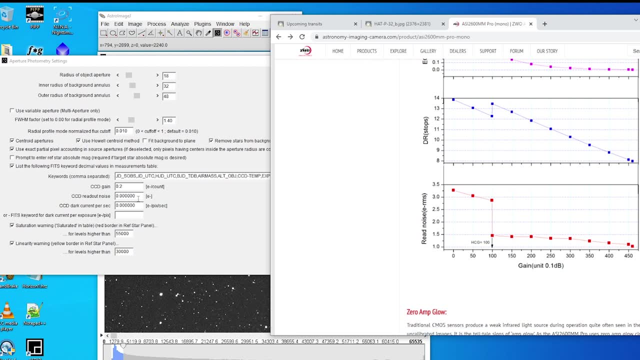 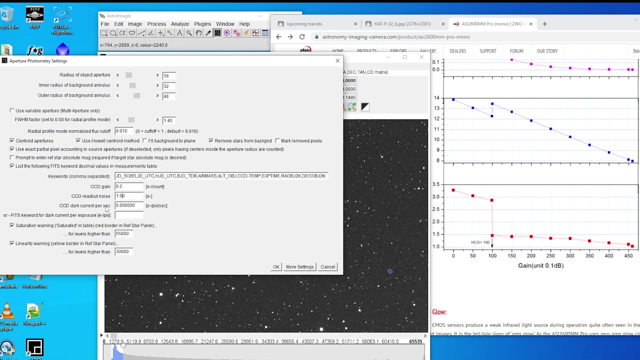 if you're shooting at unity gain, it'll be one. the next option is readout noise. the readout noise at 100 gain for me is right around 1.5. then i need to do my dark current and that's my electron per pixel per second, or you may. 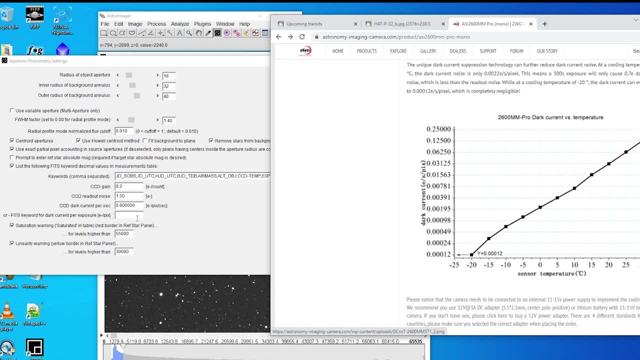 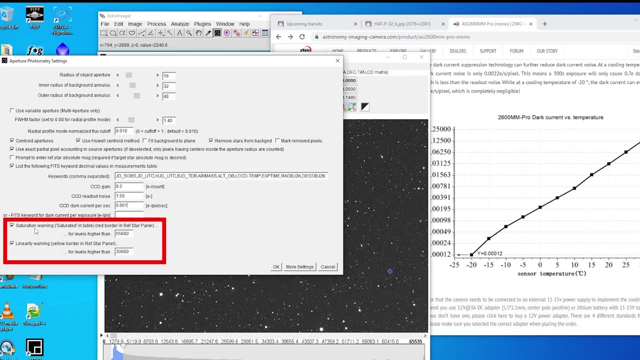 see it reported as electron per second per pixel. i shot at negative five degrees celsius, so i'm gonna go ahead and say point zero zero one. the last two entries here are related to your redacted camera or when those are reported at the same time, and then i'm gonna change that to: 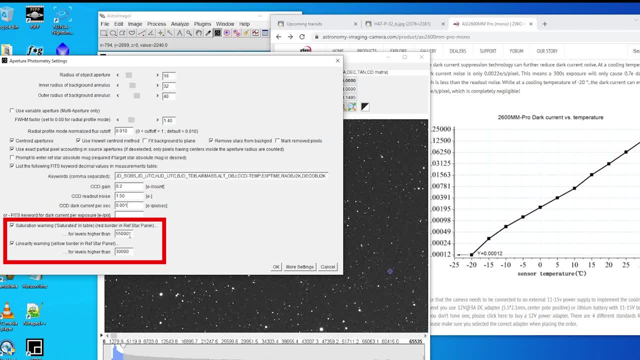 effect icon to say anything in right. there's a button here to change the color of the camera. so that's a little bit flow for that. and then this one is very important to me as well: if you can't find this data, don't worry about it. what this really is talking about is: when will you? 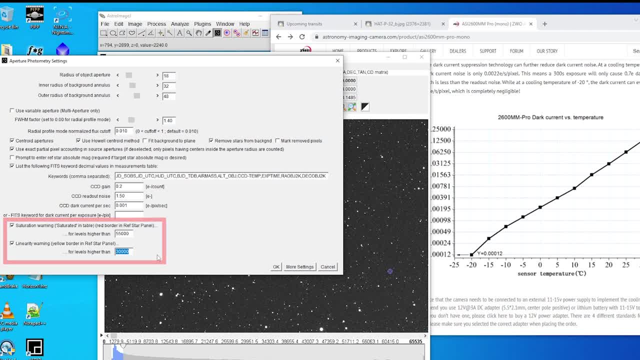 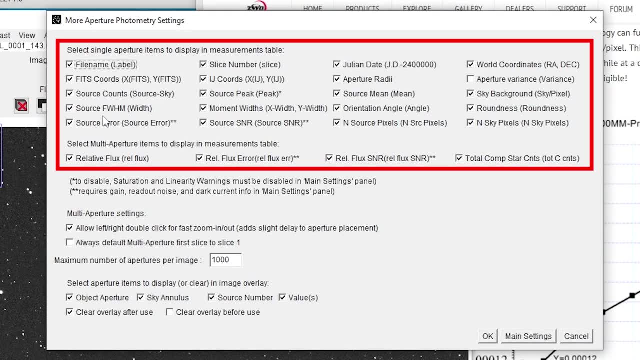 be notified by the tool. so, because a 16-bit camera has values from 0 to 65, 535 is a general rule in my research. unless you have specific data about your camera for these settings, you can usually set reported or calculated by the system as it processes all of your images. you can. 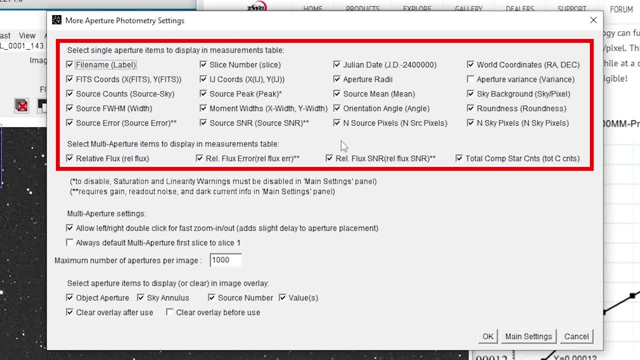 leave it all here, but you may find over time there's pieces you just don't care about, and it'll make your data easier to look at if you get rid of some of these data points. so I'm gonna get rid of a couple here that I know I don't need and 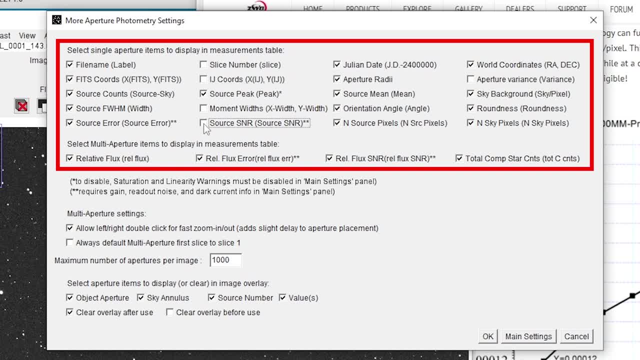 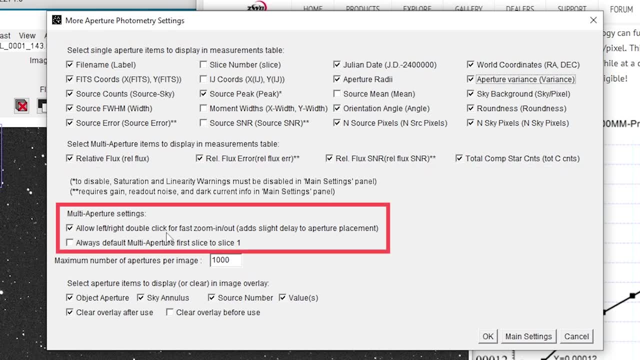 you probably don't need either. there's actually more you could get rid of, but we'll just start here. also go down here and check the checkbox to tell the system to always default multi aperture to the first slice in the stack. it's really easy to get off that first slice when you're kind of looking around at. 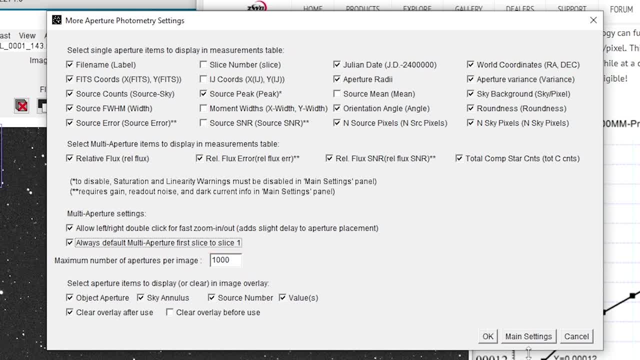 your images and some of the things that are done by this product will start at the current slice, which could be problematic. we always want to look at the entire sequence. everything else here should be good. we can go back to our main settings and then we'll click OK, now we're ready to click place. 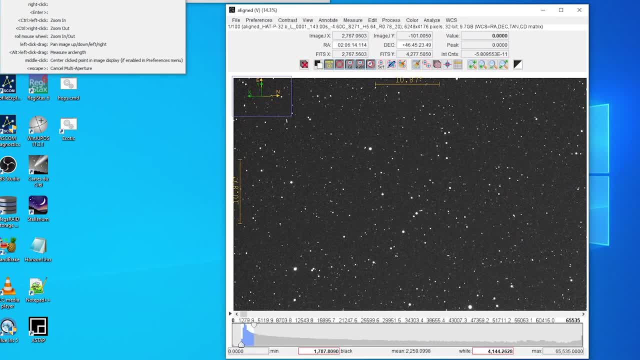 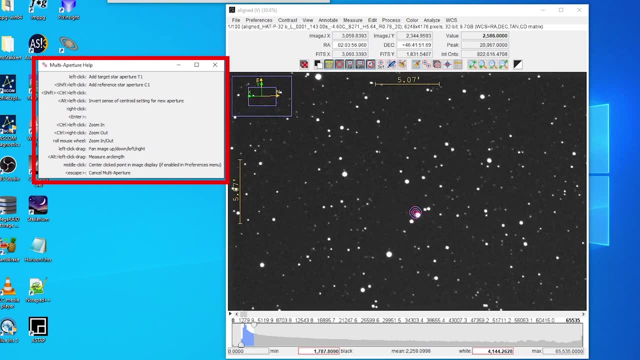 apertures. now you'll notice you get a little help menu that pops up on the left and it's first telling you that you can add your target t1. right, this is your target star and you need to know where this is in the image. but all you need to do is find it and left click on it. notice when I'm 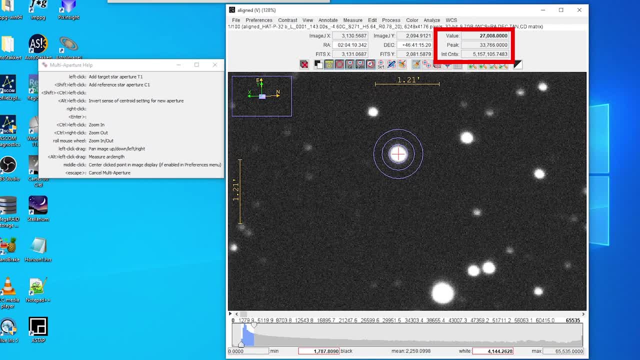 mousing over it that up top we have a value of peak and in count, remember, the value is the pixel. I'm over at the time. the peak is the highest valued pixel within that inner aperture and the int count is the total value of all of the. 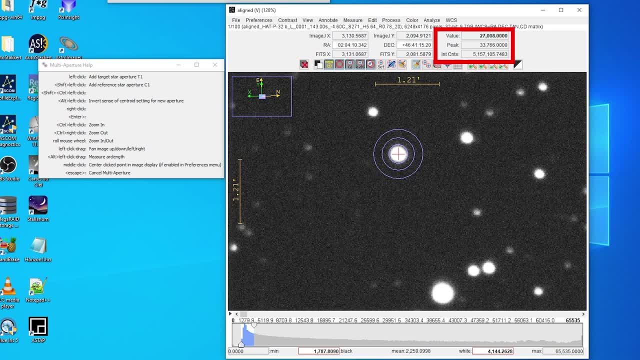 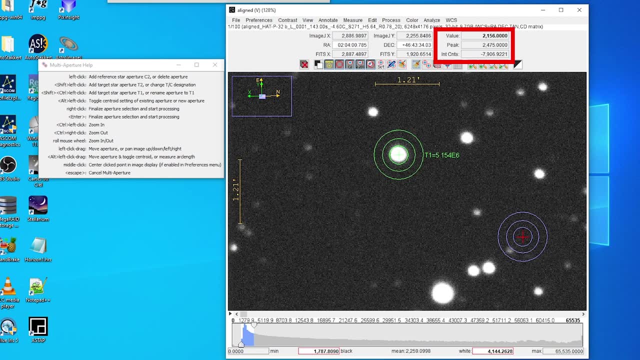 pixels within that inner aperture. this becomes important because we usually want to find comparison stars that are similar to our star. so if you know the values of your target star, when you mouse around the screen you can try to find other stars that have similar values. now notice after. 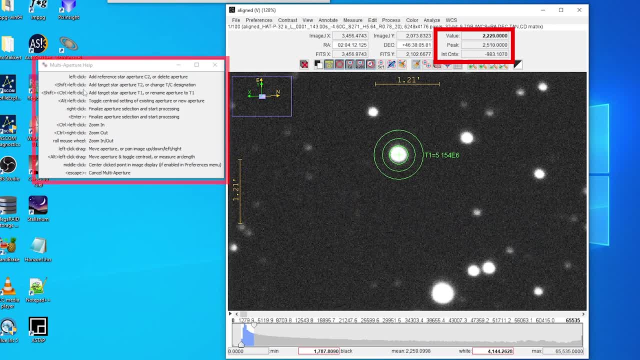 clicking our target star, the help menu changed up. in the help menu it now says: if we left, click an additional star, this will be c2. so it'll be our comparison. your initial target star is t1 and your comparisons are c2, c3, c4 and so on. now 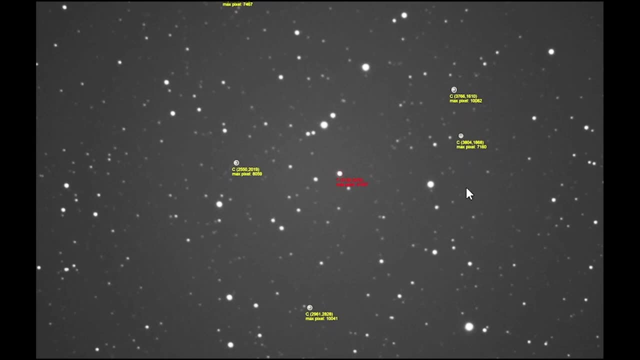 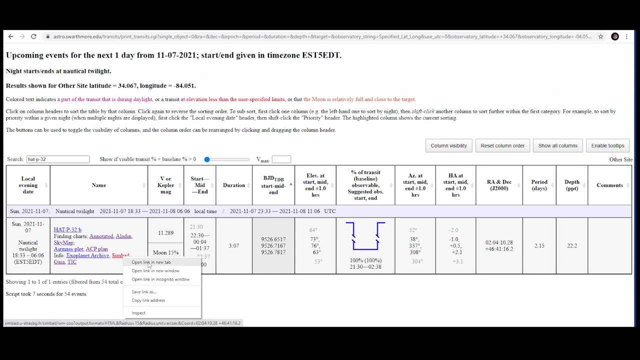 how do we know we got the right star? well, one way is to go back to the image provided by the plugin in nina. that will label and show you your target star and your target star will show you your target star and you can also go back to. 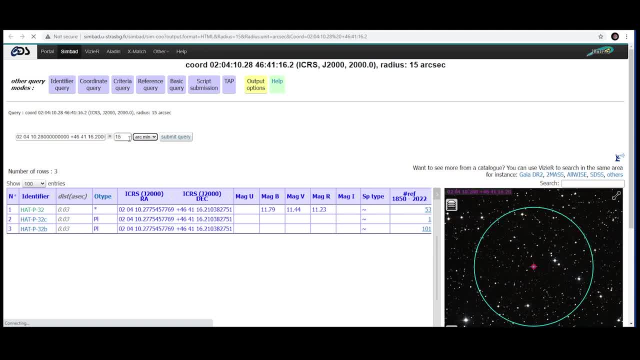 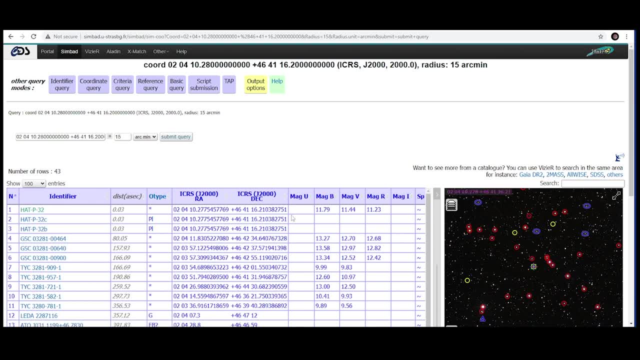 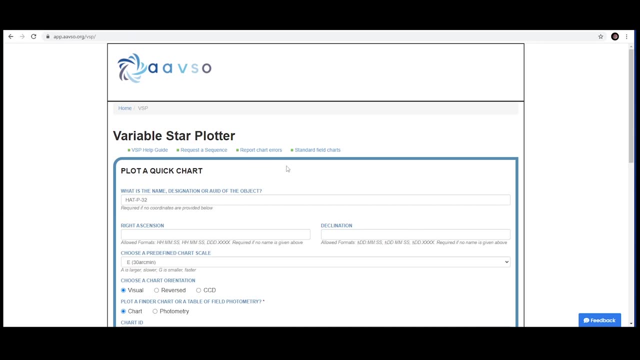 the transit finder and use the data from there, including something like a SIM bad lookup. now, this can be much more complicated than it needs to be now. another tool you can use is something like what's available from avso or aavso. when you search and find your target star, we'll show you a graphic with the. 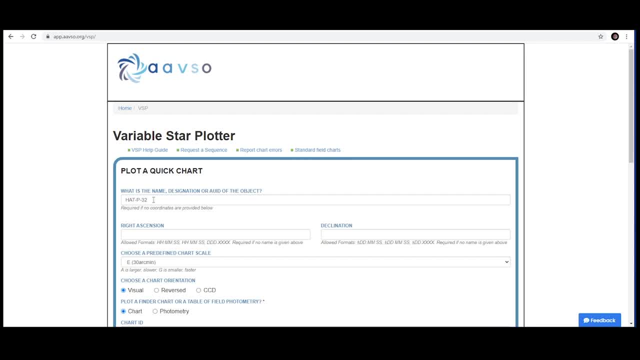 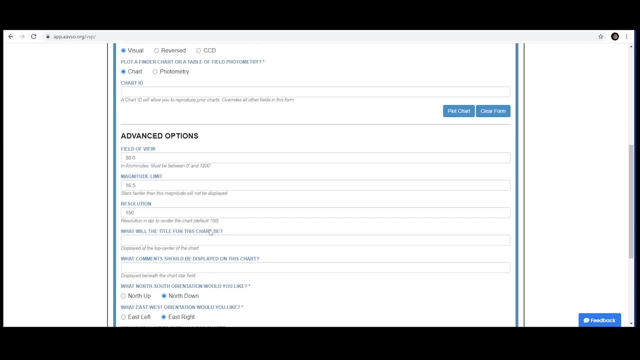 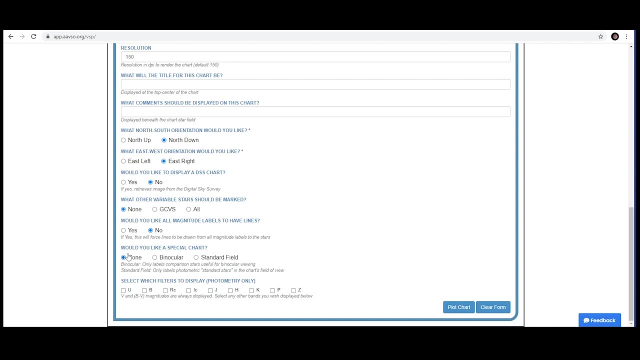 immediate field of stars around your target. it'll identify some potential comparisons and can even show you variable stars that you should exclude. it's important we don't use variable stars as our comparison stars, because we want the only variable star that we're looking at to be our target. 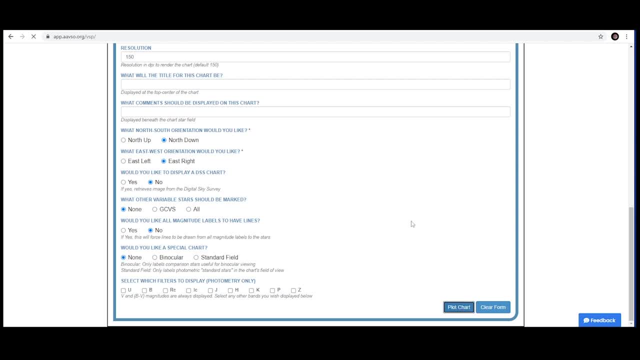 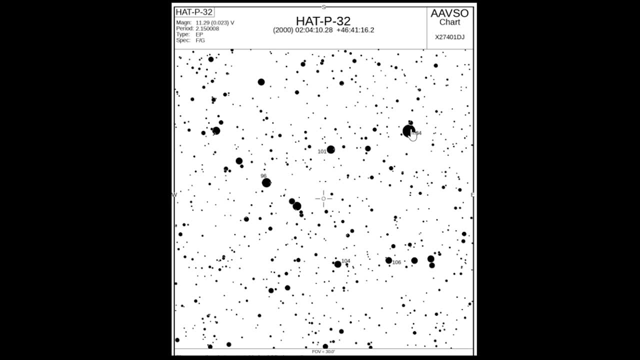 star itself, which is variable and light level because of the transit. so if I look here and I see there's a large star, that it's identified, I can go back, based on this graphic, and find that large star and see if that's going to work as a 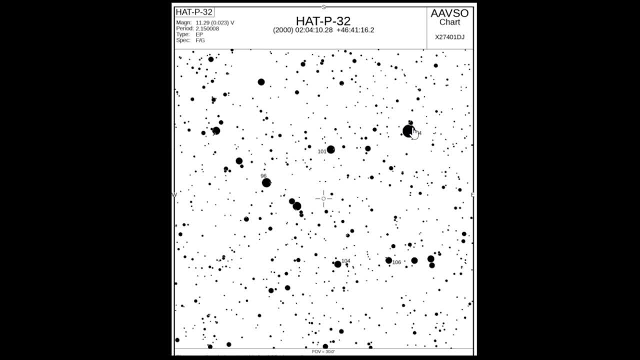 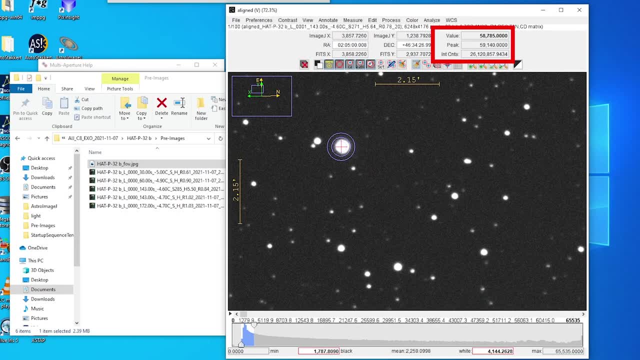 comparison. now, in this particular case, for me it's not going to be a good comparison. it's not a good comparison because when I mouse over that large star, due to the exposure length that I used, this particular star became saturated right. it's got a really high value and peak because of that. I 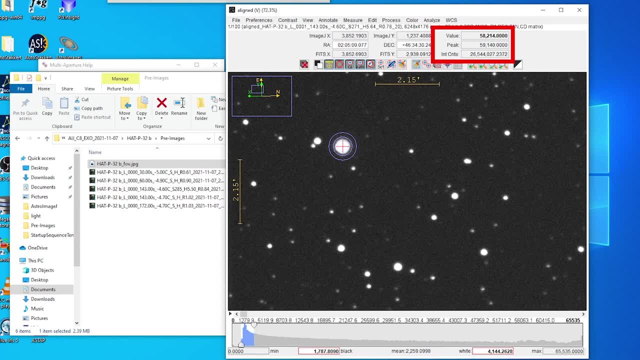 probably want to stay away from it and I'll be forced to find other comparison stars. now you can use all the tools that are available to you, or you can just kind of give it a shot here now. remember: this aperture that we're using is very important, because not only does it define where we get our data points for 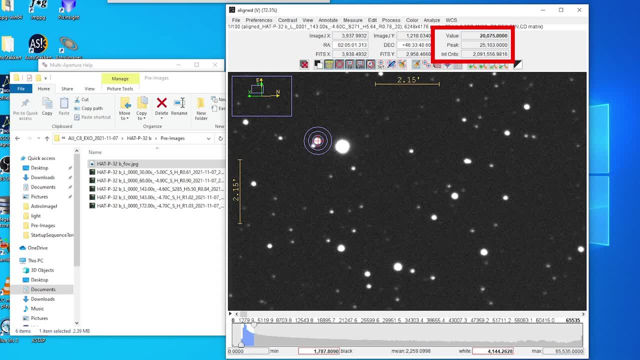 the star itself, but it also tells us for that star how to sample the background sky. so stay away from stars like this with other stars nearby, because you may get a bad background reading as a result of a nearby star, which could then diminish the flux level of the comparison. so let's go look around and 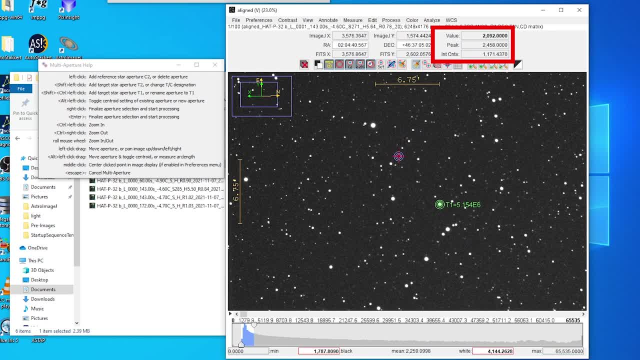 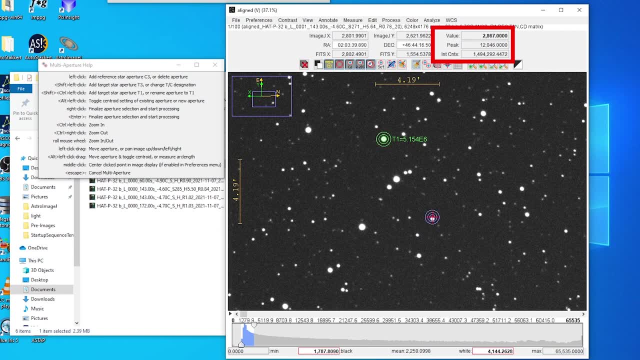 we'll try to find some stars that will work for us. as I go around and mouse over various stars, I'm looking at the levels in the upper right hand corner and as I find some that works, I can left click and select them. now one thing to. 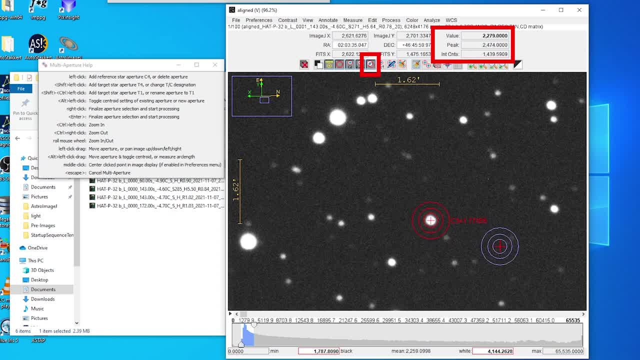 note is you don't have to click the star perfectly. even if I click off center, it will automatically Center the aperture because by default this icon up top is selected, which tells the system to behave that way. so we go around, find some new stars that could be good comparisons that don't have other 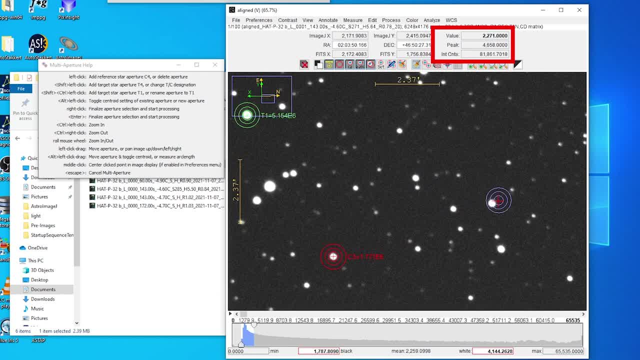 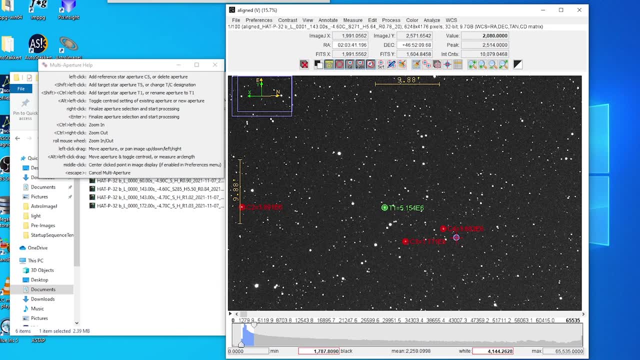 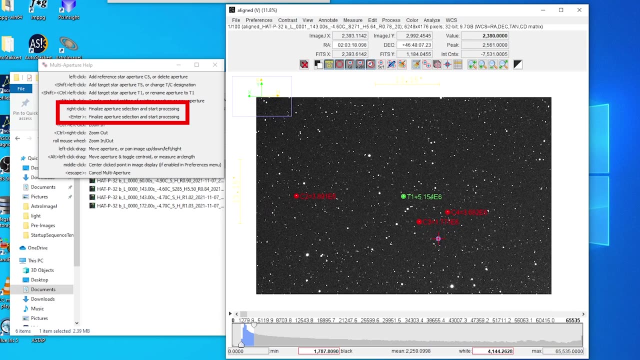 nearby stars and I'll select a couple. so we have our Target and some comparisons ready. we can look at the help section over the left and it tells me either to right click or press enter to proceed. now I want you to prepare yourself for what's about to happen to the screen. 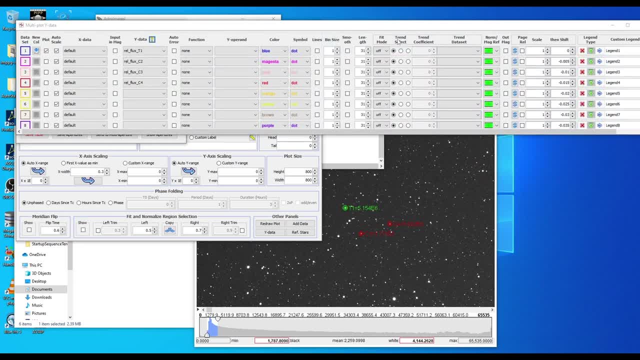 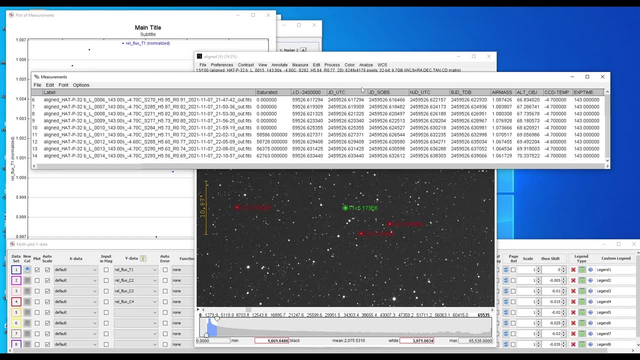 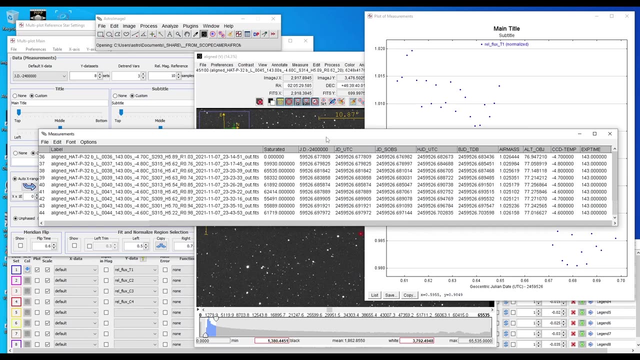 once the processing begins, a lot of things open. now I'm going to speed this up pretty dramatically. this can take a little while. the system is going to go through every single image and on every image it's going to look at every Target star and comparison star you identified and it's going to calculate a lot of data. 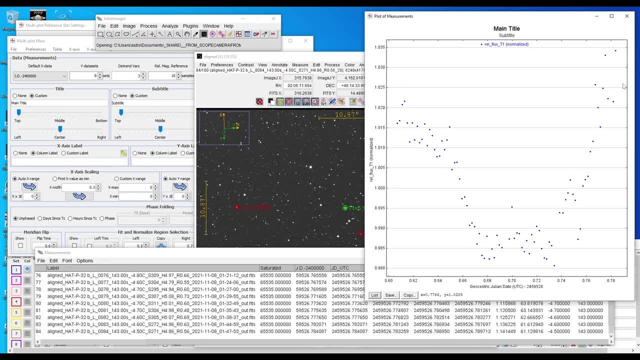 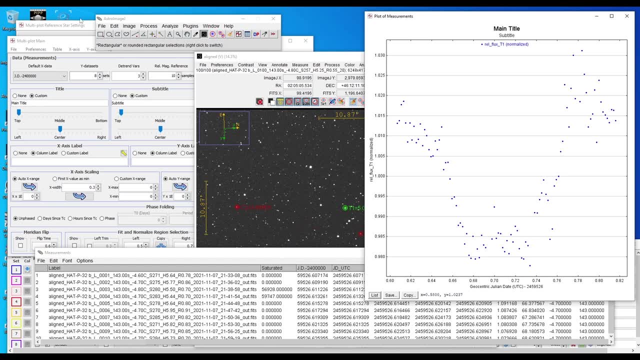 and put it in this measurements table. you can watch the measurements table as the process progresses, as well as, potentially, the graphic being plotted as well once it's done. one of the first places we want to look is here at the multi-plot reference star settings and notice that I've got some different. 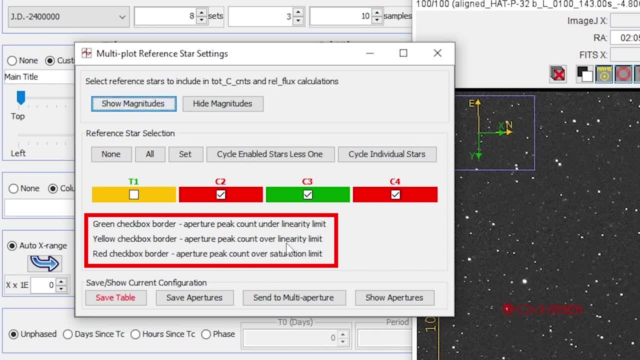 colored stars. so for my t1 it fell on the yellow category, which is not ideal, but I'm not going to be able to go back and do anything about that at this point because my Target star is my Target star. there are no alternatives for that one. 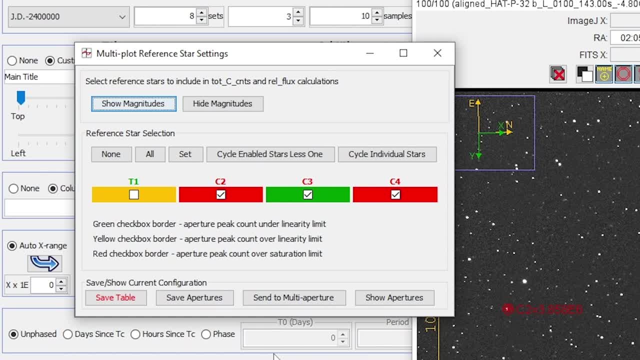 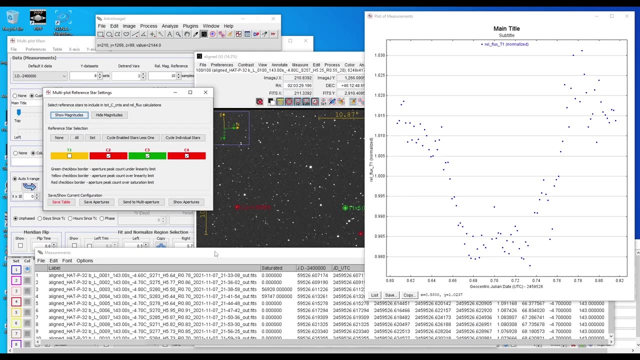 but notice that my comparisons here, notably two and four, are in the red. level means the star is recorded very high values for their peak counts. now that makes these particular stars as comparisons potentially not ideal. so if we just want to look at this, we can go into 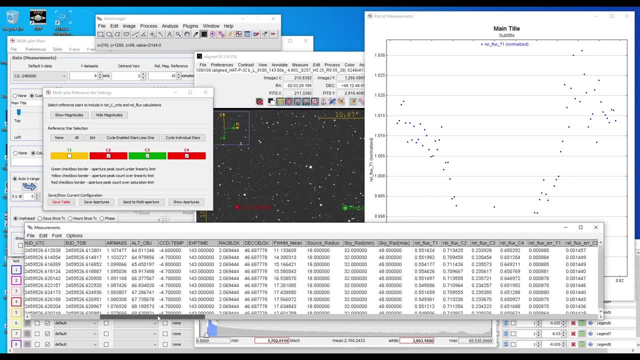 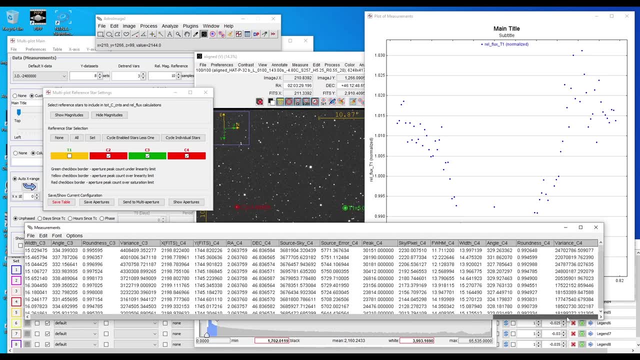 the measurements table. so the measurements table from left to right is ordered by Target and then comparison 4. so if I scroll all the way to the right I can get to the comparison four star data. specifically in this case, I'm going to look for peak C4 to find the peak values in. 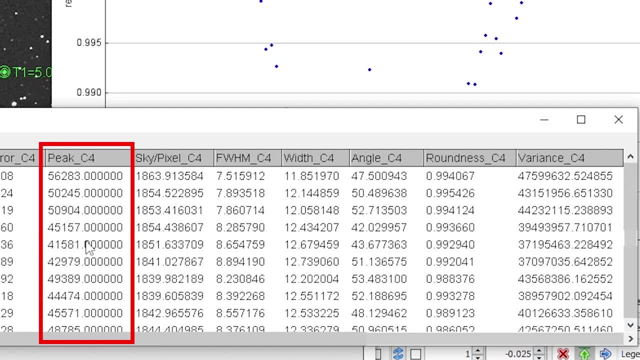 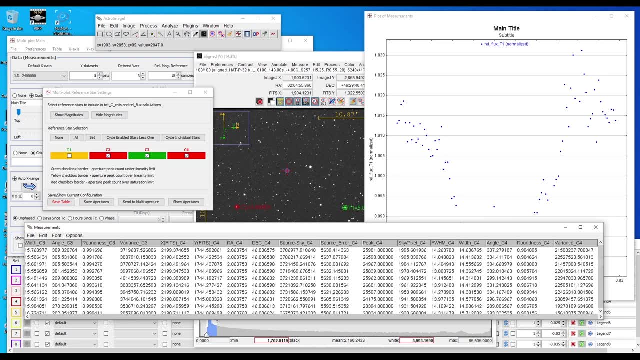 every one of these images for that comparison star. you'll notice, at some point I started getting values above 50,000. remember I defined a threshold at 50 000 earlier. that's why this was flagged as red. now, to fix this, I'm actually going. 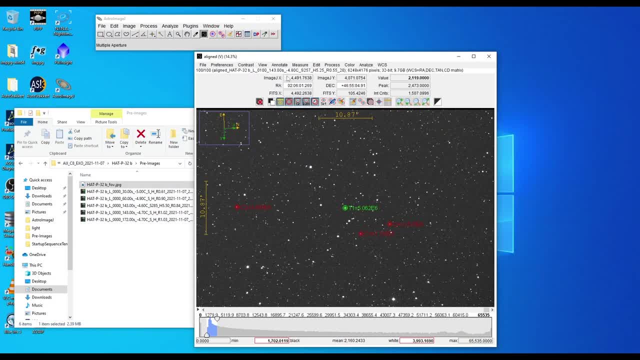 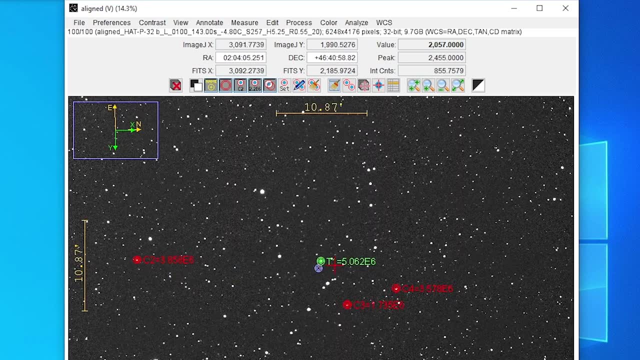 to have to pick new comparisons. so I'm going to close everything except for the image sequence and the smaller AIJ window. Now I've got my comparisons still on the screen marked and I can see where those stars are, and what I want to actually do is select new comparisons and sort 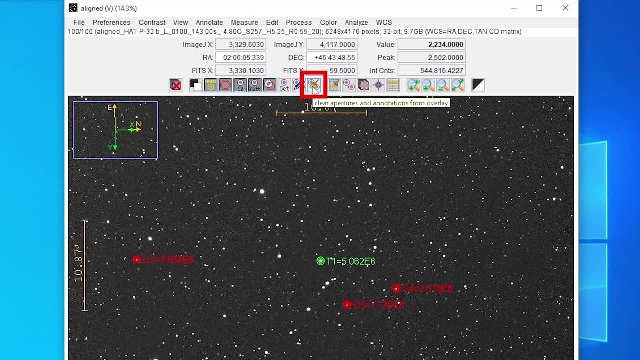 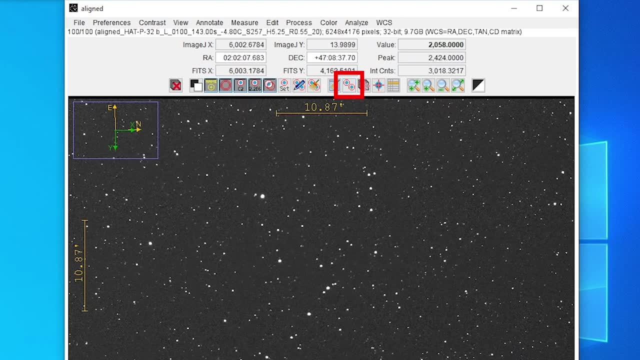 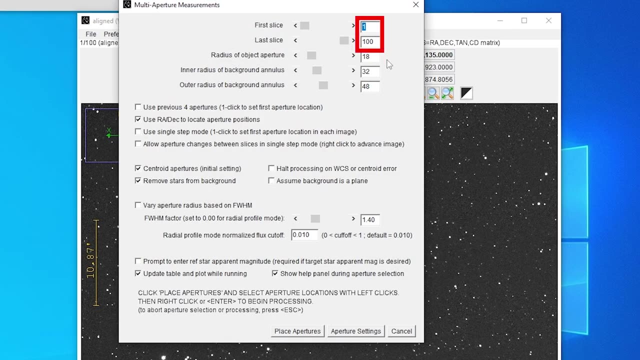 of start over here. To do that, I'm going to clear my previous comparisons by clicking this icon and I'm going to select some new comparison stars. To select new comparison stars, I click the multi-aperture button again. Make sure I'm looking at all of my slices and make sure that I do not have using previous. 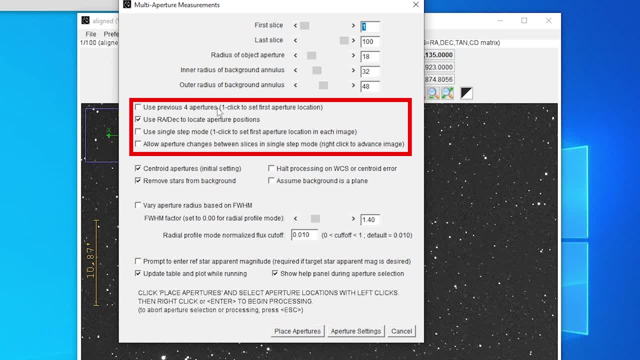 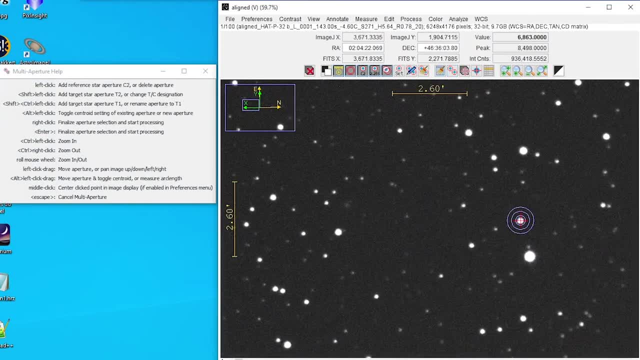 apertures clicked. I still want to use Arian Deck and I'm just going to start over. by clicking place apertures. I'll find my target star once again and I'm going to go find some new comparisons. Now, when I right click or press enter, it'll go through and calculate the data. Now, in this case, 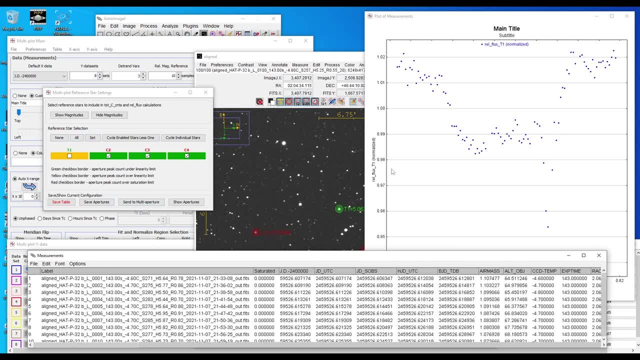 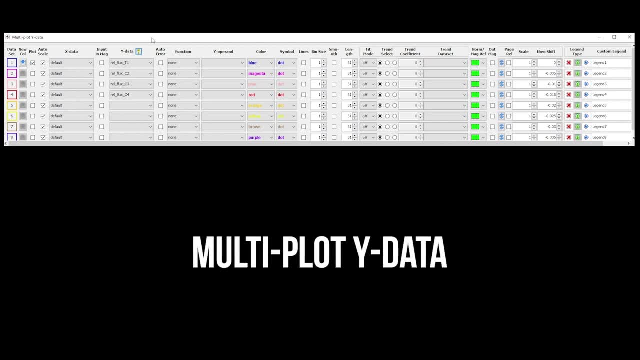 I selected better stars and you can see that all of my comparisons are fine. It's only falling in the green. I want to talk to you a little bit about how the data is plotted and look at some additional information that was calculated. So let's go through the important pieces of this window. First, we see we have eight potential data. 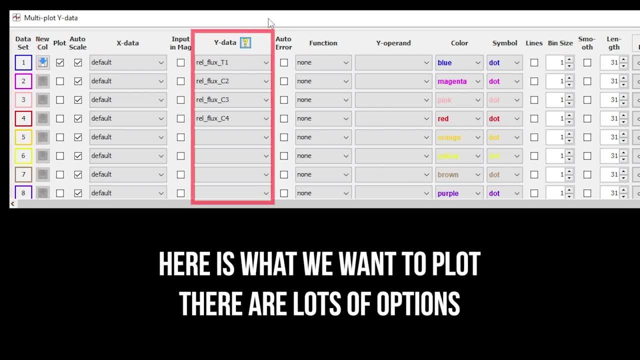 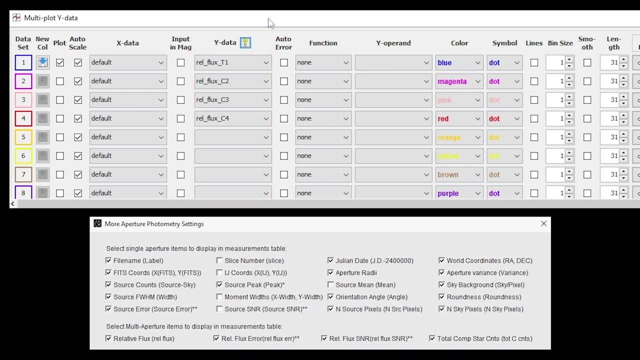 sets or eight lines. Next, we can see what is being plotted on each line. There are a lot of options here, though, and if you remember this particular window, that's where these options came from. One of the first check boxes for each line is whether we choose to plot or not plot the line on. 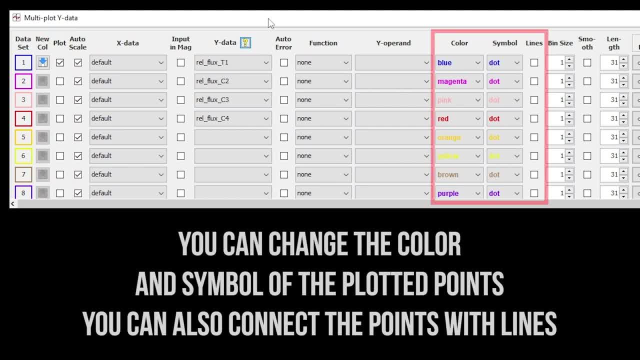 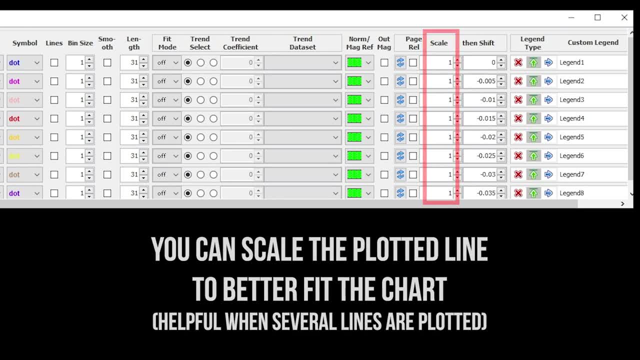 the graphic, one thing plotted right now. we can also choose the color symbol and whether or not the symbols are connected by lines. we can also scale the data as needed and even shift the data being graphed up or down to prevent it from colliding with other data that we're graphing simultaneously. 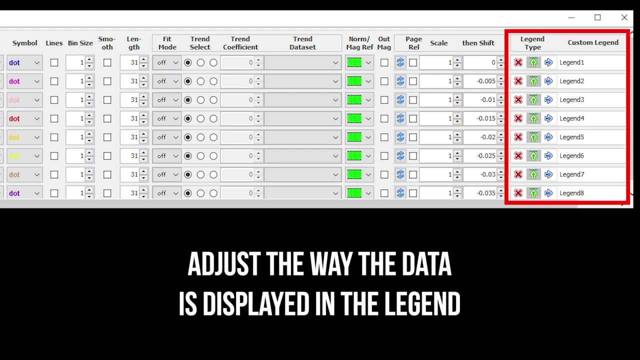 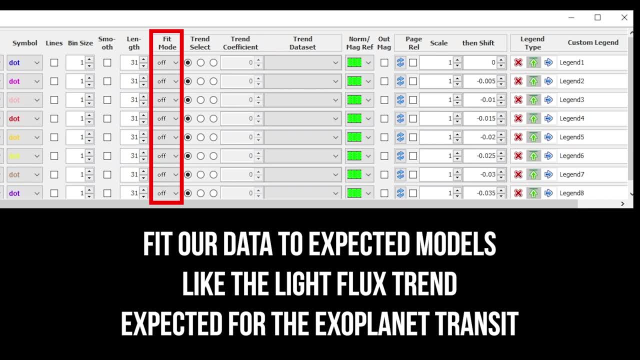 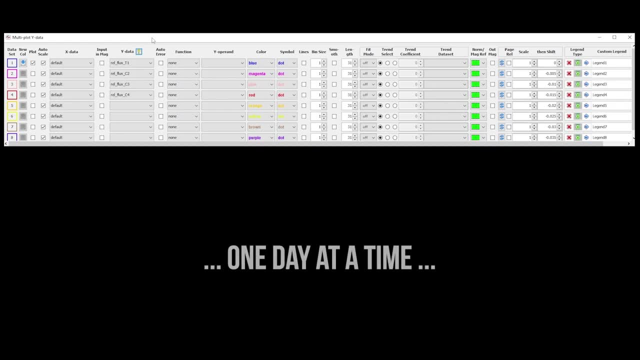 we can also change or modify the legend to identify any of our plotted data and can change the fit mode so that we can fit our data to other expected models, like a typical planetary flux based light transit curve. what about all the other stuff? we're going to leave that for another day. 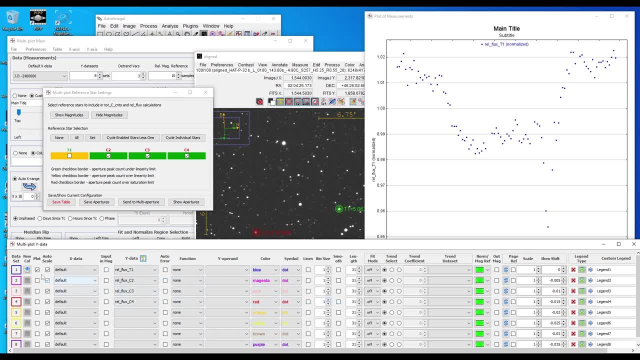 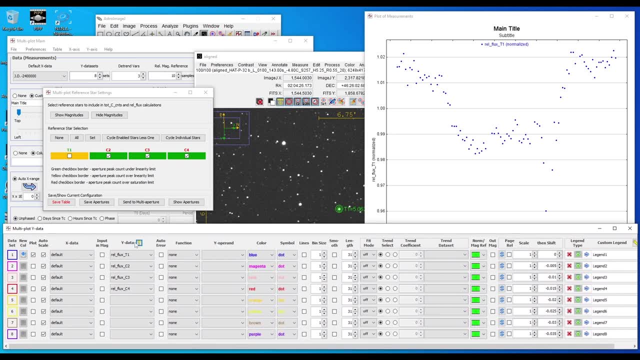 so let's go back to our full screen and look at this in practice, specifically for our only piece of data plotted, which is our relative flux of our target star t1. so over here i can uncheck or check the plot of this and you can see when i uncheck it. it goes. 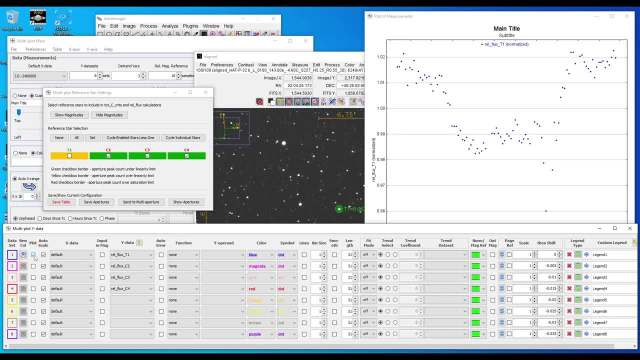 away from the graphic and then it'll come back when i recheck it. you can see i'm plotting relative flux of t1. i have colors and symbols and i can enable the line feature here to connect the plotted elements, and i can also manipulate what those plotted symbols are. i do have this blemish here that 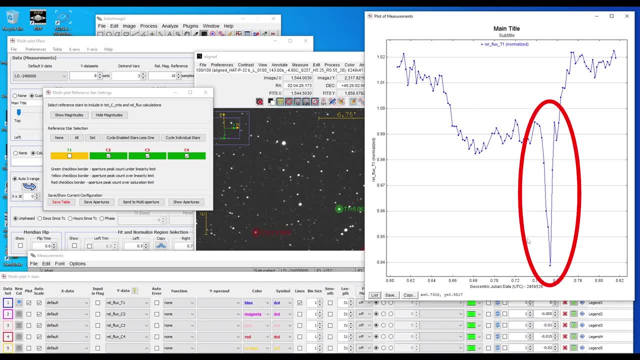 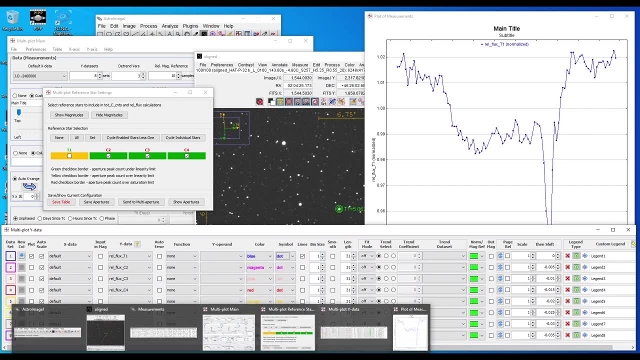 i want to deal with. so i may need to go back into the measurements to take a look at that, and it seems to be about two-thirds to three-quarters of the way through my evening, so i'm going to scroll down and specifically, i want to look at the relative flux of t1 because 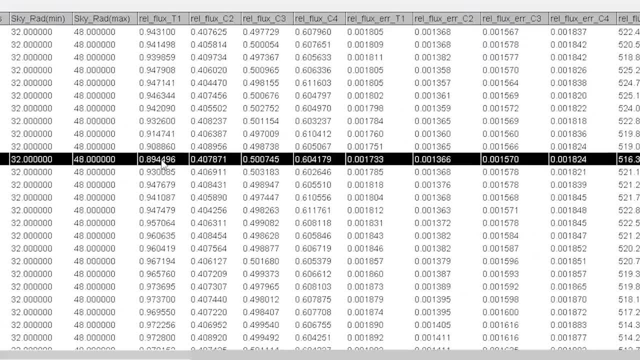 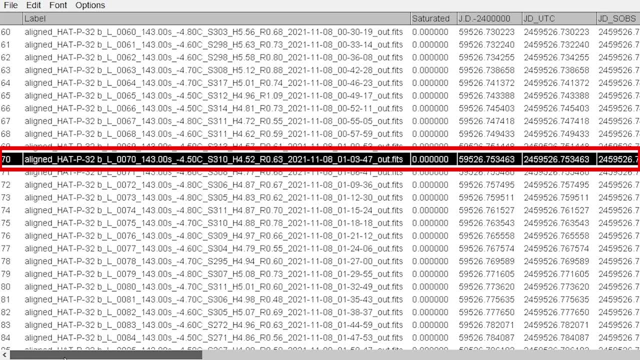 that's what's plotted and i can find that here. so i'm going to scroll down and specifically, i want to look at the relative flux of t1, because that's what's plotted and i can find my lowest data element in that data set is this 0.89 number. 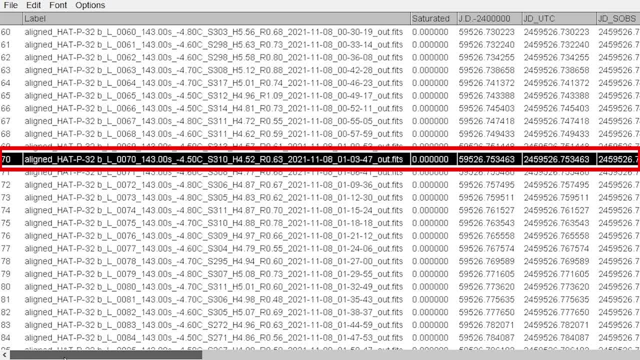 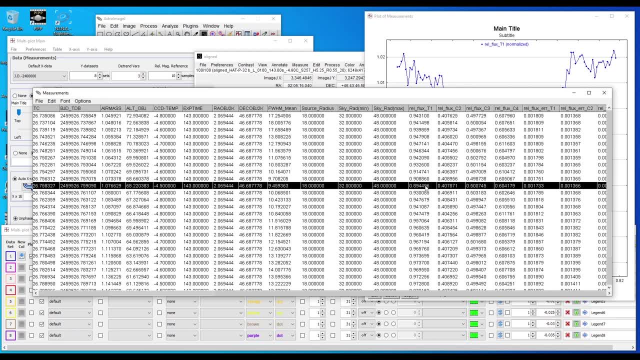 and if i scroll over to the left on that particular line, i can see that that is slice 70, which should correlate to my image 70.. now i'm not totally certain why the relative flux happened to drop at that point, but it may just be an artifact of my night sky. so now that we know it's slice 70. 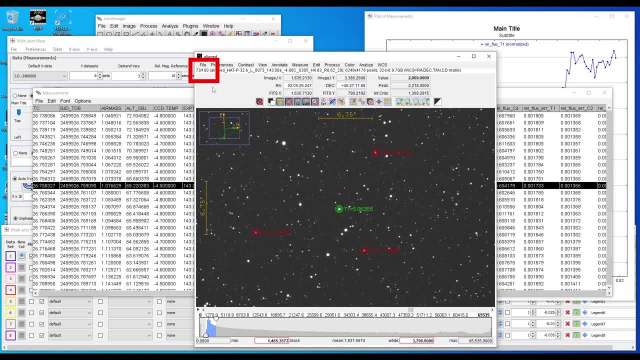 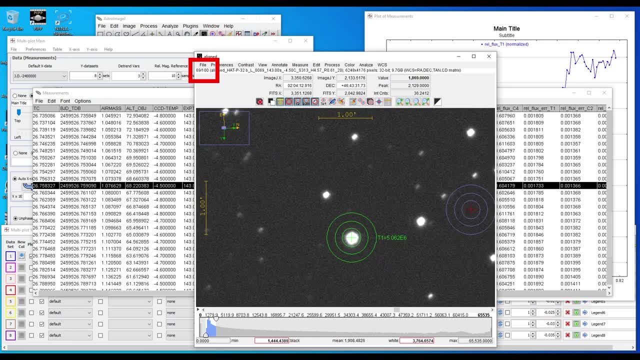 let's go look at slice 70 and see if we see anything. so i'll go back into the image sequence and i'm going to go find around 70 and i'll move back and forth through a couple of those images and it's kind of interesting. maybe the star gets a little smaller. so let's go into the table and 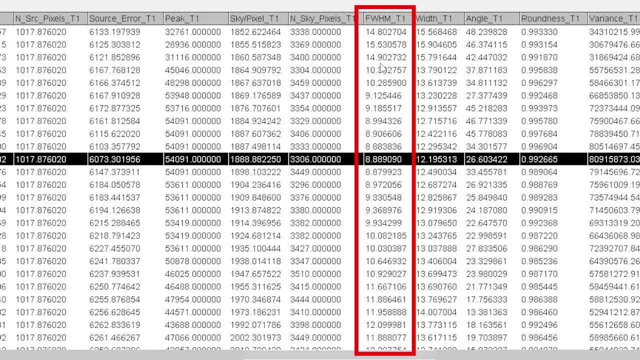 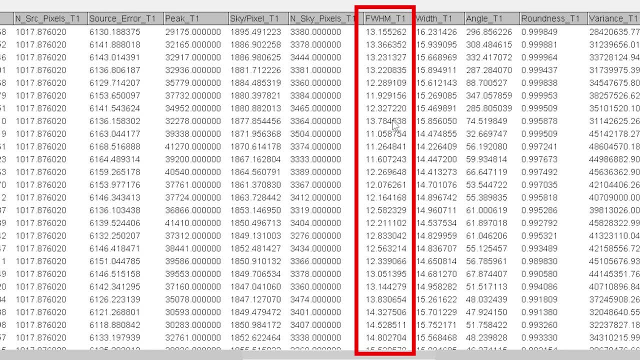 look at fwhm for t1 and you can see that it actually started pretty high and then got pretty low. so this is obviously a little unusual. i wouldn't expect my star to get smaller unless my seeing conditions improved or my tracking improved. but it was just a handful of minutes here. 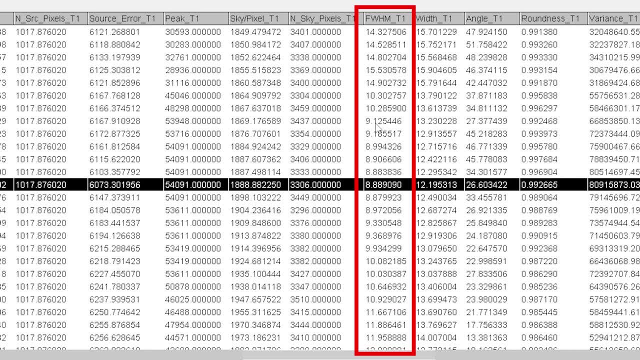 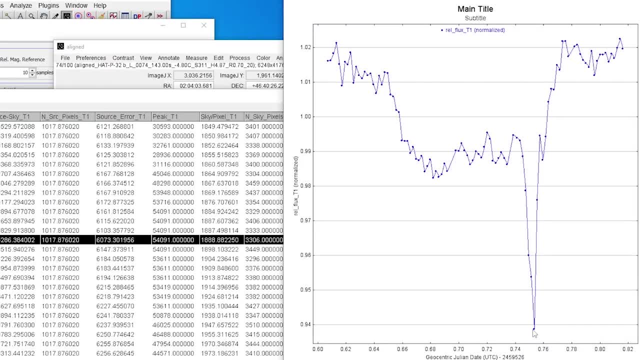 so i'm going to take this to be sort of an anomaly in my data, so i'm going to choose to exclude this from my data collection. now, personally, i don't find a problem with removing data when it's explainable. i can see what happened to my data: either my guiding got better or my sky got better. 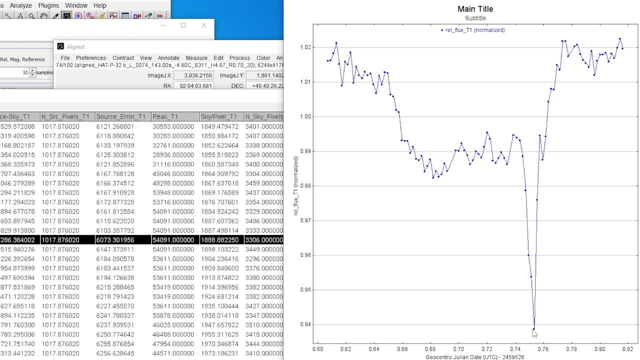 temporarily, but it's obviously an anomaly from the rest of my data set. so let's see how we can get rid of these particular data points that are causing me a little bit of a problem in my curve. and remember, i'm not advocating getting rid of data you don't like. 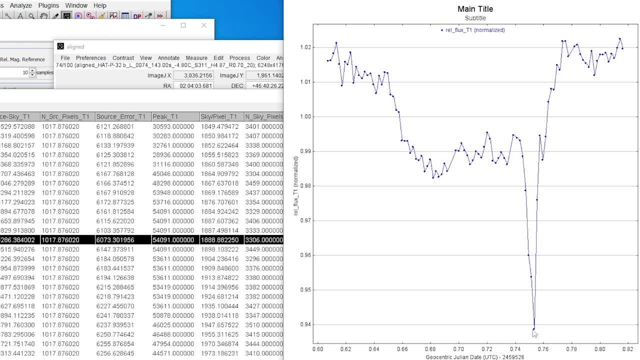 because it's not pretty. i'm telling you that i know i have a problem in my data set based on acquisition and i'm going to get rid of those particular data points. so i can look at the graphic and i know where 70 is. so if i go back, that's 70, 71, 69, 68, 67. so if i get rid of slices, 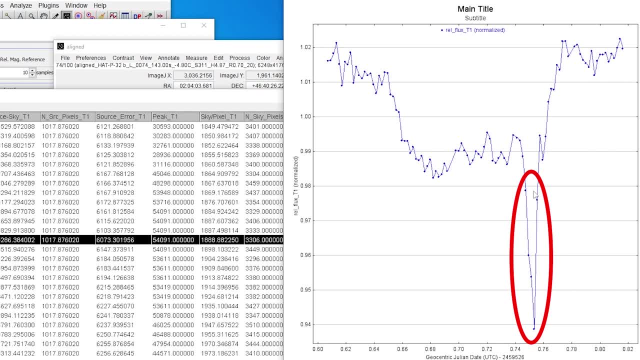 67 through 71, i'll probably get rid of this anomaly and give me cleaner data to work with. so the easiest way to do this is within aij itself. we don't have to do a lot of work to get rid of this anomaly, but we can do a lot of work to get rid of this. 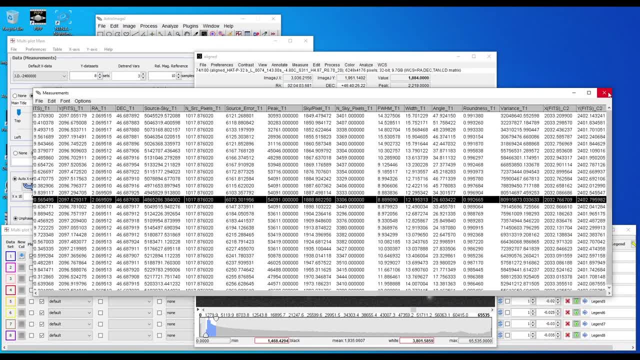 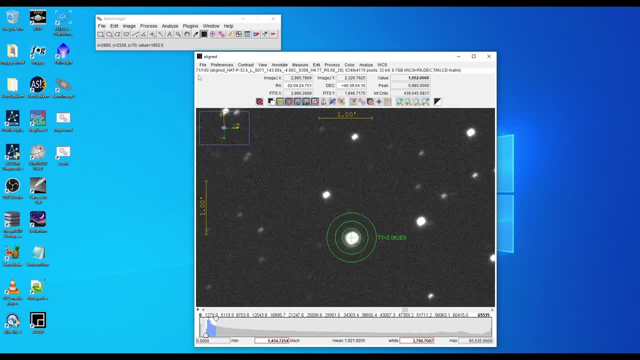 anomaly. we don't have to delete the images, we can just delete the slices. so i can close it all out again, except for my image sequence window and if i go to the sequence and if i find the highest slice that i want to get rid of, in this case number 71, once i'm on image. 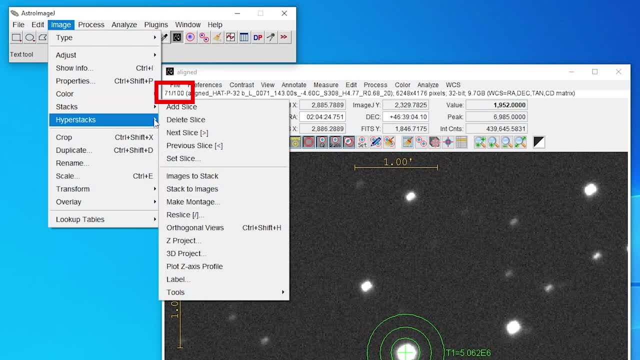 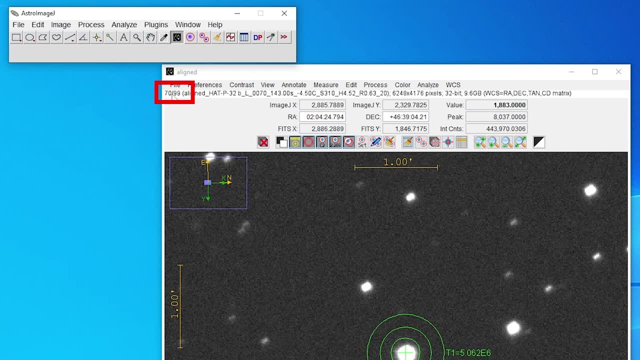 slice 71, i can go to my main astro image j window and go to image stacks. delete slice and i'll delete the slices from 71 back through 67.. now i'm going to speed this up a little bit here. now notice, when i go into my 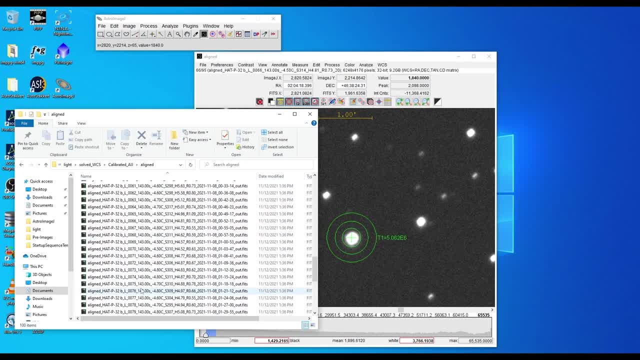 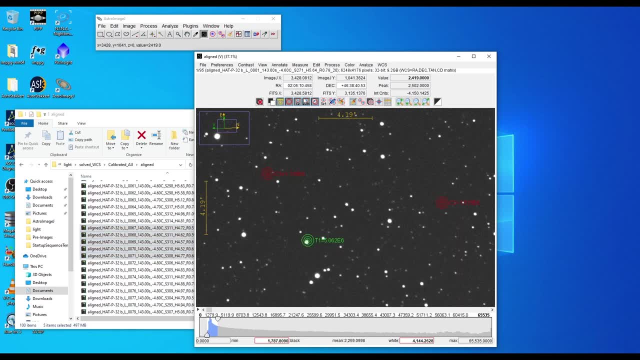 image folder. even though i've deleted the image slices, i did not delete the images. i've deleted the slices in the stack that aij is working with now. because i've removed slices, i need to reprocess my data, so i'm going to go ahead and clear my apertures and add new apertures. 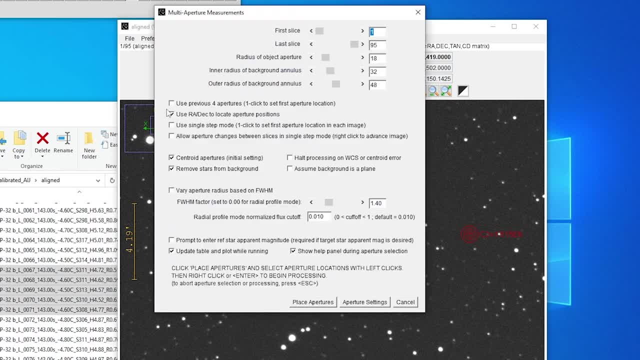 now, in this particular case, there is another check box we can check to save us some time because we know we had good comparison stars, rather than trying to find comparison stars again when we come in here. what we can do is click, use previous four apertures and this will basically. 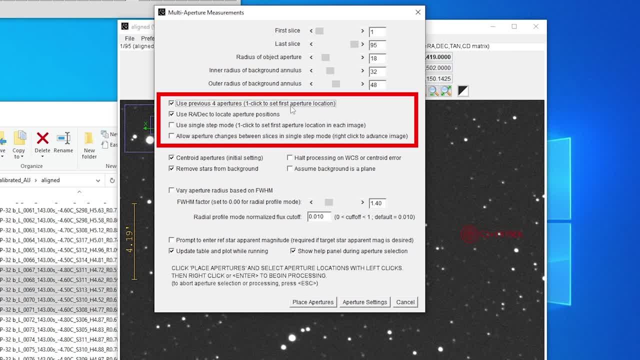 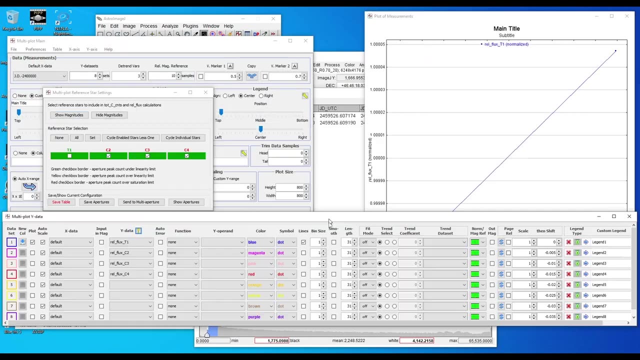 tell my system to reuse the apertures that i just defined. make sure we've got all of our slices here. in this case it is not from 1 to 100 anymore because we've removed some slices. that's okay, and we're going to go ahead and let it calculate. remember to calculate. it's a right click, or? 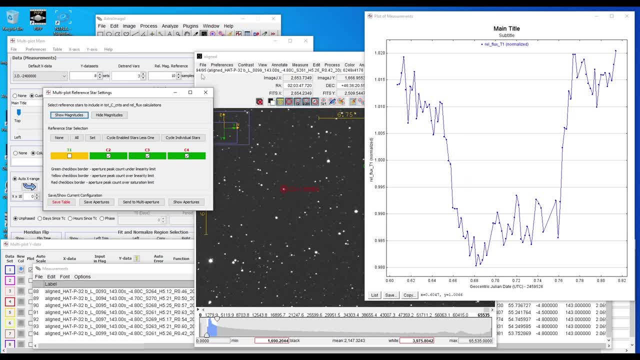 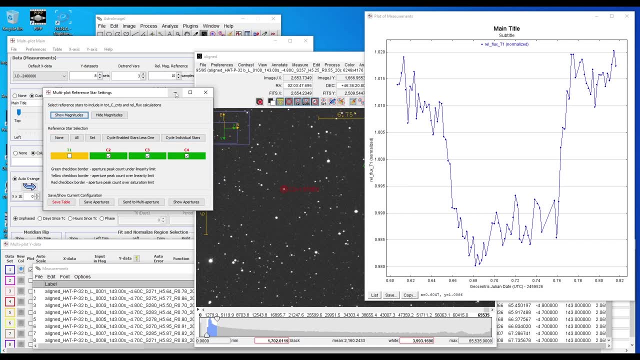 pressing enter. now the data looks much better. we've lost that downward spike at the end and we should have much cleaner data to work with now that we've removed that anomaly. now let's learn about another part of the interface that was put up on the screen. 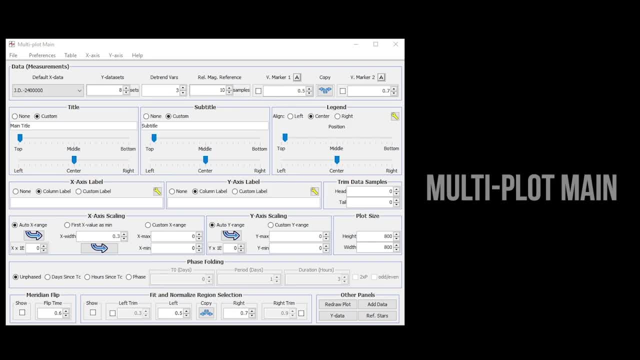 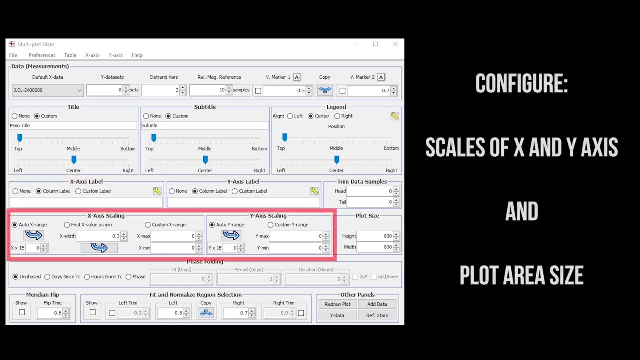 and that is our multi-plot main. now, this particular window is how we are going to configure the graphing interface itself. so we have options to set our x-axis values, titles, subtitles, legend, locations and various other labels. we can also scale the x and y-axis and even change the plot. 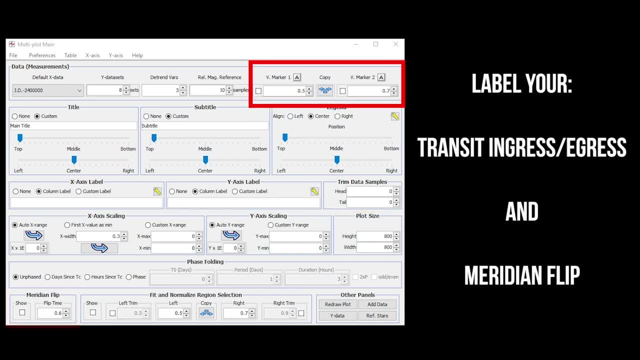 size of the graphic interface and we can also scale the x and y-axis and even change the plot size of the graphic interface, just broaden theiguity of the display itself. we can also identify the expected transit ingress itself. we can also identify the expected transit ingress and egress, as well as our meridian flip on. 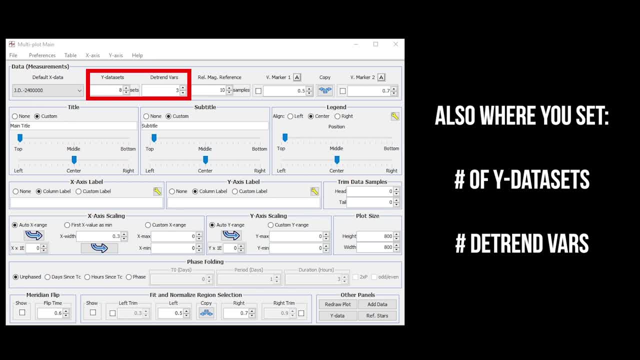 the graphic and egress, as well as our meridian flip on the graphic. previously i showed you on the other window how we had eight lines to use for other window, how we had eight lines to use for plotting data simultaneously in our graphic. if you want to plot more or less, this is the value you would change. 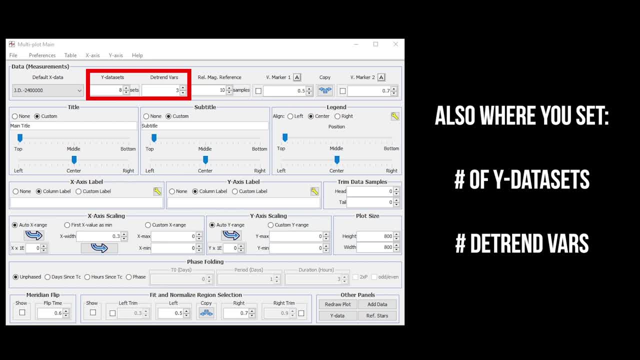 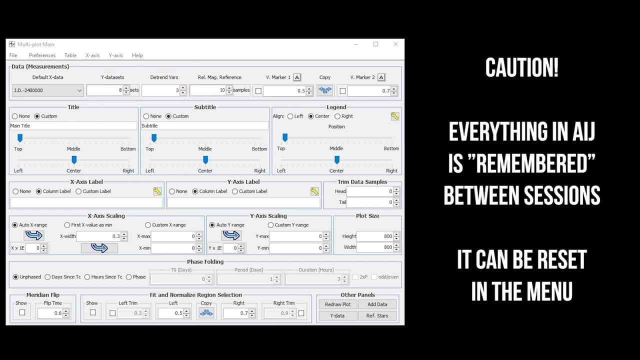 in the main window in order to get more or less lines. you can also change the number of detrending variables, but we're not going to do that in this video. now, there is another thing here i have to point out is that everything is then given the number of department view. 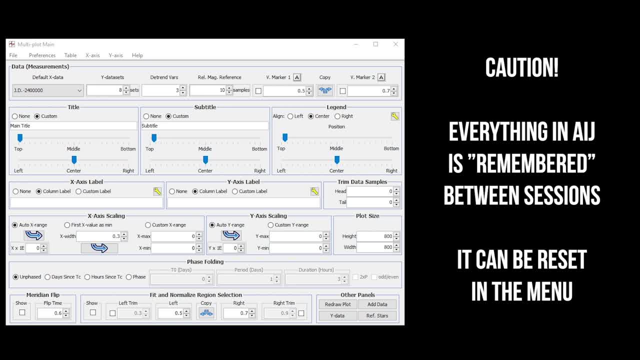 Everything in AIJ is remembered between sessions. so if you get really lost or maybe you've already used AIJ and your settings and interface look very different than mine, you can actually go up here in the file window and tell it to reset your preferences and it'll force you to restart AIJ entirely as an application. 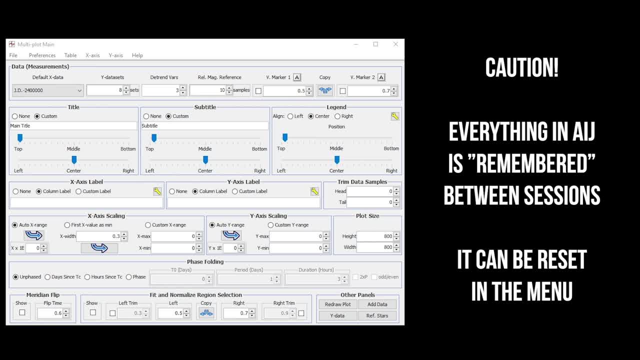 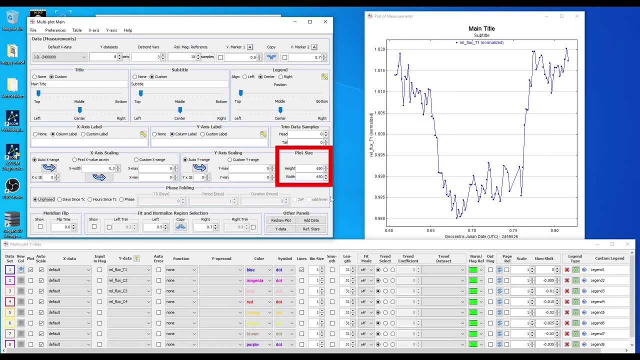 But there may be times, especially when you're unfamiliar with the tool itself initially, that you get lost to the point where you can't figure your way back out of the hole you've dug for yourself. Okay, so let's change our plot area size. Let's make it a little bit smaller so it fits on the screen with everything else we have in front of us. 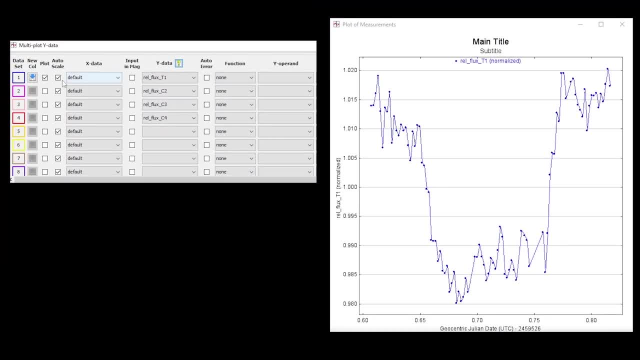 Now, from a post-production perspective, I'm going to zoom and crop certain screens here so that we can really focus on only the parts we're working on, Because if I have to keep you at a full screen resolution, you're not going to know what I'm doing. 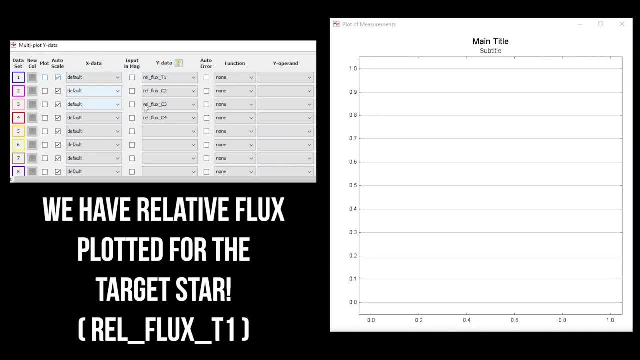 So notice, at the top line we have relative flux plotted for the target star. What I'm actually going to do is disable that and we're going to plot some other things here, just so you can see the power of AIJ and all of the other data it could plot. that could help you understand what you're looking at. 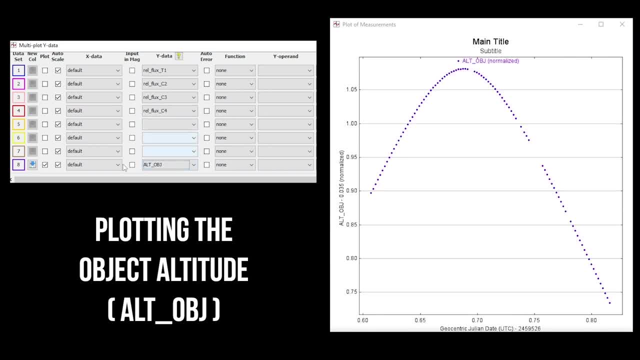 Let's go plot the altitude of the object. Now you can see I've plotted the altitude of the object. It pulled that data out of its calculations from the FITS headers when it went through processing and we can see it looks like a typical altitude chart. 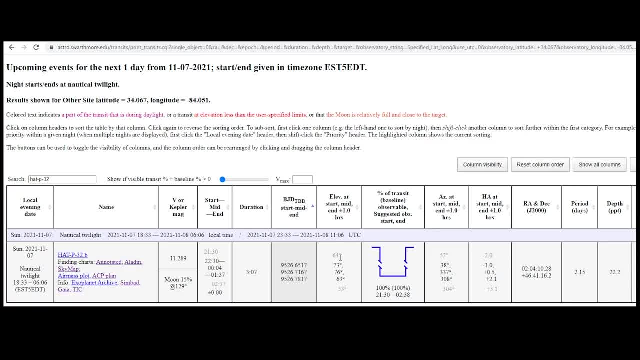 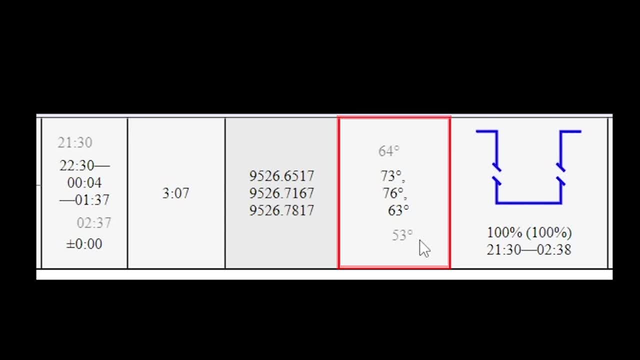 Now we can see it's a little bit smaller. Now we can validate this by going back and looking at our transit data that I showed you earlier. and if we go back and look at this, we can see here we started at 64°, peaked at 76° and then ended up down at 53°, and this does mirror what we expected. 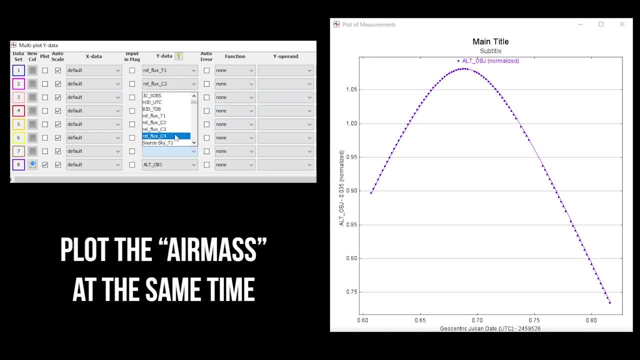 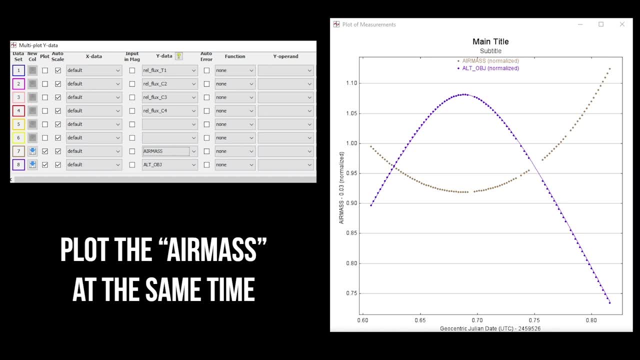 We can also choose to plot the air mass. If you're not familiar with the term, air mass is the amount of air you're imaging through. So if I shoot low along the horizon, I'm going through a lot of air until I get out of the atmosphere, which is going to affect my imaging. 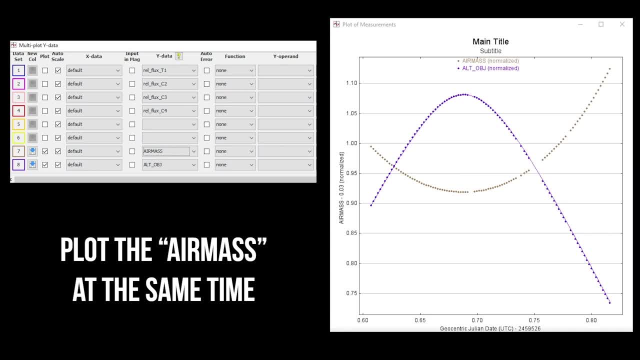 If I point 90° directly overhead at zenith, I'm going to go through a lot less atmosphere to get to my target. When I plot these simultaneously you can see they are inversely related. The higher my object is in altitude, the lower the air mass is that I'm shooting through. 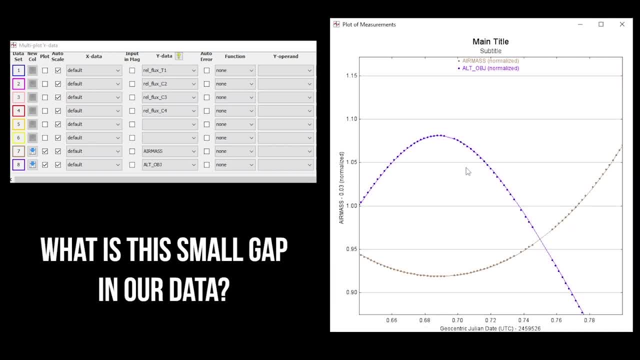 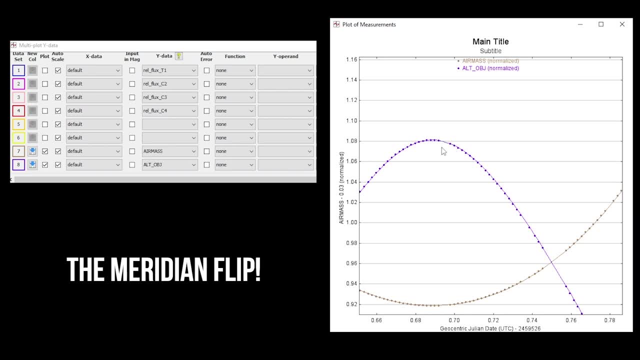 Now, if I zoom in here, we'll notice we have a gap in our data set. What is that small gap near our peak altitude? That's our meridian flip right. We lost some data points when the flip occurred because there was a gap in time where we had to process the flip. 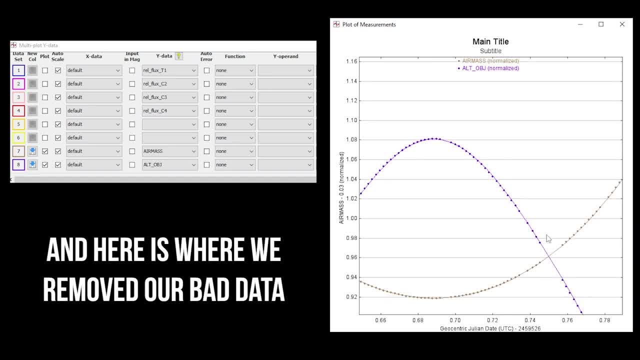 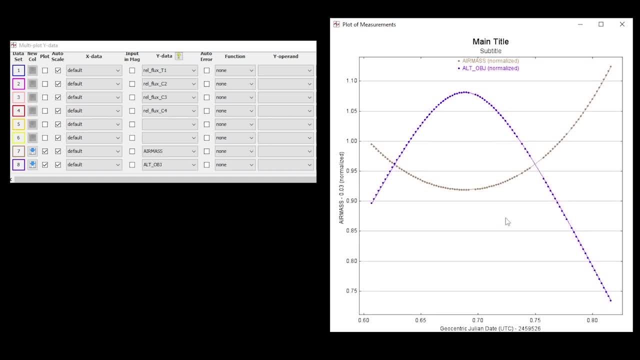 and we were not imaging Over here to the right, this gap is our bad data that we recently cut out. So let's get the timing of the meridian flip so we can plot it. If you remember, earlier when we did alignment, we said that our particular meridian flip happened between slices 43° and 44°. 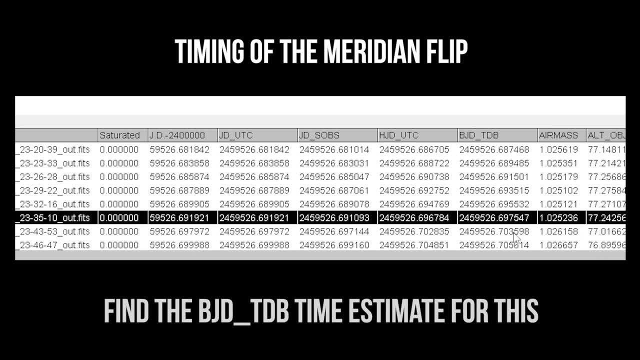 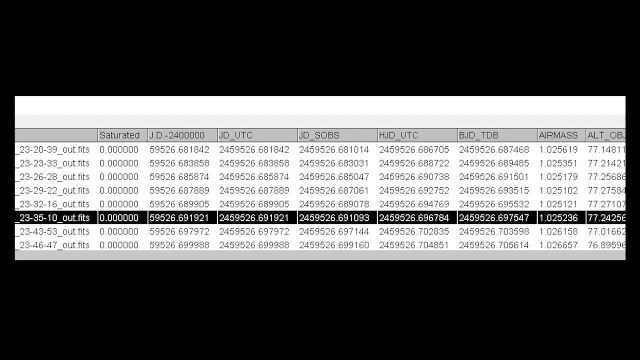 That's when we had the jump in our image. So if I go back to our measurements table and find slices 43° and 44°, I can look at the BJD TDB time and determine when our flip occurred. What I'm going to do is grab the decimal clock. 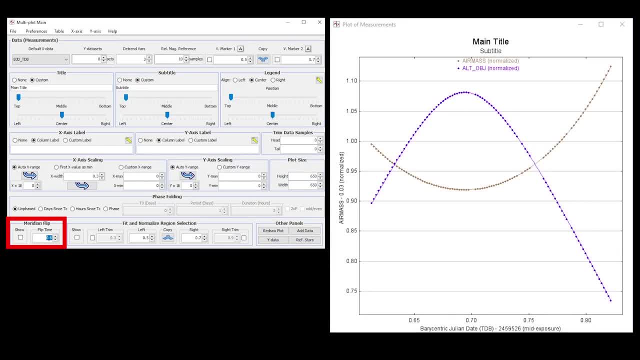 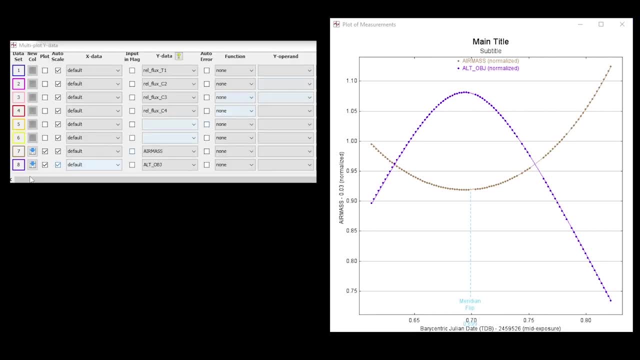 I'm going to take a little portion of that and enter it here in our main window and then click to enable plotting of that And now see that our meridian line is plotted on our graphic. So let's go back and let's turn off air mass and altitude. 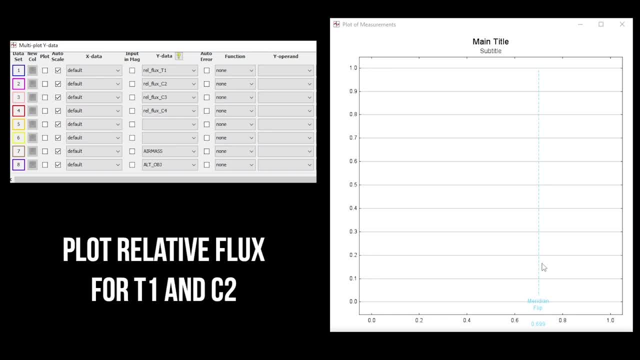 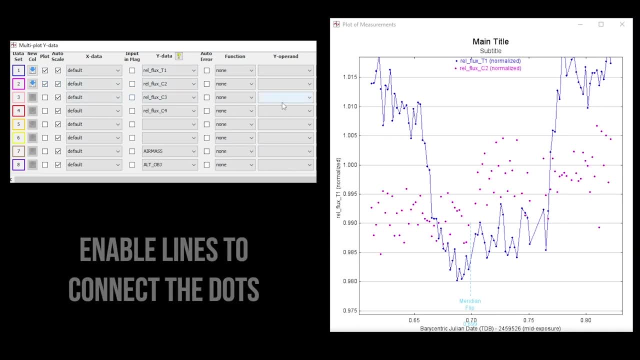 And let's go ahead and turn back on the plotting of relative flux for a target, T1 and our first comparison star, C2.. Now, when I enable plotting of my first comparison star, C2, I may want to make some modifications. Let's turn on the connecting of dots with lines. 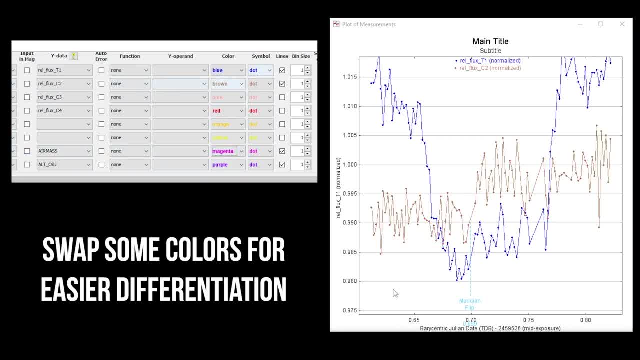 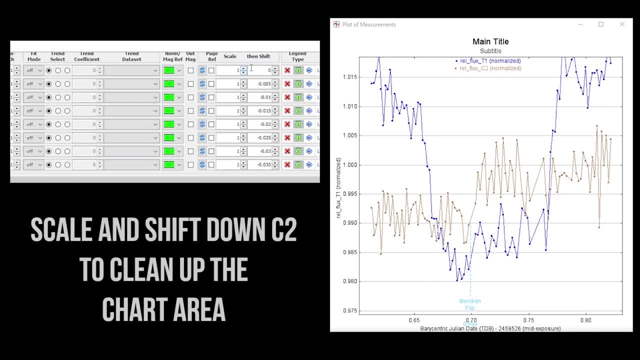 Let's also change the color to differentiate it a little bit more from our target star. We'll also go over and to get these lines from being plotted on top of each other, I'm going to change the scale and the shift. I can change the shift to drop it down a little bit lower in the graphic. 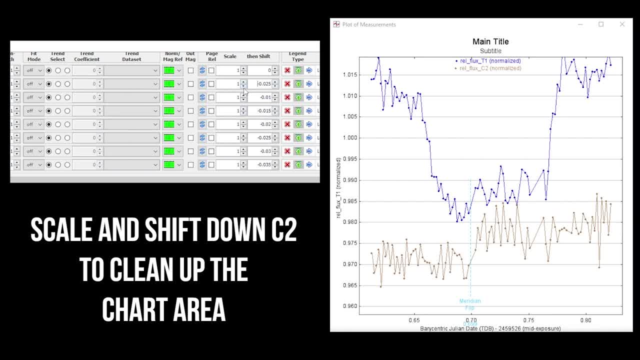 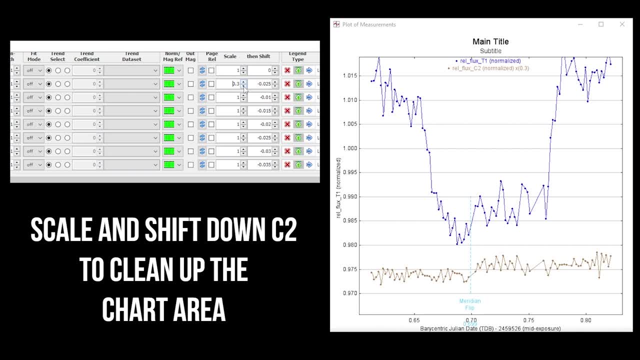 so it's not sitting on top of my T1 data set. I'm going to shrink the scale, which will smooth out the line in itself, and we can see that it doesn't dip, that it's actually maybe going up a little bit to the right. 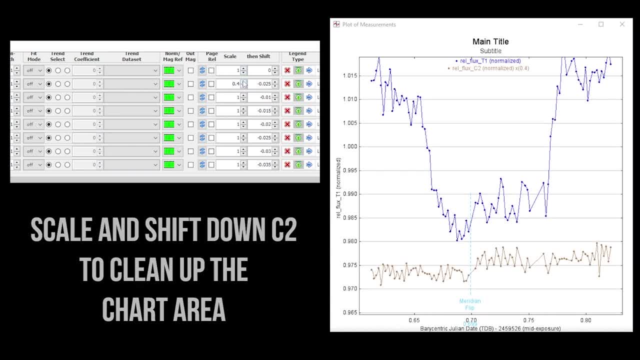 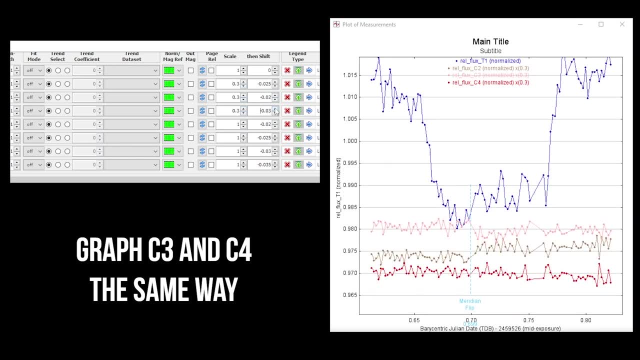 but it's more or less flat. Once I'm happy with the outcome, I can go ahead and graph C3 and C4 the same ways And again I'll adjust those and I'll move them down using the shift and scale capability. 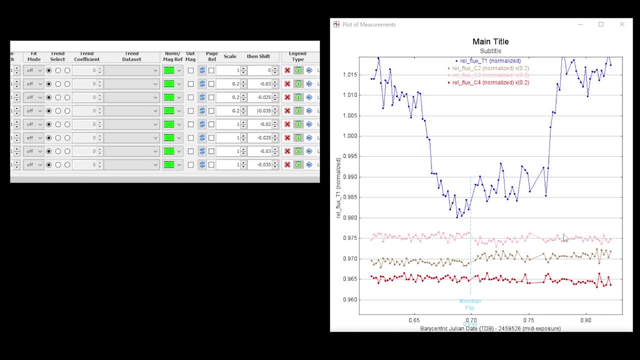 So now I've got my target star at the top, and then I've got C2, C3, and C4, and we can see the data looks good. C2, C3, and C4 are all pretty flat and level. 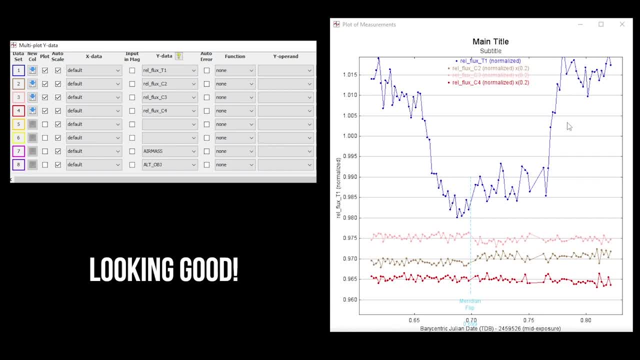 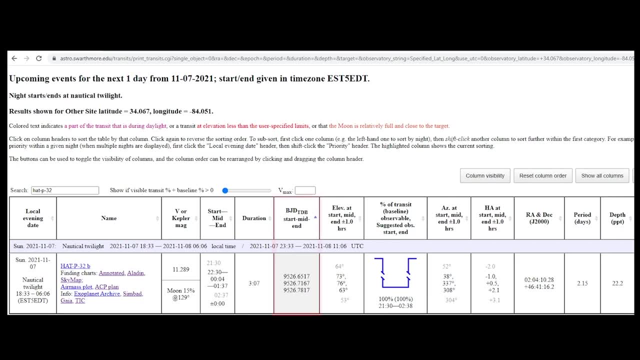 They didn't have light dips, but our target star did have a light dip. Now the question is: did it dip when it was supposed to dip, based on the transit? So let's go back and get some more data about our transit. 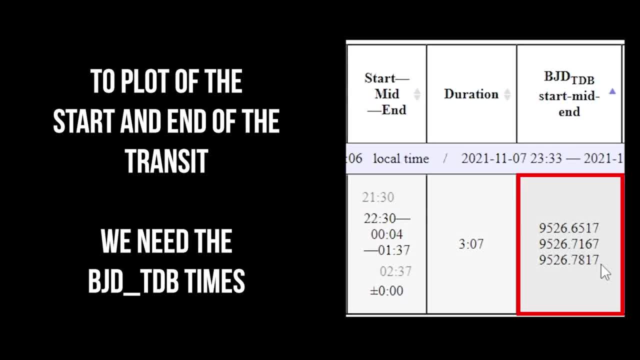 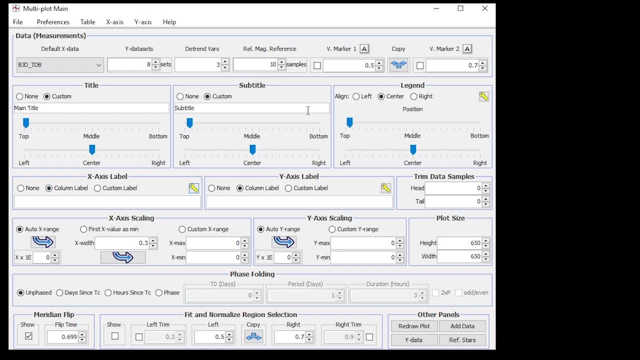 The data we care about right now is the BJD TDB time for our transit and specifically, we care about when it started and when it ended and we care about those TDB decimal portions. We're going to go back to our main window. 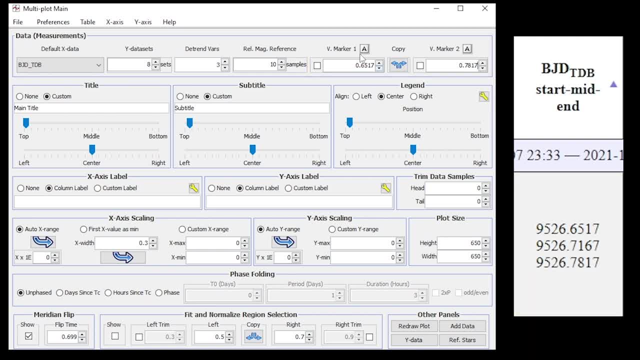 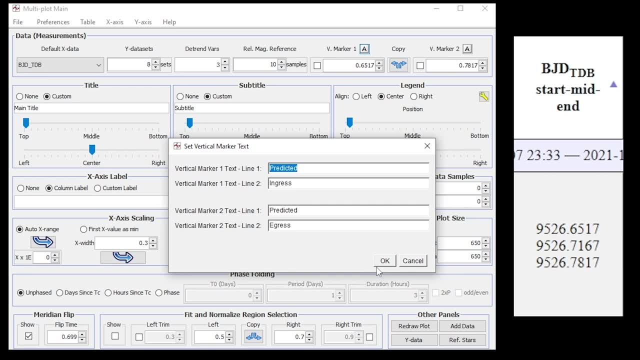 and we're going to put it in the section for the ingress and egress data. You can see there's a little button here that lets you see how this will be labeled and it's automatically set up to label this as predicted ingress and predicted egress. 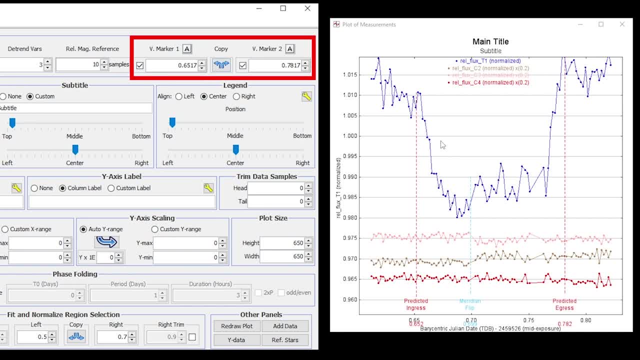 Now that I've got these data points entered, I can click the checkboxes to plot them and you can see they're actually falling right about where I would expect them to fall for our transit. This is a good sign. Now, one thing I don't want you to forget that most people do forget. 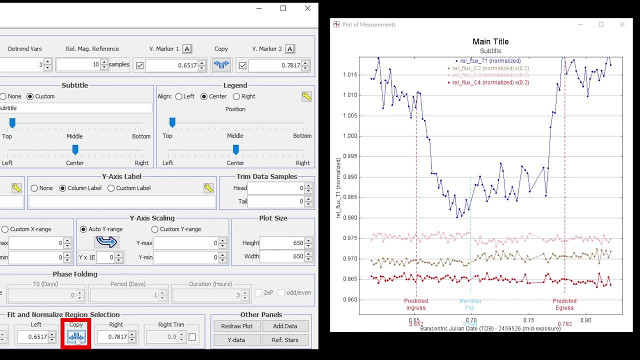 before they go plot. a predicted fitting curve is that you need to go to the bottom of the main window and click this copy icon and it's going to copy your ingress and egress data points down here to the fit region. So now we want to come back to the T1 line. 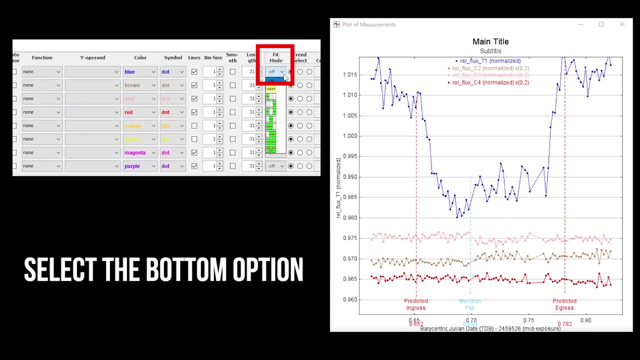 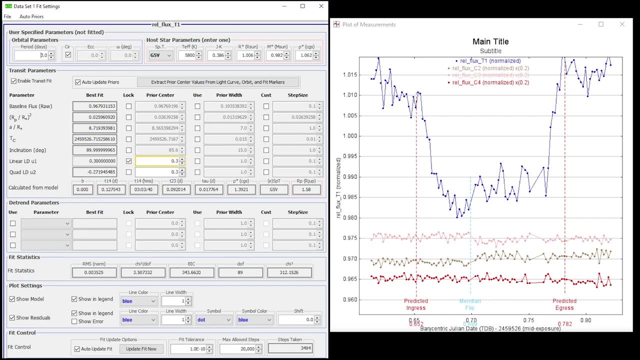 and scroll over to the right and look at the fit mode. Now you're going to go all the way to the bottom of the fit mode options and select the one that looks like a flux light level curve and we're going to get this pop-up window because we didn't have enough windows yet. 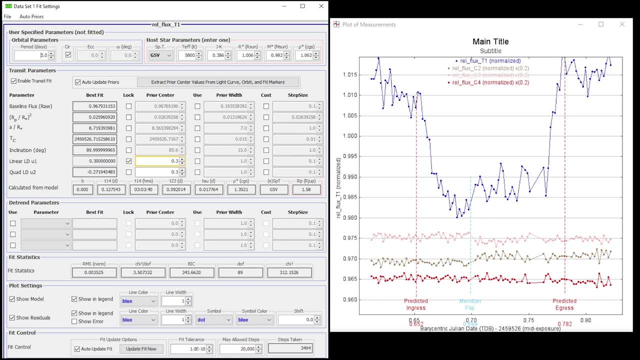 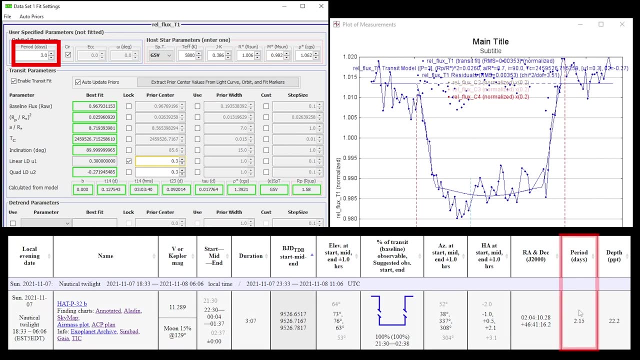 Now, in the upper left-hand corner of this window, there is a place to put the period and days of this particular planet, and we need to go back and get this data from our earlier table. If I go back there, I can see that this particular planet had a period of 2.15 days. 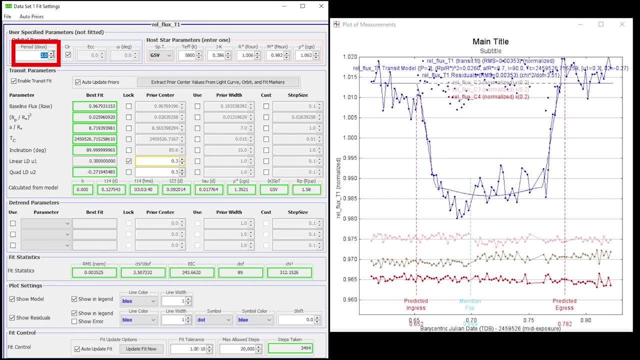 so I'll enter that here, and once that's done we can actually also lock in U1 and U2 with these check boxes and you can see we're getting a light line. that is a fit model that looks pretty good to our curve. 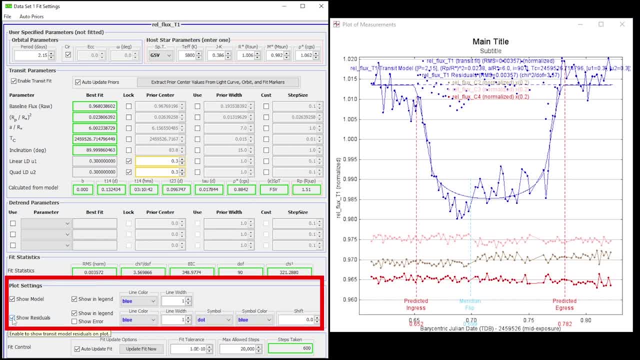 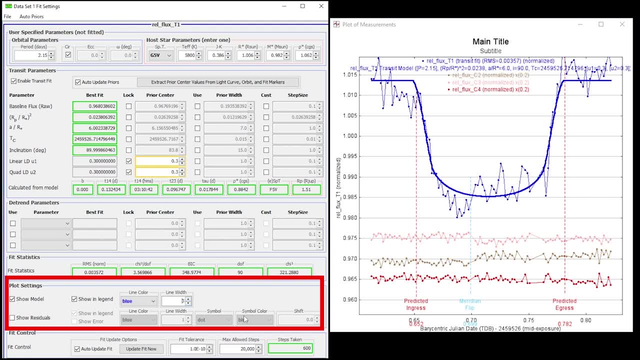 Now to clean this up a little bit more. we're going to go get rid of our residuals from being plotted. We're also going to increase the thickness of that curve that's being graphed to 3 to make it nice and bright. 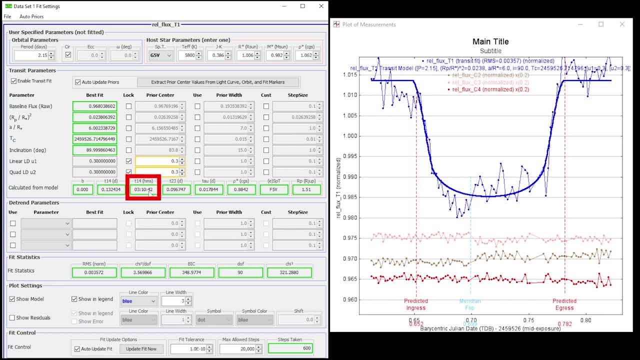 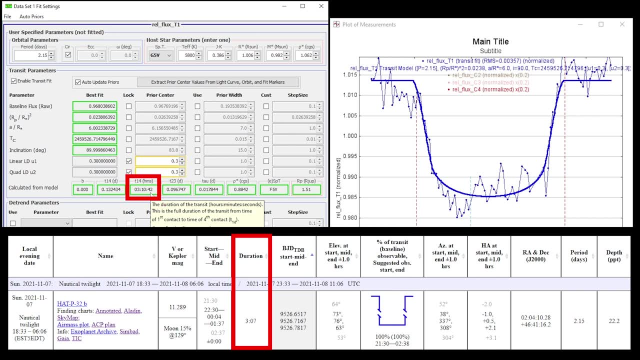 One thing we can validate now, based on the curve that was fit is: did our transit duration match? and if you come over here we can see that we have hours, minutes and seconds of the actual transit that we've plotted based on our data. 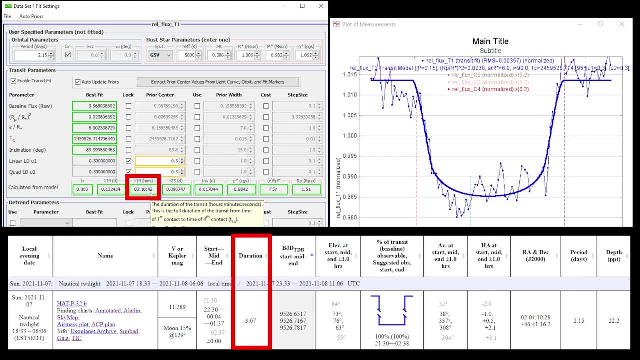 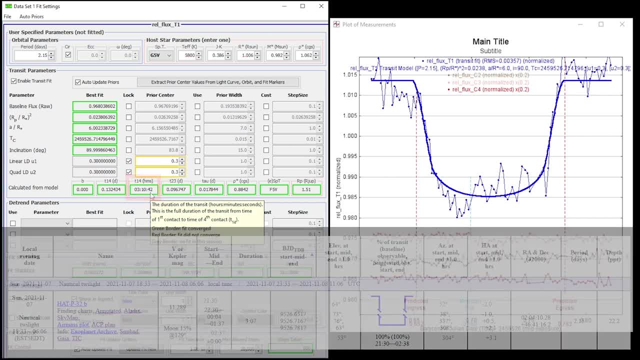 and if we go back and look at our earlier reference, we can see that we found it was 3 hours and 10 minutes and it was predicted to be 3 hours and 7 minutes and I'd say that's pretty good. 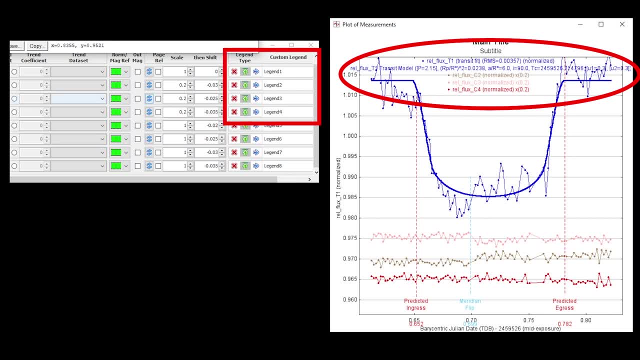 One thing you may want to do is clean this up, even a little bit more. We can go clean up the legend here. I'm going to turn off the names of all our comparison data in the legend just to get that off the screen. I'll click the Xs for that. 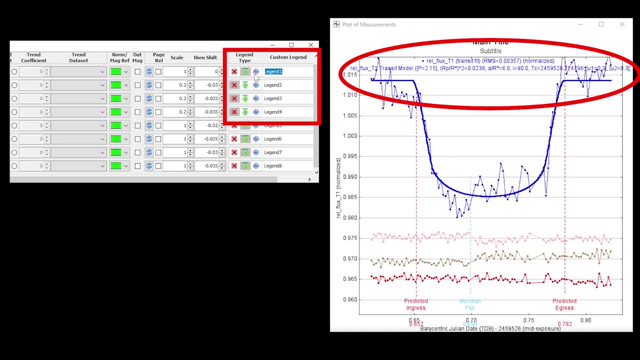 I also want to relabel the plot data that we have for our curve to just be the name of the planetary object hat P32B. so I'll go ahead and label it, turn it off and then use the right arrow to force that onto the legend. 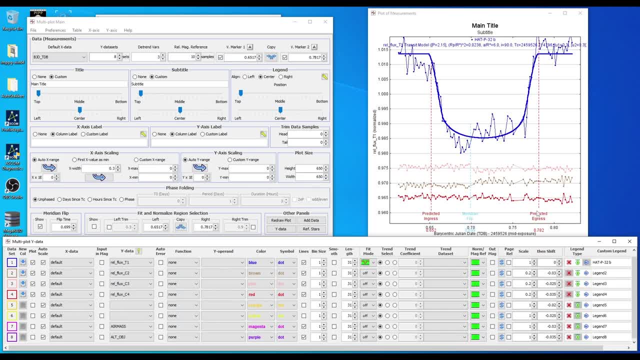 Now I'm going to come back to the full screen here So you can start to see how all the pieces come together as I make a couple more minor changes. Now there is one other line in the legend I want to remove, but it's actually a result of the fit mode. 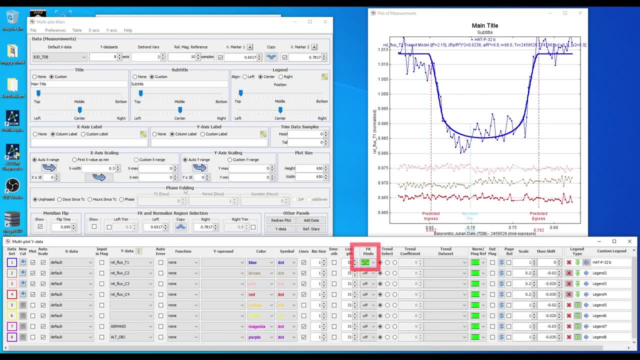 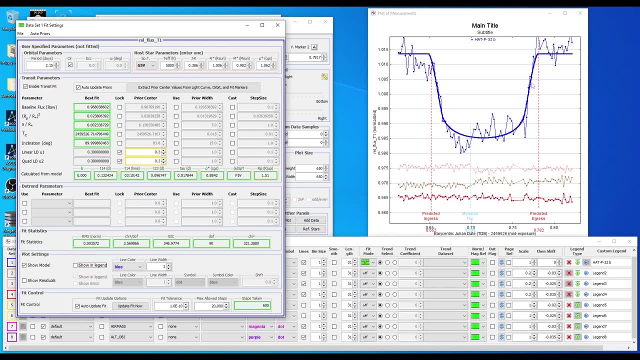 So what we actually need to do is come back here, select the fit mode, curve again and then, within that pop-up window, go Turn Off Show in Legend. Now, it's certainly not a requirement, but I think it cleans the screen up a little bit better. 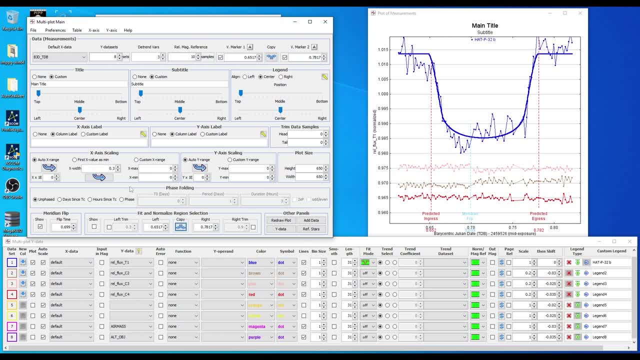 So now we've got a simplified legend and maybe we can just clean it up a little bit more, So let's go ahead and do that from a graphical standpoint. So just to clean this up a little bit more, it seems like my data might be clipped on the top end of my graphic. 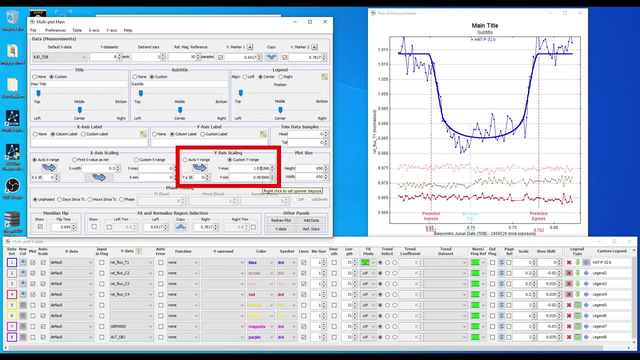 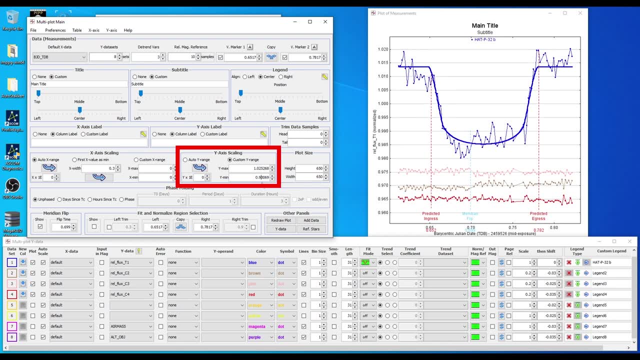 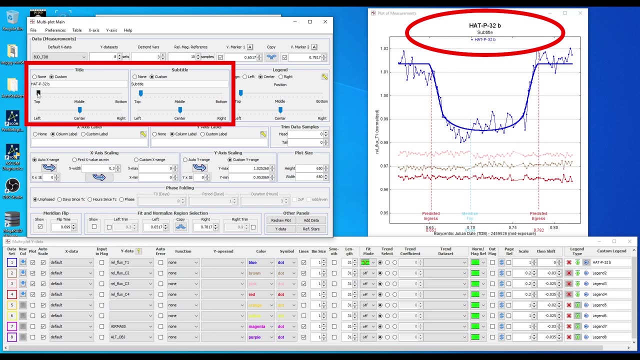 so I'm going to change it from being auto-scaled in the Y range and I'm going to go ahead and manually modify my Y axis so my data fits a little bit cleaner. I'm also going to change the title and subtitle and notice: you can move these objects around. 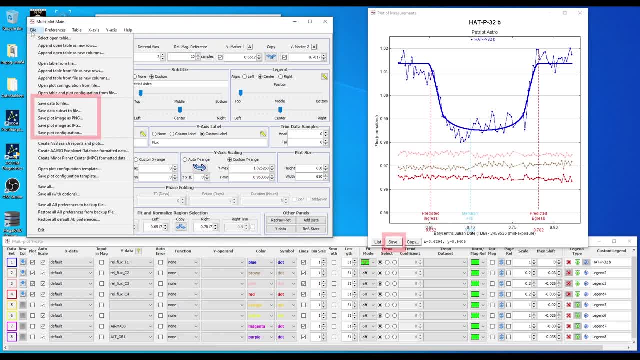 There's several other things you can change here. Now, as far as exporting an image from the graphic itself, on the right you can click Save to save an image of that graph on the screen. You can also in the main window. 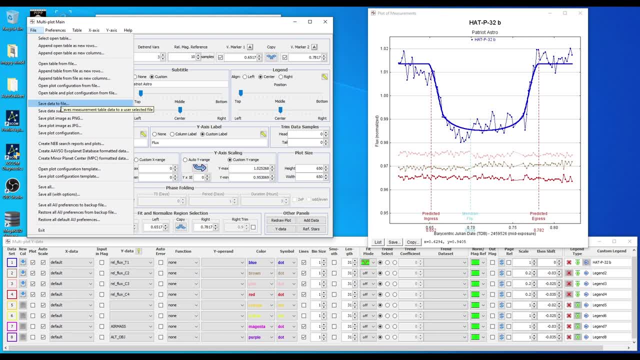 click File and choose to save as PNG or a number of other formats. Notice also that we have several other options available to us to export data. If you plan on sharing your data and your findings with the scientific community, you actually need to export a lot of this data appropriately. 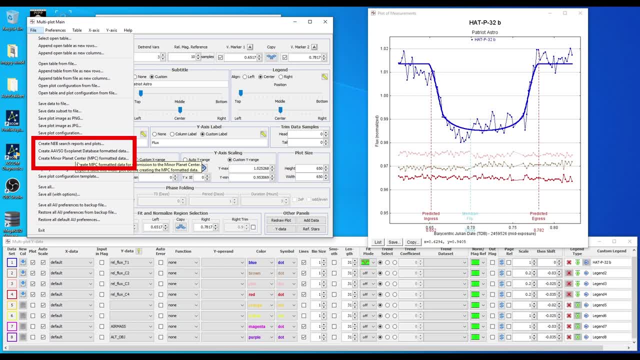 so that you can submit it into those databases. I'm not going to do that here in this video. And then finally, in the bottom left-hand corner, if you ever do get lost, know that you can click to restore all default AIJ preferences. 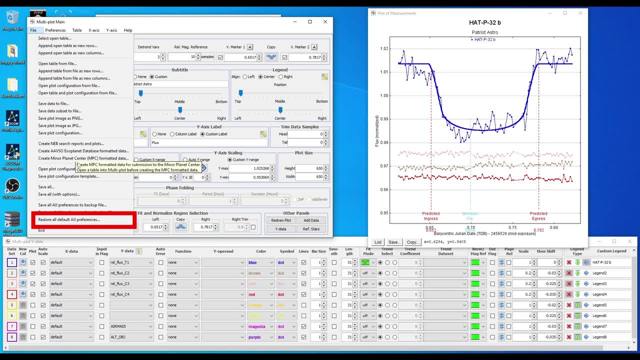 That'll get you back to all of the default parameters and interface settings, as when you installed it initially. All right, so, as you can see, there's a lot of capability in AIJ. There's the ability to plot a lot of extraneous data.